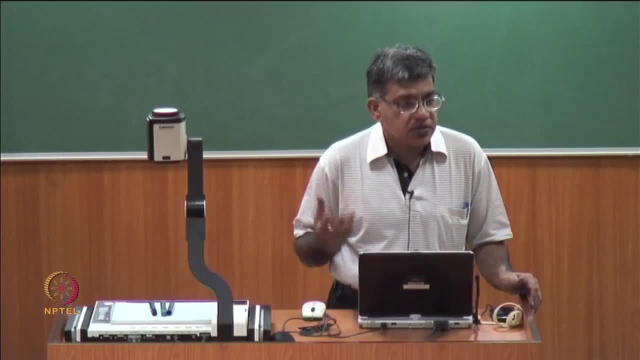 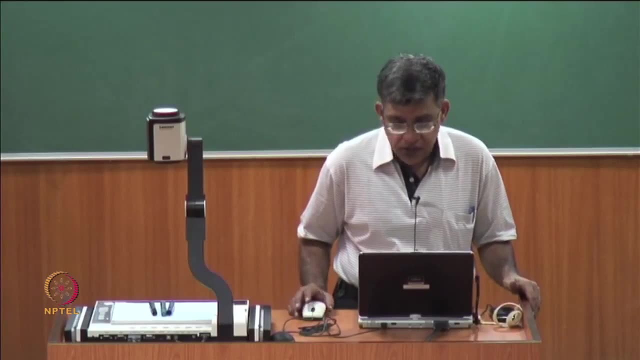 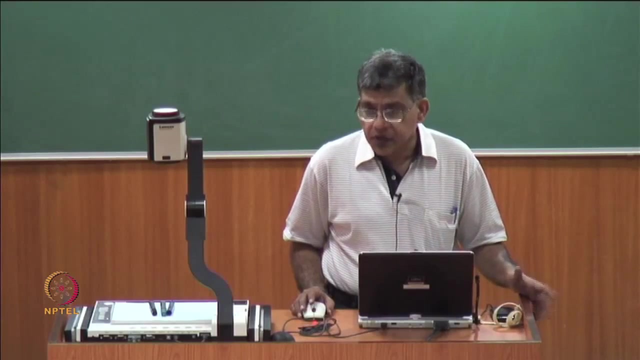 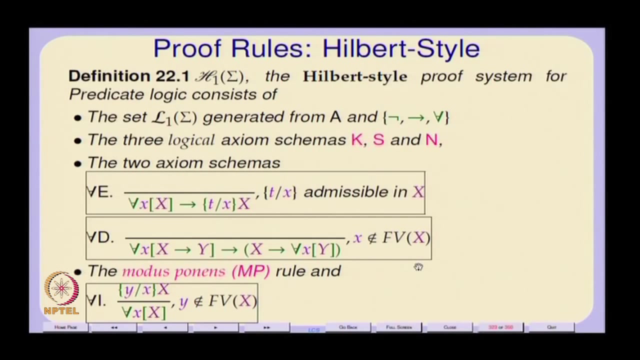 axioms through the non logical axioms. So, whereas this one just looks at logical validity itself for all possible kinds of different signatures, And so we will actually look at first order predicate calculus before we go on to any other first order theory And then. so there is a small change here, this for: 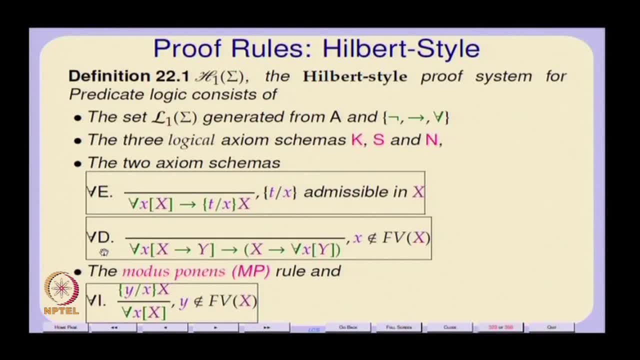 all d. So they used to be a quantifier for all x a. So I actually said that for all x distributes over this arrow. But now I am actually putting some restriction. this is because of some proofs. there is some problem with some proof, So it had to be in this form. So if x does, 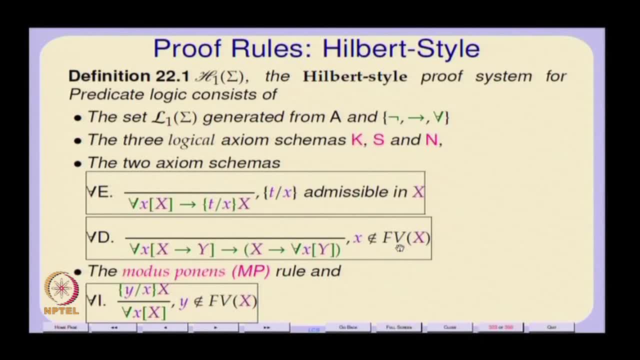 not have small x occurring as a free variable, then what it means is that, rather than distribute a quantifier for all x, you can push it in, so that Then this capital X big becomes quantifier free, And so that it adds a certain extra power for the purpose. 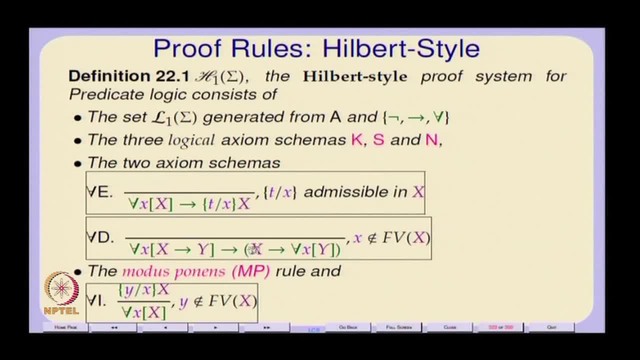 of certain groove rules and its validity is not in question, because if x is any way not a free variable of x, So that even if you quantify it as a free variable of x- couch, That is what you are interested- it does not matter. But this form has some advantages. the other thing is this: I have 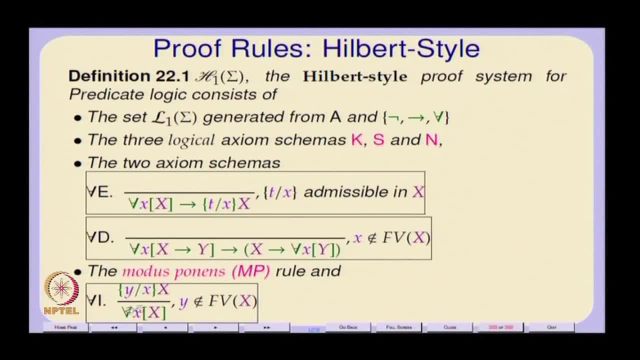 also made this. I think- I do not know, I think it was not in this form when I spoke last time- But this universal introduction, universal quantifier introduction or what is known as universal generalization, So I am writing it in this form. essentially, what I am saying is: if you ever how? I think I had it in this. 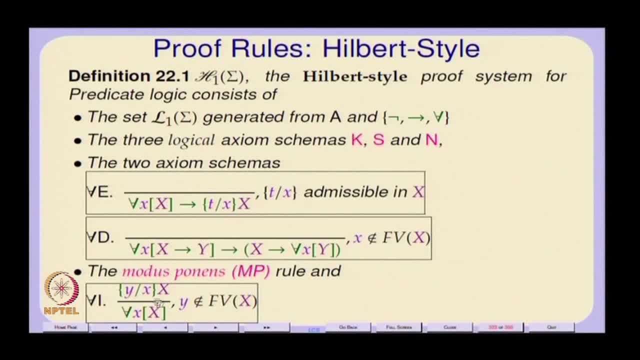 form last time also, So there is no problem. So essentially, this means that, if you can, if this y is a completely arbitrary variable, then you can quantify it over x. The notion of arbitrary needs to be captured somehow, symbolically, and that is. that can be a problem, But we went through all this is all fine. 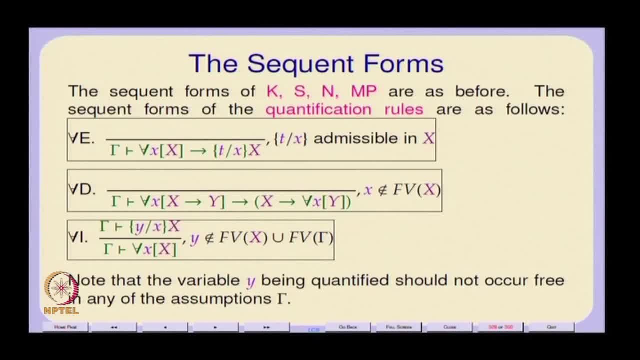 Of course, we have to look at the sequent forms of these rules, because- and this, the sequent forms, are essentially of this kind, Now that in this, in the sequent form, what we are saying is we assume that there is some set. 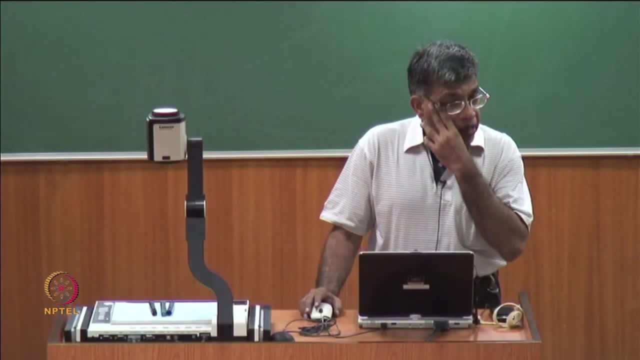 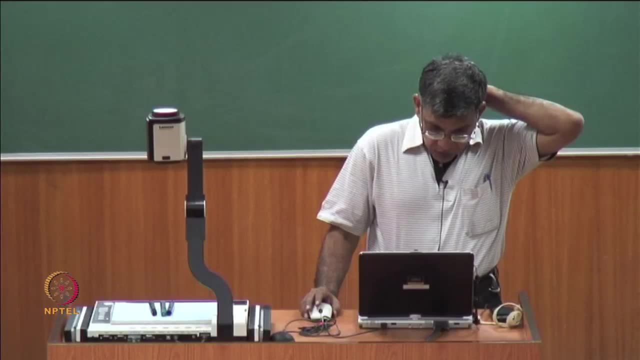 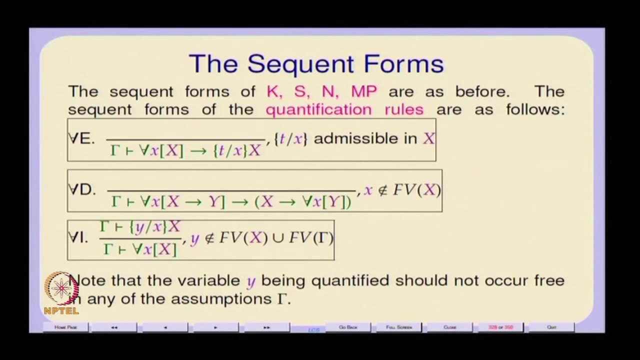 of assumptions, gamma. for any first order theory it will be the axioms. the non logical axioms might form gamma. So we have to look at. So this gamma is therefore important while we are dealing with predicate calculus. it does not matter whether we look at, use it in the sequent form or in the non sequent form, But the moment. 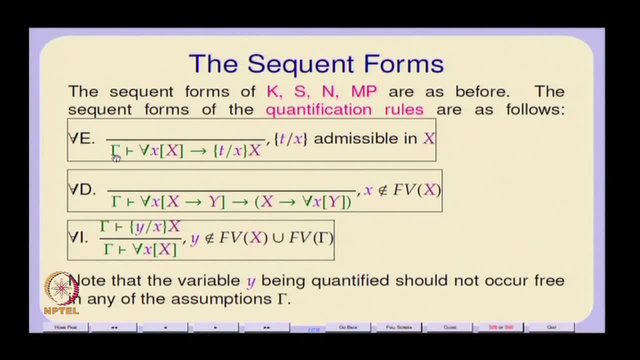 we talk about a first order theory. we are talking about a set of non logical axioms which will be there in gamma. So now, if you have a collection of 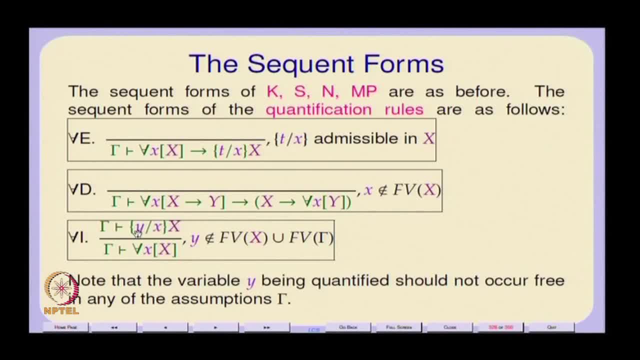 arbitrary y- I mean the meaning of the word arbitrary- has to be captured somehow. If that y may not be arbitrary, then you cannot necessarily. 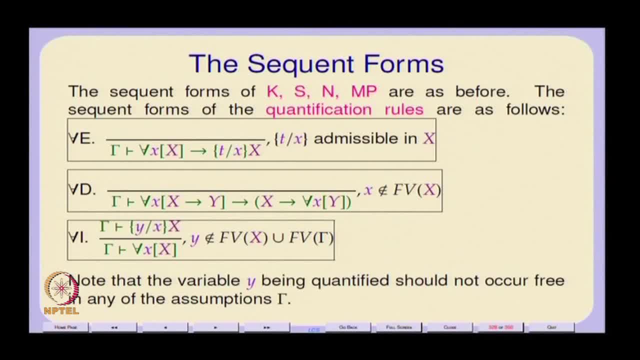 generalize on it. If, however, y occurs free only in this expression, capital capital x, with y substituting x, and this proof goes through, then it does not depend on any particular value of y And therefore it can then be generalized. So I mean, that is the intuitive reason. in a formalization, one has to worry. 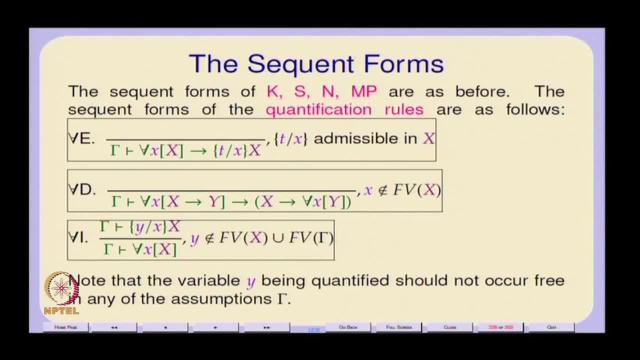 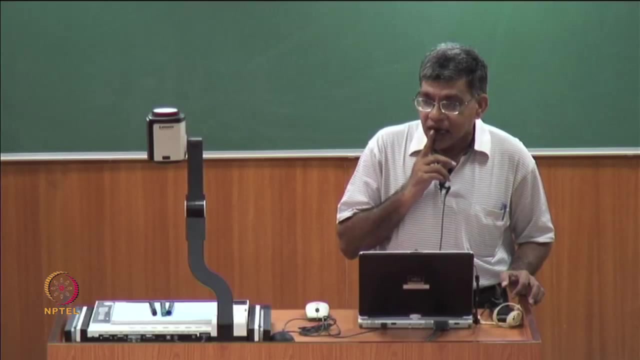 about what are the freely occurring names. So if y is a name occurring in more than one of these assumptions, in one or more of these assumptions, And it also occurs free in this hypothesis, then it means that y is some particular kind of y, I mean like Socrates, for example, s it 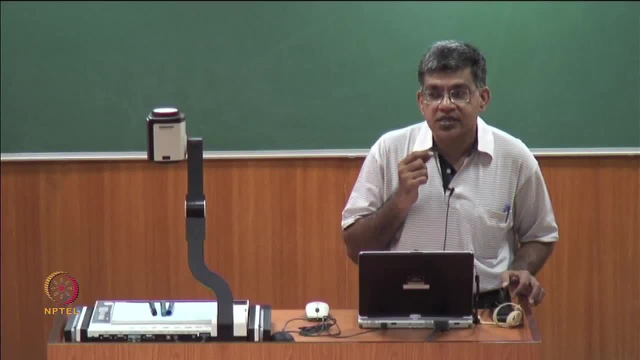 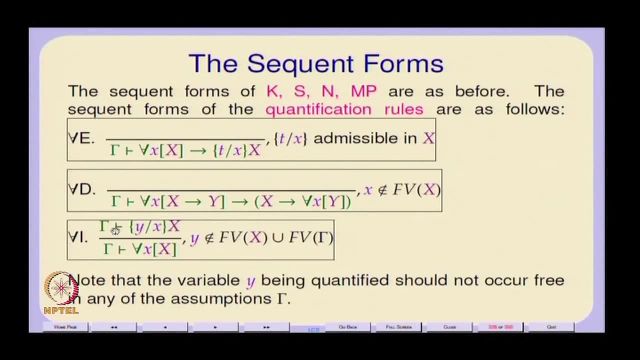 is not, then it is not. you cannot directly generalize then, because it might, because under certain interpretations So this may not. for example, then if you generalize, then you are not, you may not preserve validity, Because that if that y stands for only certain particular values. 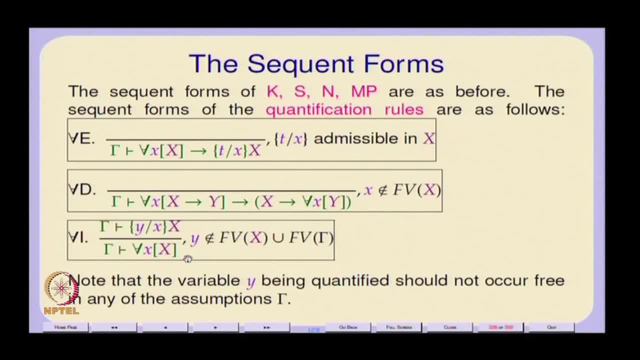 for which this predicate is true, Then it does not generalize to all values, and that is the intuitive reason why we require that this y should not be. I should not occur free anywhere in gamma either. Anyway, if y occurs bound anywhere in gamma, it does not matter, because that those bound y's are different. 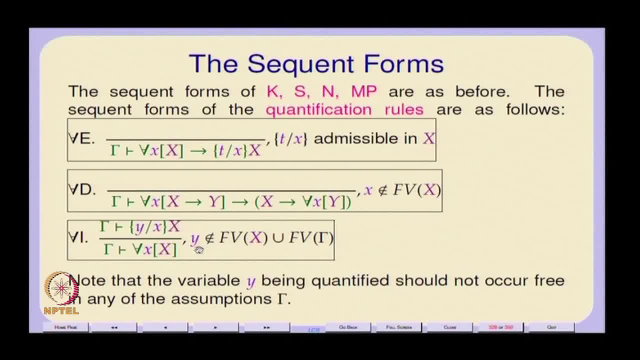 from any free y. So the notion of y being completely arbitrary is only guaranteed if it occurs free in this formula. And if it occurs free in some other formula, also in gamma, that means you are. it is like this: you take. you take the identity element, for example, So predicates. 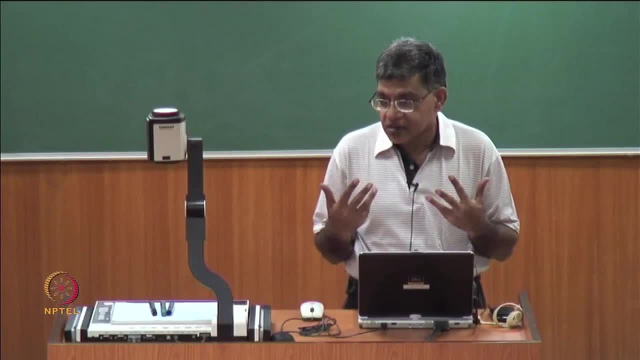 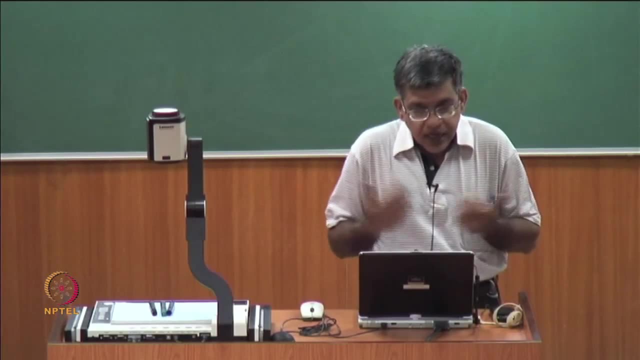 dealing with identity element cannot be universally generalized, Because usually in a in any algebraic structure, there will be a single identity element. all other elements are not identity. the identity might have a variable name or it might be, even if it is not a constant. 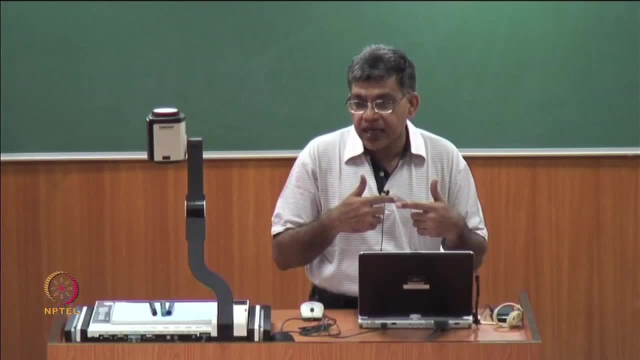 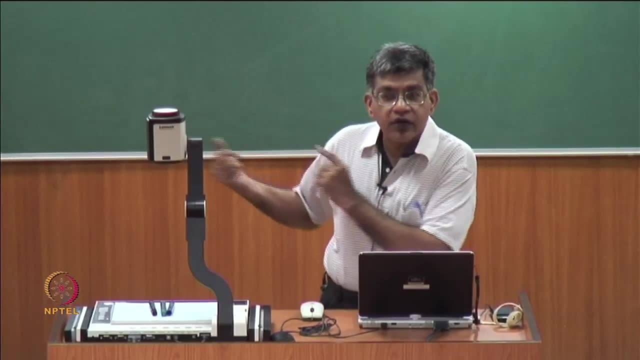 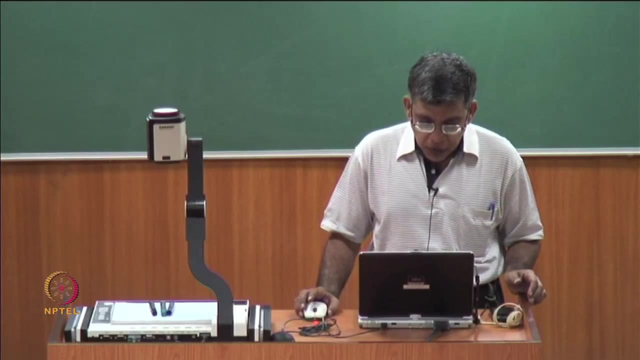 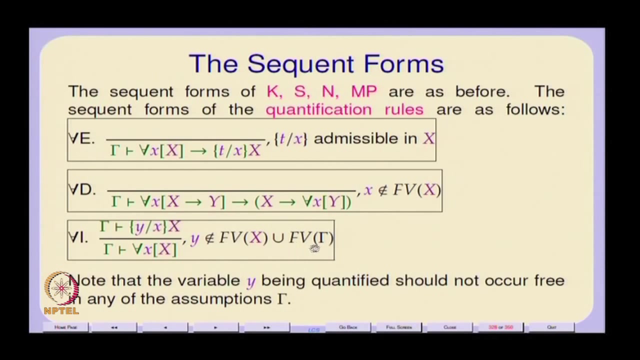 So this, the set of predicates, the assumptions that you might make, might with with some free variable y might imply that that y should stand only for the identity element, In which case you cannot generalize arbitrarily, right? I mean, that is the intuitive reason why you require that this y should not be a free variable anywhere in either in x or in any of the. 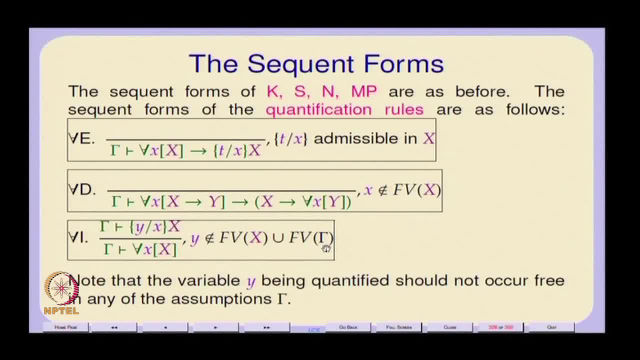 assumptions in gamma. If it does occur, then you are not necessarily preserving validity. if you, if you generalize on y, Whereas if it does not occur free, then this y replacing small x and capital x and occurring free, is essentially an arbitrary y. it is not a particular y And hence can be generalized. I mean, that is the. 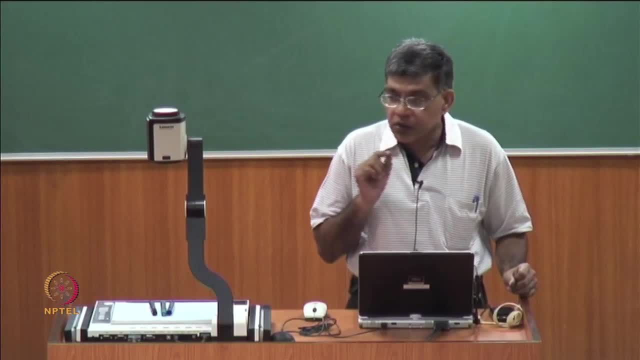 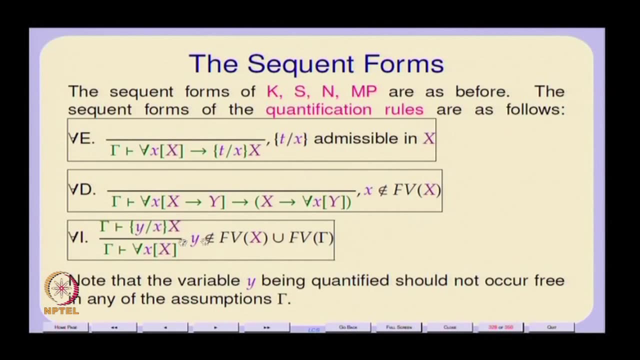 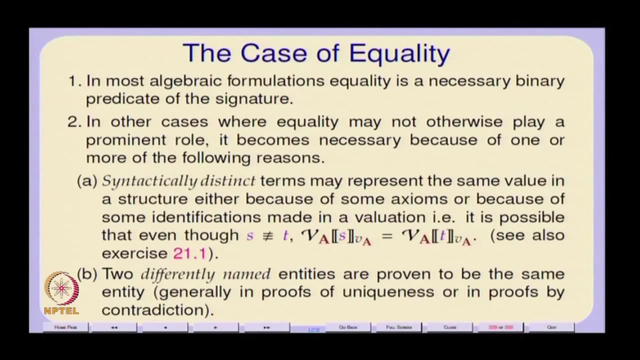 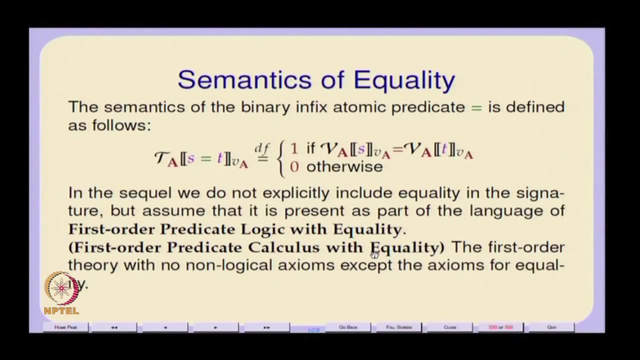 intuitive idea why you need to be careful about the occurrences of free variables, right? So in the sequent form, we will actually use universal generalization in this in this way. 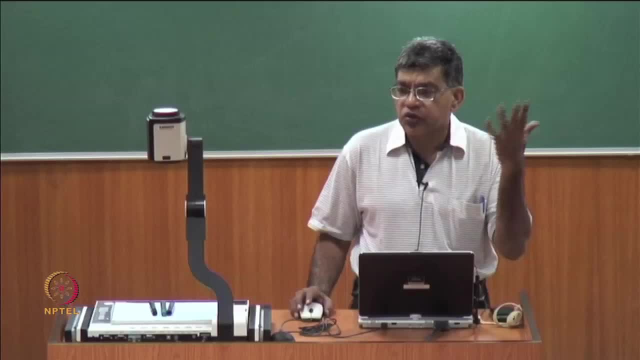 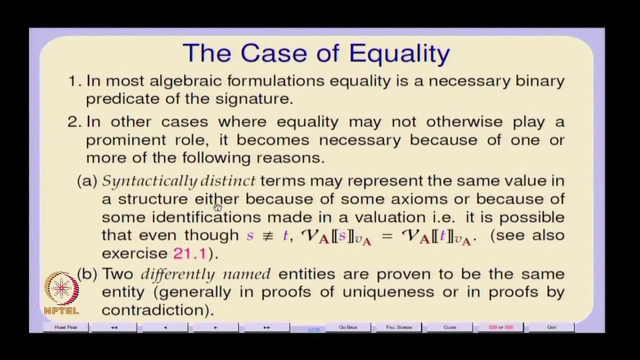 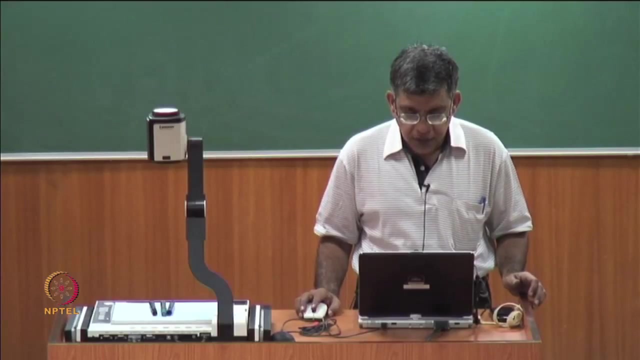 in all algebraic structures. But, however, keeping in mind the fact that syntactically distinct terms under certain interpretations might lead to the same value in the structure, we have to define the semantics of equality essentially, as this: So s and t might be. 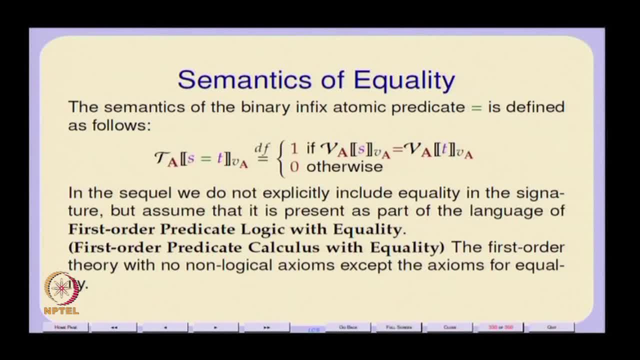 two distinct terms and under any interpretation, a with a valuation v a. this equality is true if the valuation, the value of s and the value of t are the same in the structure a, and otherwise it is false. And since equality is sort of special, we can also talk about first order. 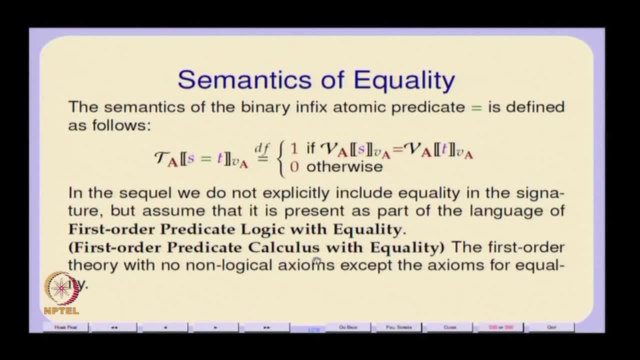 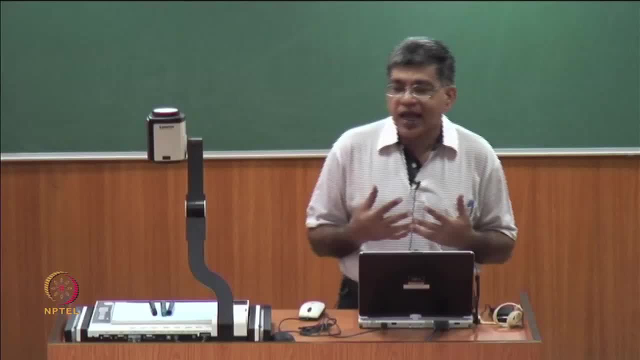 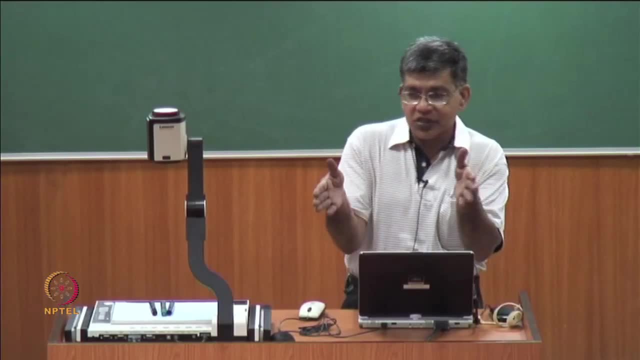 predicate calculus with equality, So, which means that we have to look at the. So I mean. now it is a debatable question whether the equality axioms should be considered non logical or logical. I mean equality lies somewhere in the interface between the logical and the non logical. 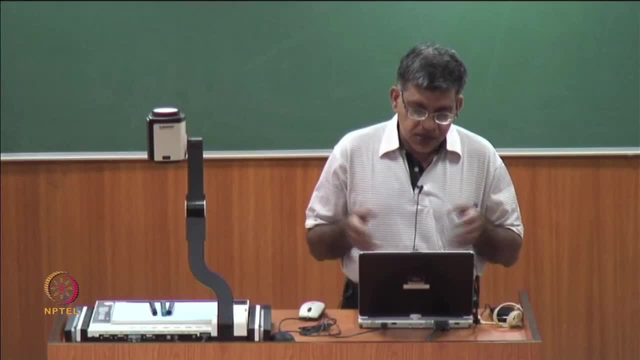 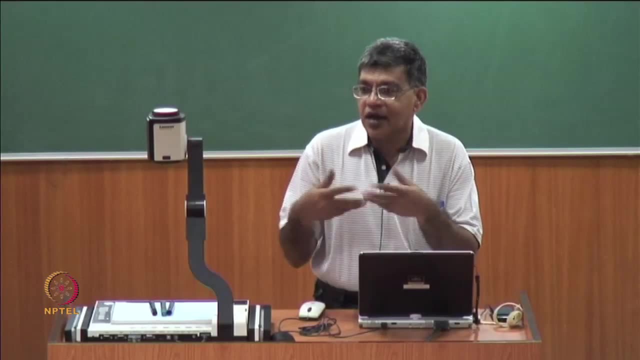 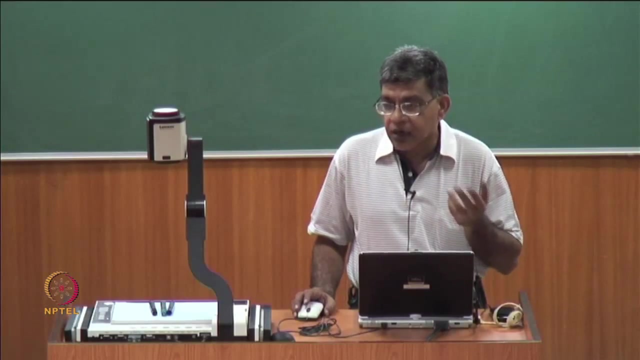 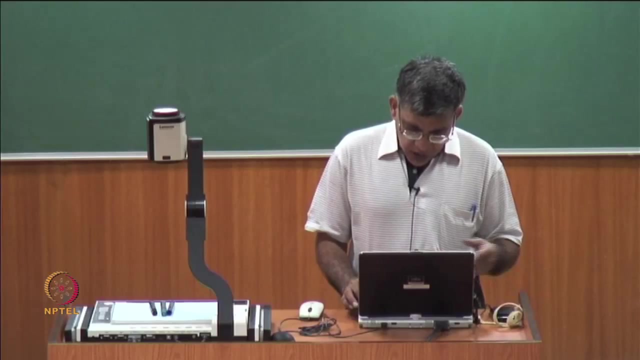 So because of this we might actually. so you have actually a first order predicate calculus with equality, where equality is regarded as one of the logical and special binary relations binary predicates that should be available. let us say So. that may not be true always, so that is called first order predicate calculus with. 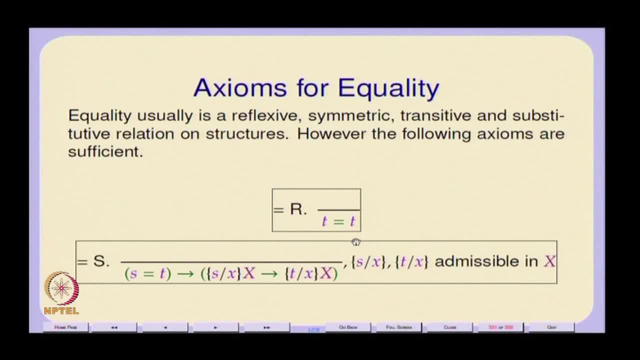 equality. So let us look at the axioms of equality, and I think that is right. So, firstly, of course I have made a correction: instead of x equals x, I decided to make it for all terms t. So this is the reflexivity property. the second thing is that I had this notion. 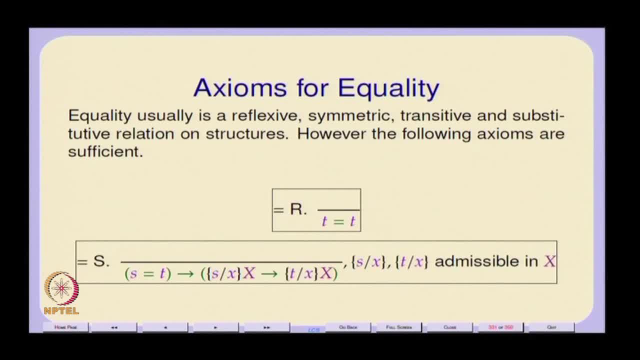 of replacing 0 or more occurrences. now I have made that more uniform through this substitutivity axiom right. So if s for x and t for x are both admissible in x, then s equals t arrow, s for x of x arrow. 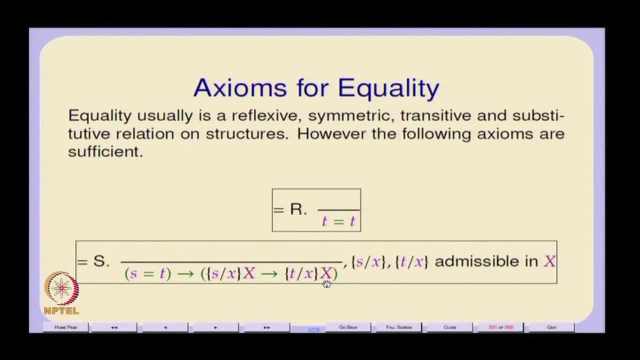 t for x of x. So this is the uniform substitution and all occurrences, all free occurrences of x would be substituted. this has some advantages, right? So substitutivity is this axiom, and it is actually a very powerful axiom. 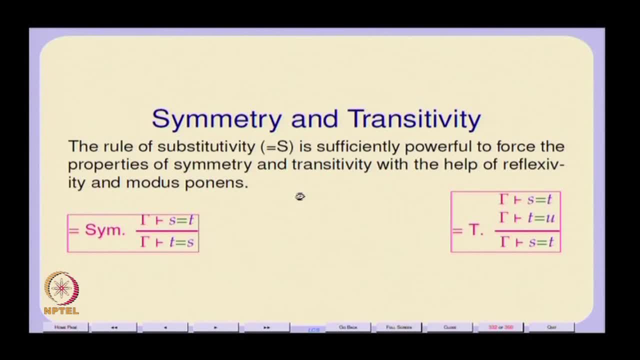 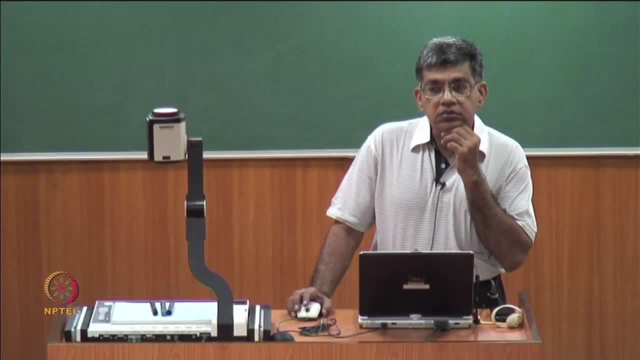 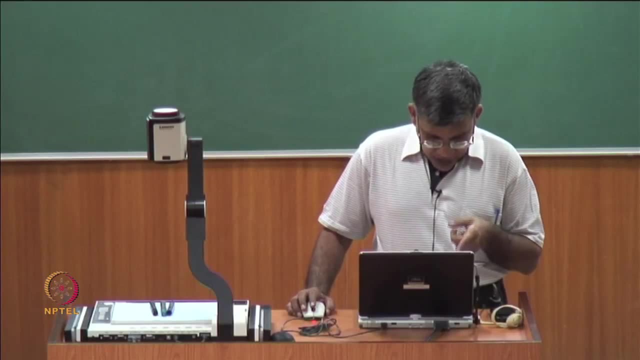 So one thing is that normally any equality relation is also an equivalence relation. So what you expect is that. what you expect is that the properties of symmetry and transitivity should also hold. But this substitutivity axiom, in this form, is so powerful that we can actually use symmetry. 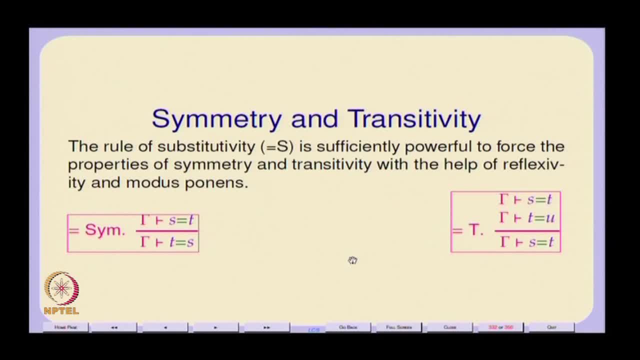 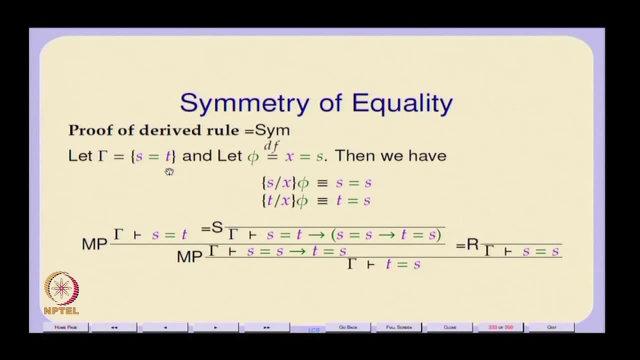 and transitivity as derived rules, basically. So here is a symmetry rule and so, essentially, if I take s equal to t as an assumption, and I take this formula, So this is the formula: x equals s. one thing, of course, is that x might occur free. 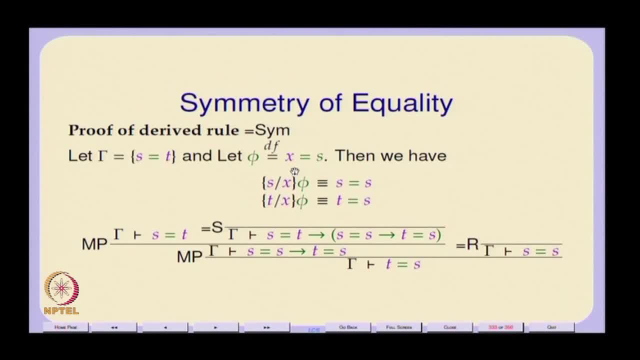 in s, for all we know is it: can x occur free in s? x could occur free in s. I mean, there is this question of whether x is recursively defined, in which case whether you are finding a fixed point and so on, so forth, But purely syntactically speaking, there is no reason why x should not occur free in. 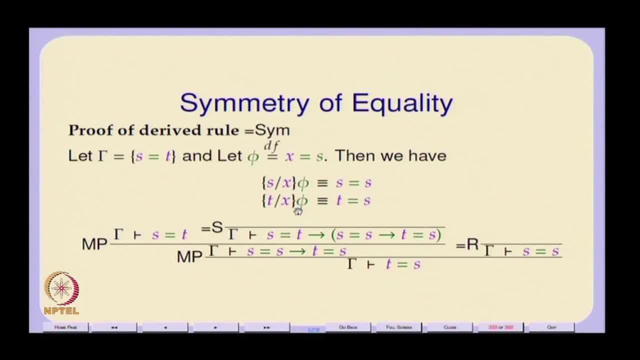 s And it can also be substituted, so, which means that you might actually substitute a free occurrence, a term containing a free occurrence of x, for occurrences of x in this predicate, and that is not unmeaningful. I mean it is not meaningless, I mean in the sense: 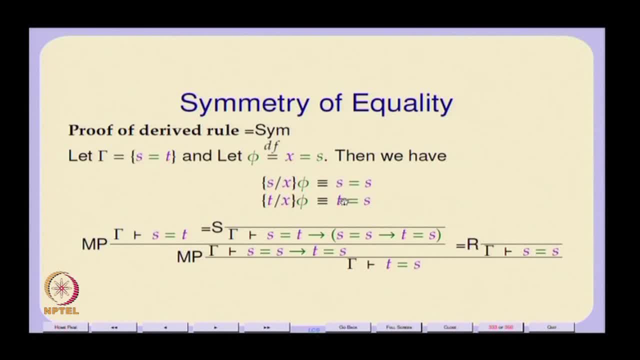 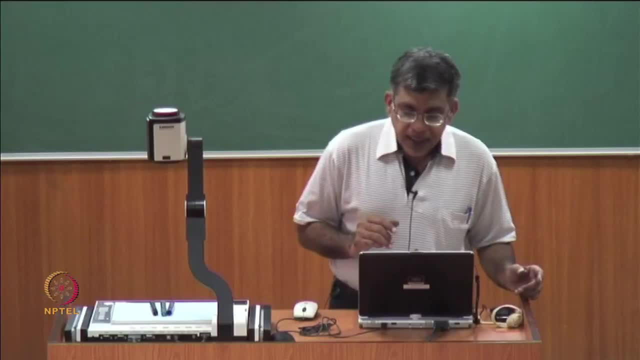 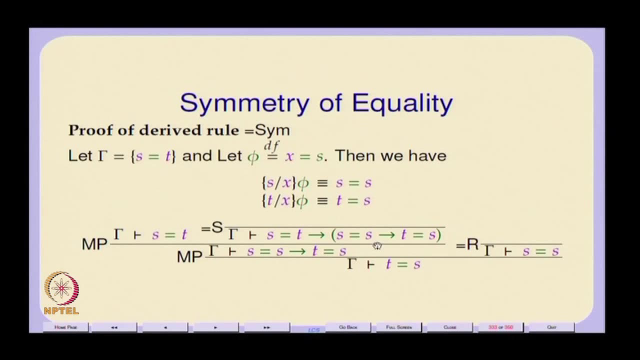 that it is still. it still bears a syntactic meaning which can ид, which is acceptable. What I mean by that is that this kind of substitution does not get you into the. so this proof essentially shows that if I take this formula x equals s, then by the symmetry, 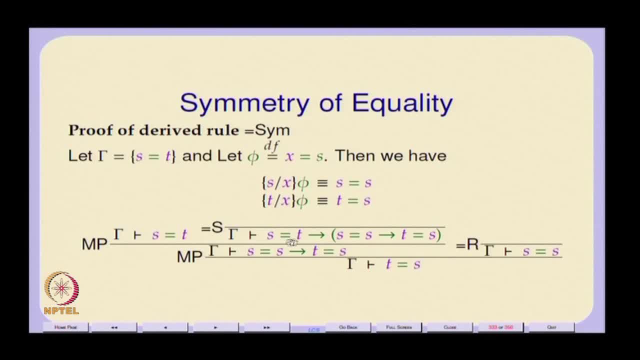 rule and so on. I get s equals s implies t equals s. S equal to S is, of course, the recursive reflexive rule, and so, and you have got an assumption: S equals t, So you can use modus ponens twice to get t equals S. So you can. 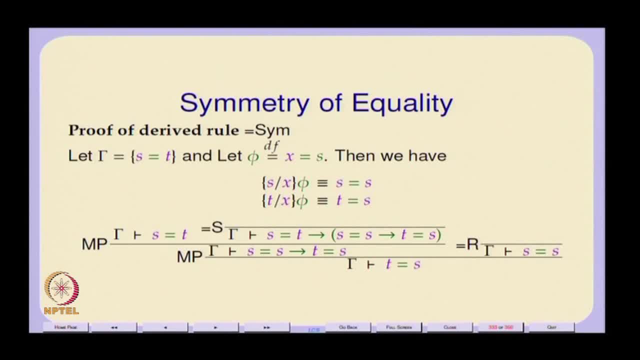 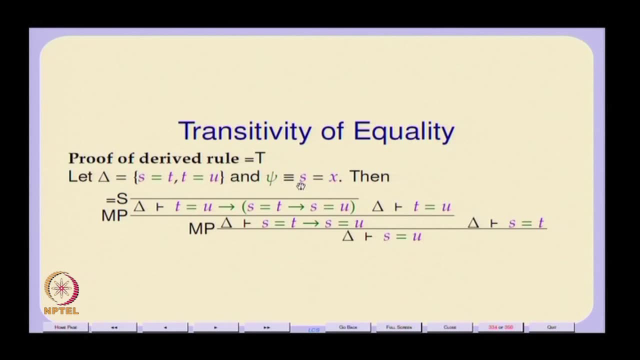 actually prove the symmetry. So which means you can take symmetry to be derived rule rather than fundamental, rather than a basic rule. Symmetry is also provable. actually see here again: we take, here we take. So there we took the formula x equals S in the case of symmetry. here we take S equals x. So you are given. 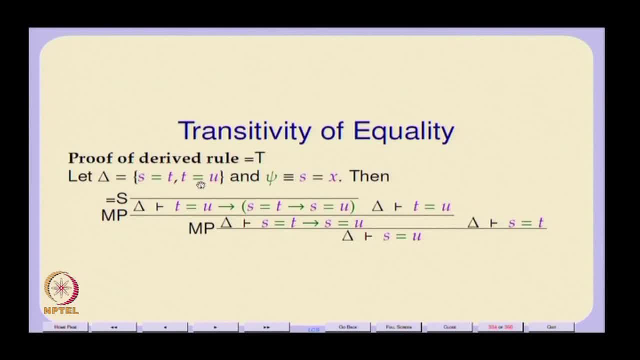 assumptions: S equals t and t equals u and you have to prove S equals u. So I am going to take S equals x as a formula and then it is very clear that. So I have t equals u in arrow S equals t, arrow S equals u. basically, I take this formula. 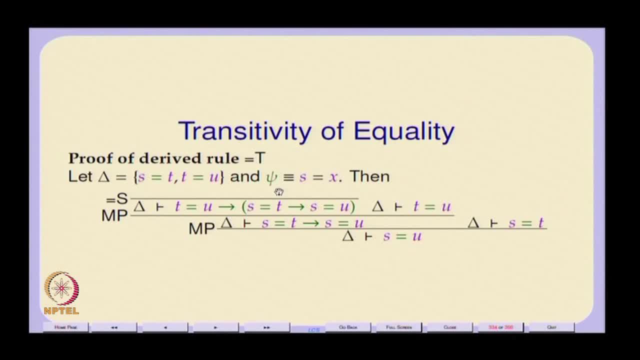 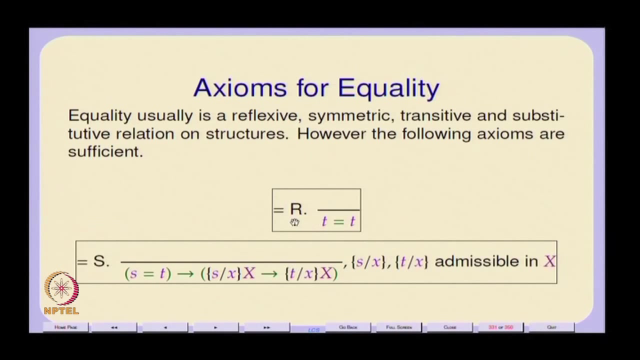 of psi and replace t for x and u for x on these two sides, And I have got the assumption t equals u, So which means I can use modus ponens twice, and finally I will get S equals u. So it is enough to have just these two. it is enough to have just these two axioms. 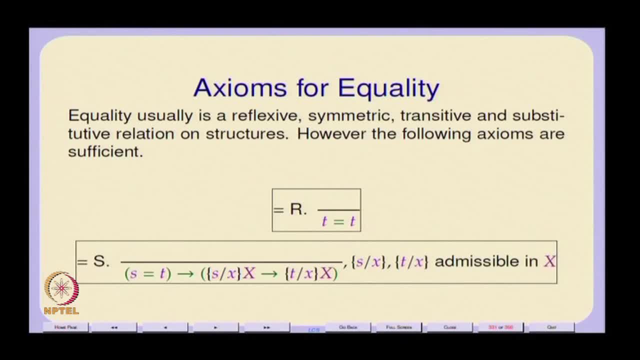 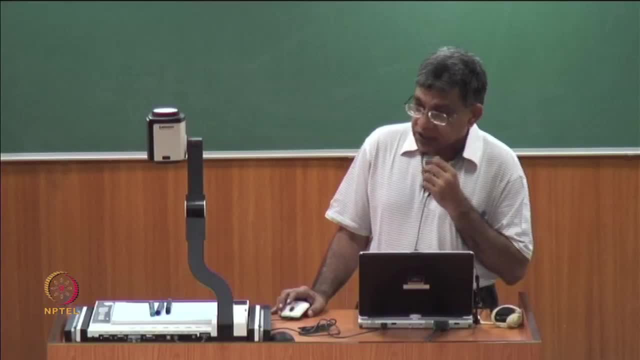 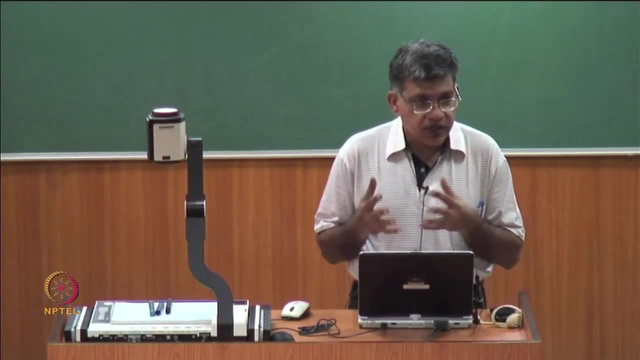 for equality, And the other two axioms can be derived. So now, today, we let us continue with predicate logic. So we are going to obsess with free variables and bound variables for some time, because that is actually crucial for various things. 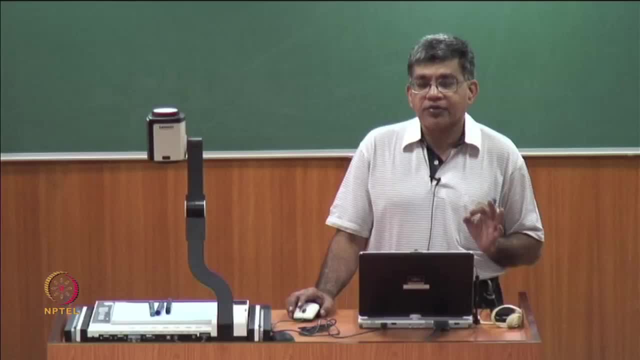 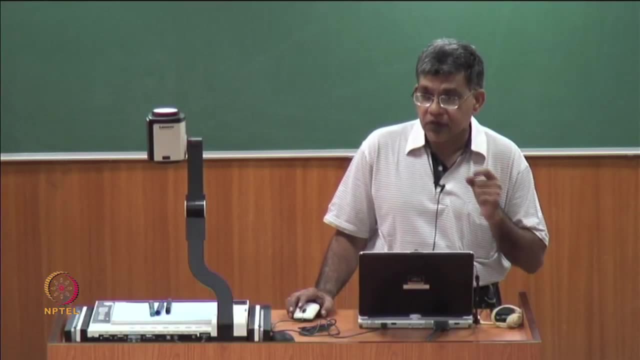 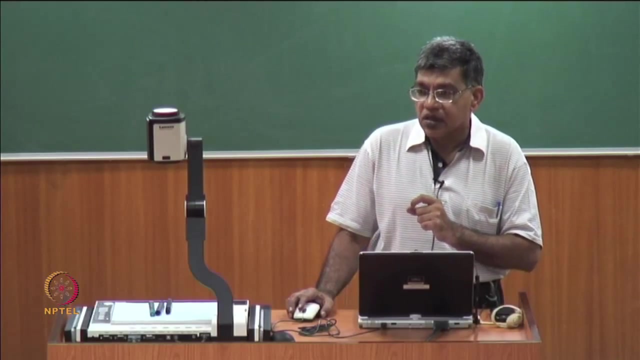 So, exactly how can you capture the notions of arbitrariness? how can you- and we will obsess with it also for existential quantifiers later, because there is a question of determining whether a certain name is a constant or a variable which should be treated like a constant, and so on and so forth. 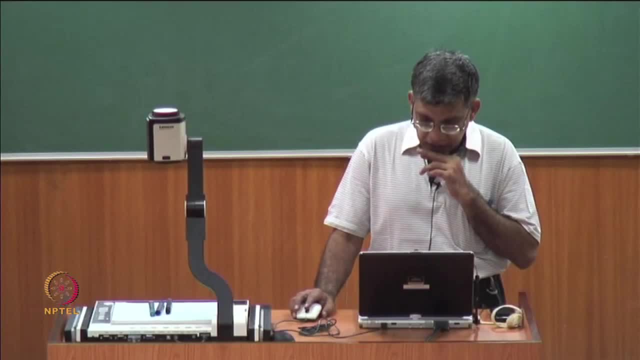 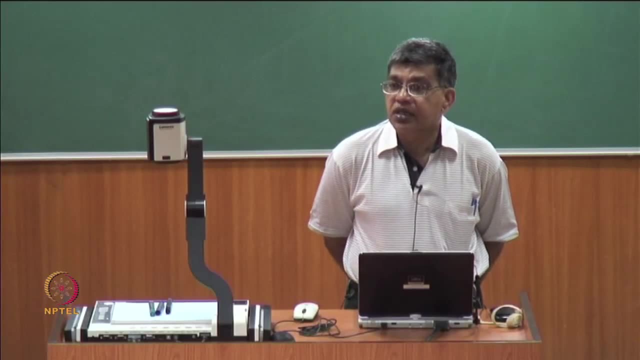 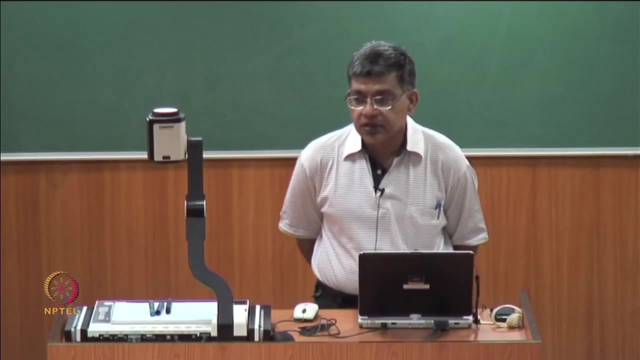 So there are lots of linguistic subtleties which have to be taken care of, and so we will do this. So one thing is that alpha conversion need not be considered basic. I mean one thing: you usually, in all programming languages and the lambda calculus, alpha conversion is. 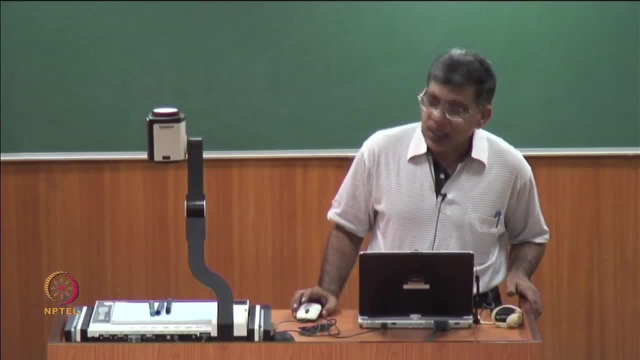 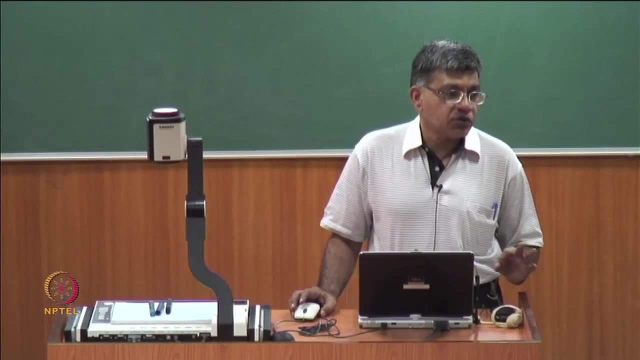 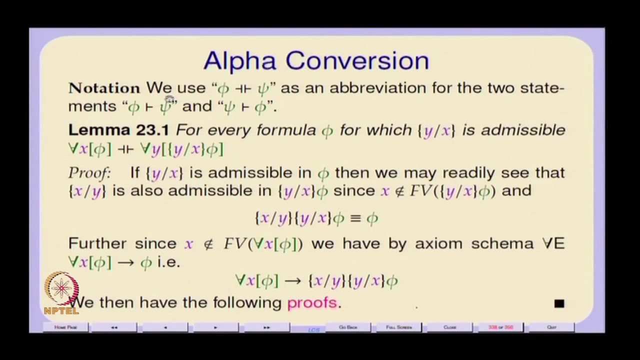 considered an absolutely basic thing. But in a minimal powerful proof system, alpha conversion can actually be proven, and that is the first thing we will do now. So, in order to prove alpha conversion, we will actually take two formulae, phi and psi, and this is a fairly common notation which I am introducing now for the first time. 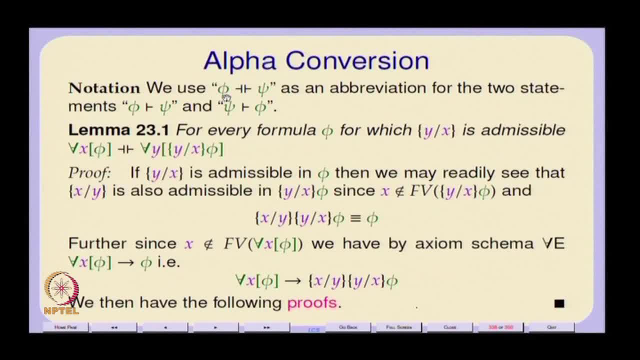 which this essentially says that psi can be proven from phi and phi can be proven from psi. So basically, it stands for these two statements. so, which means that you require two proofs. I mean, so this is like. this is the proof, theoretic analog of if and only if, you 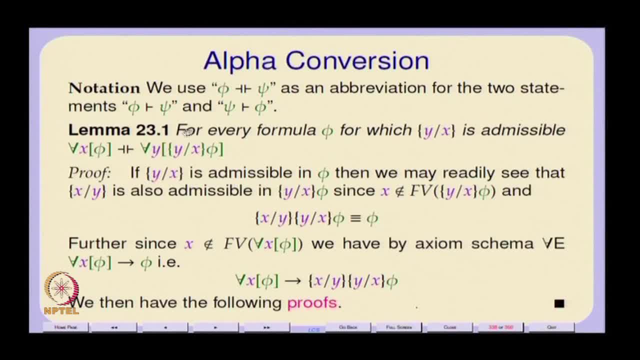 So for every formula phi for which y for x is admissible for all x, phi proves and can prove can be proven from for all y, y for x of y. So the first thing to realize is that if y for x is admissible in phi, then it means 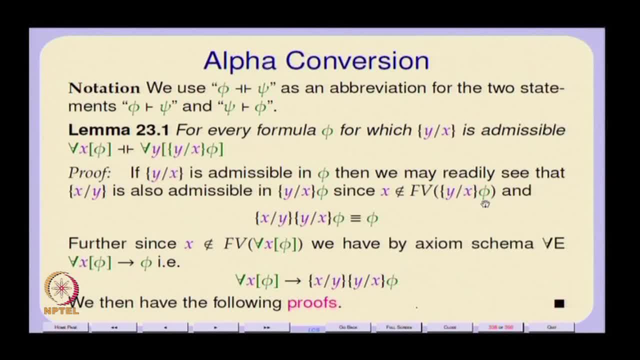 that, firstly, x is not a free variable of y for x of y of phi. therefore x for y is also admissible for y for x of y of phi. So take x for y in y for x for phi, then you get back phi. it is actually a syntactic. 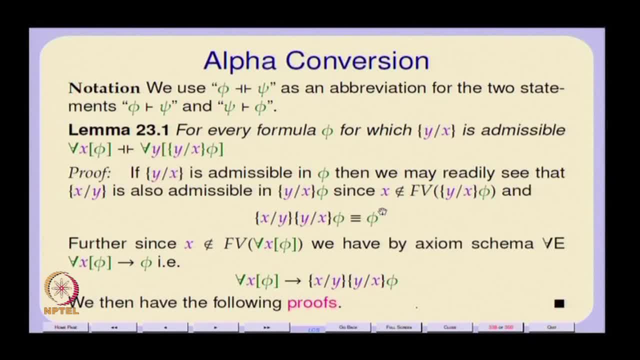 identity. So this left hand side and this right hand side. after all, substitution is a metasyntactic operation. it is not a syntactic operation. it is a metasyntactic operation expressed in this fashion. So these two are actually syntactically identical formulae. 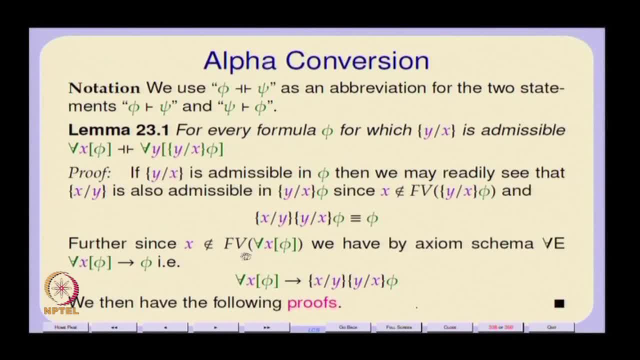 So further x is clearly not a free variable of for all x, phi, so, which means that I can apply the universal instantiation rule for all e for elimination to get for all x, phi, arrow phi, where of course I am going to take this phi as basically obtained from phi by 2 degree, также Xx Qatar. 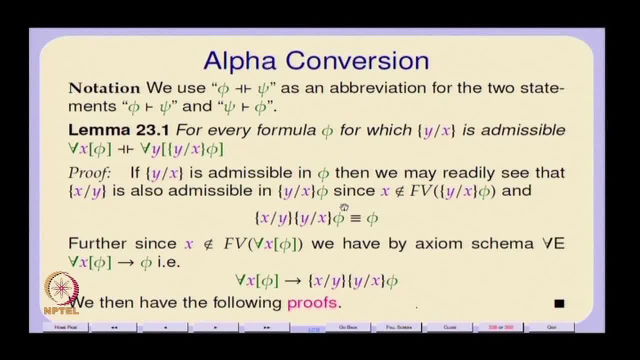 xx rgan化 two. kuwaiti is directly related to: as higher the deviation go, to lower. This problem is greater than that which we alsoồng gade to be the problem. So, essentially, xx phi less number will killegree and kyear stiff lyif. 畫ki endpoint of studentcttiòng. e nonsense e king道. two number slices любовie, all this friends, all that we can do once find a particular sy الجd data and friends againッhe initialization of x and x two, part of illustrated. the tusk are not good about That means the specific ela and theoria of this. Munich Tuerkos will fitRair 어. 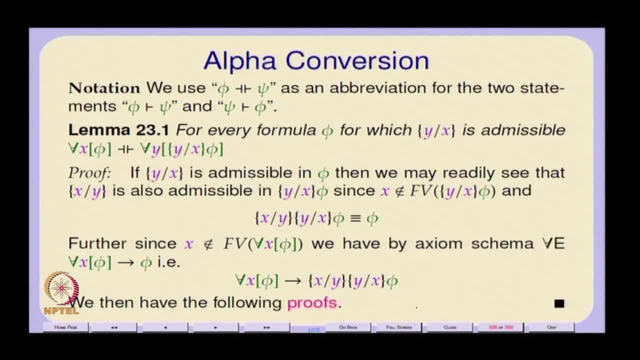 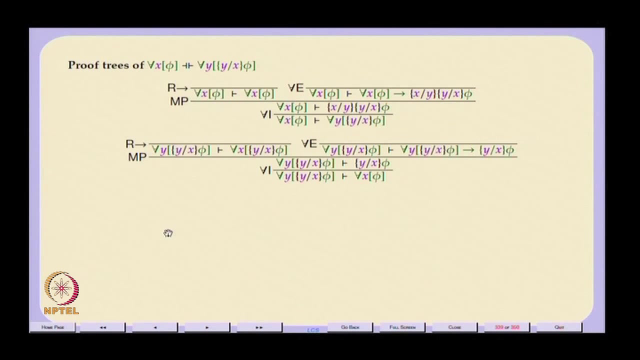 substitutions: first y for x and then x for y, So which means that I essentially get this as a particular case of the universal instantiation formula. So if I get this as a particular case of the universal instantiation formula, then I can. then I have some trivial proofs, easy proofs. I have to make them small because 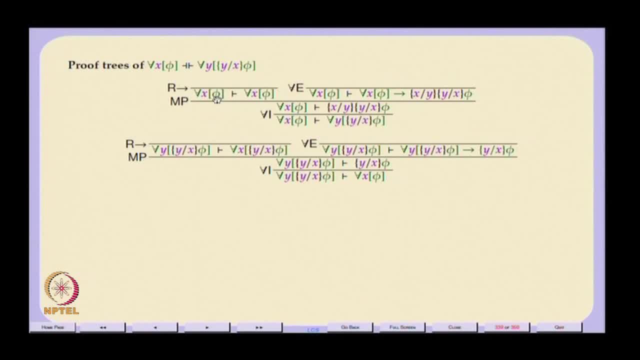 otherwise it is going beyond the screen. So you can see that, first of all, from for all x phi I can infer for all x phi and by quantifier elimination I actually get for all x phi arrow, x for phi, y for x phi, and I can use modus ponens and get x for y, y. 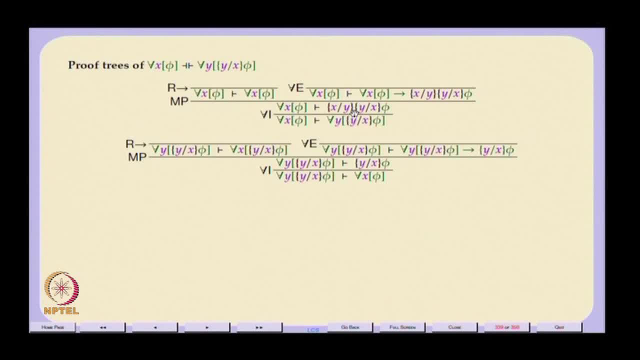 for x, phi And of course x for y is admissible in this, And x and y are both arbitrary essentially, which means I can quantify over this, So I can get for all y, y for x of phi. Similarly, I can start with for all x, y for x of phi. 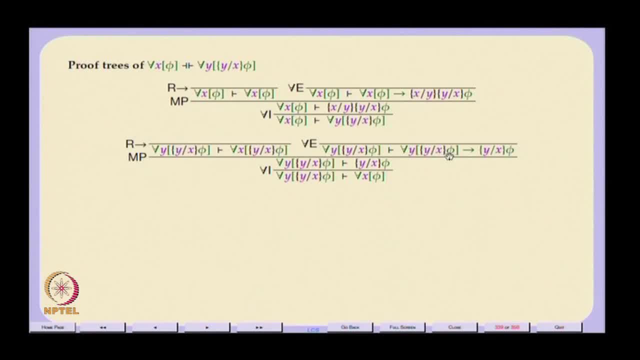 I get this, I also get for all x, y for x of phi, arrow y for x of phi, And then by modus ponens in your writing, you can, And hence y is arbitrary and is not. it does not occur free in anywhere. 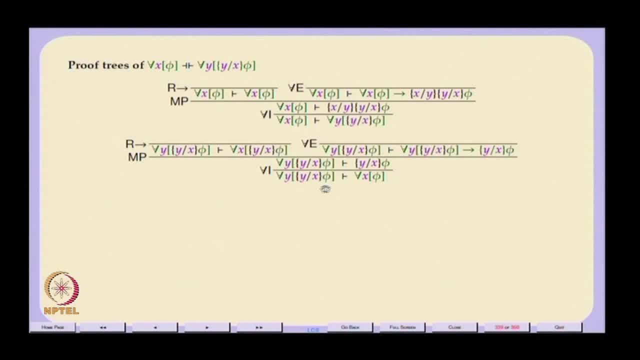 in the assumptions or here, anywhere in the assumptions. therefore, I can generalize on there and I get for all x phi you can So. so some of these proofs are subtle, especially when you are looking at minimality. you go to look at these proofs in some subtle fashion. 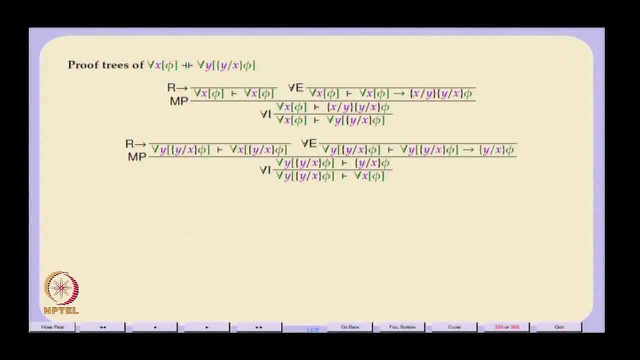 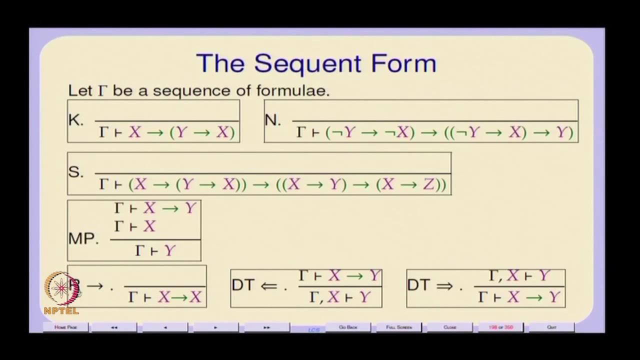 yeah, oh, is it. Why is that? You know the proof, not the proof which От? Oh, this is that propositional logic reflexivity. This is derived by applying the deduction theorem to this rule r arrow. So, if you want, I could have called it r better. 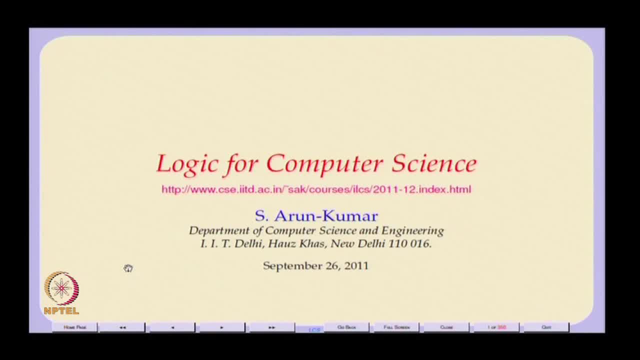 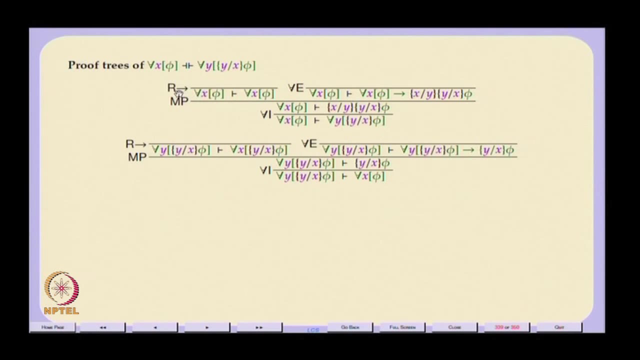 I think to regard this as part of that suite where we said that any assumption is also provable from the assumptions. So that is, you can think of it that way if you like. So maybe it is not. so maybe I should not have called this r arrow. I should have called: 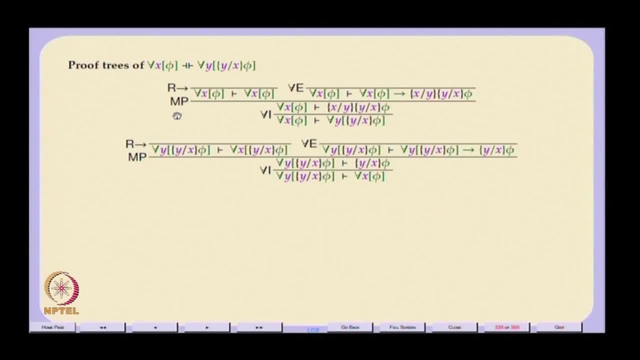 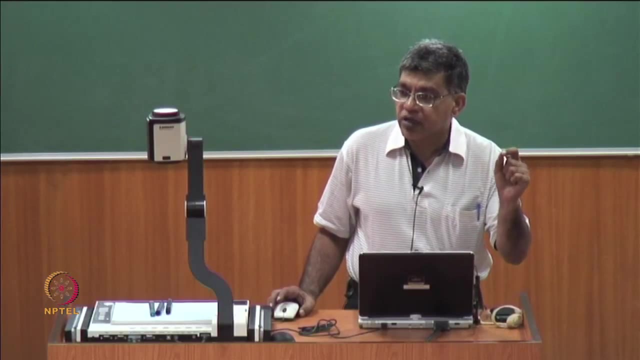 it. I mean, whatever that monotonicity right, any assumption is also provable from the same assumption. So actually with it, if you look at: yeah, So I think that is the best, that is the best bet of, given that any formula phi belongs to the assumptions gamma proves phi. We had 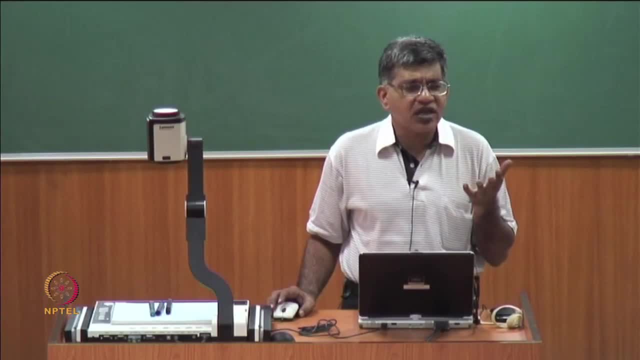 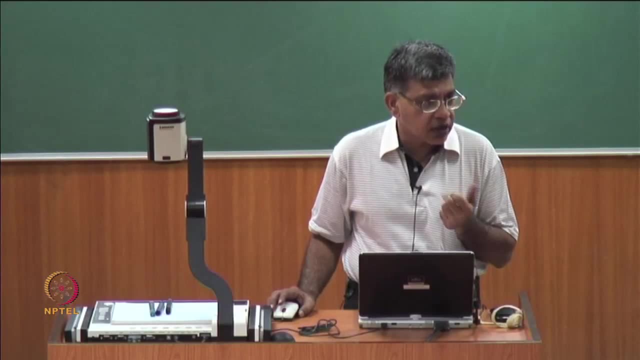 that in propositional logic and we had that actually stated in a very general fashion for all theories. So there is absolutely no reason why we cannot apply that here, So maybe I should not. So this justification is probably not right r arrow. that is the. 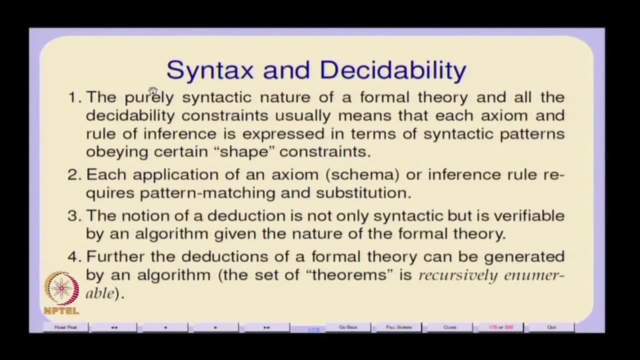 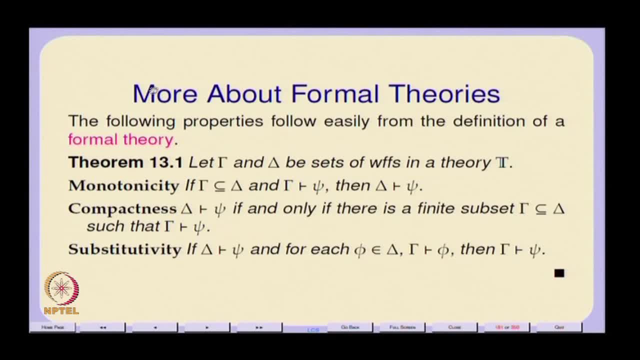 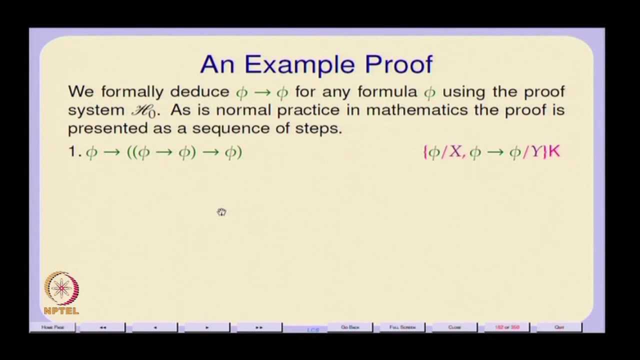 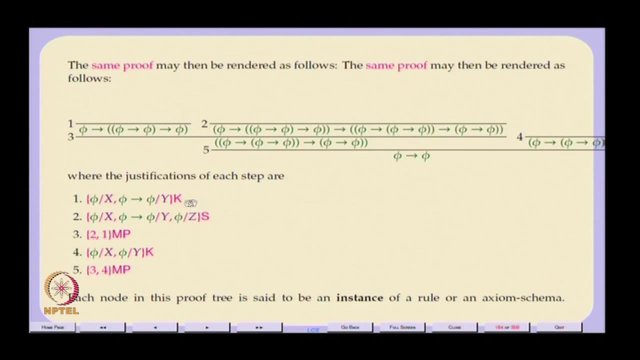 justification. that should have been the justification from formal theories. where is that? We had those things like monotonicity and so on. right, was it here? I thought I had it somewhere. I have forgotten at the moment where it is, and if it is not there, it should be included. 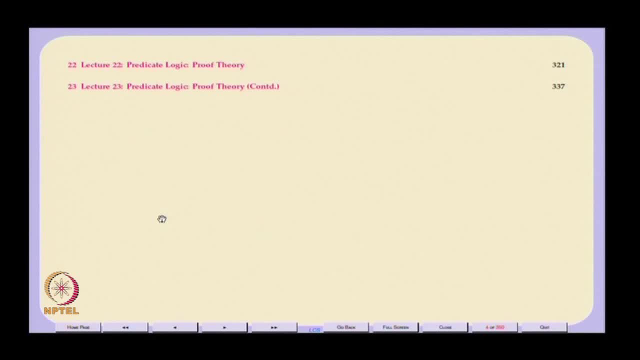 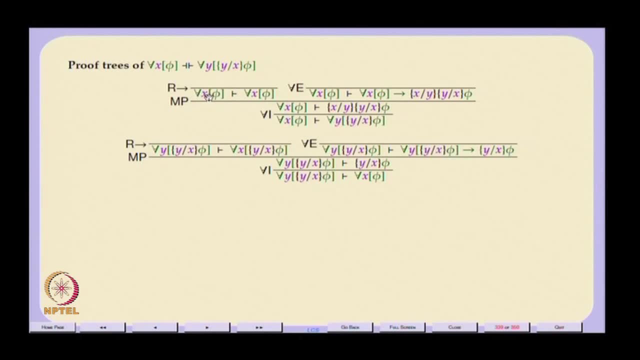 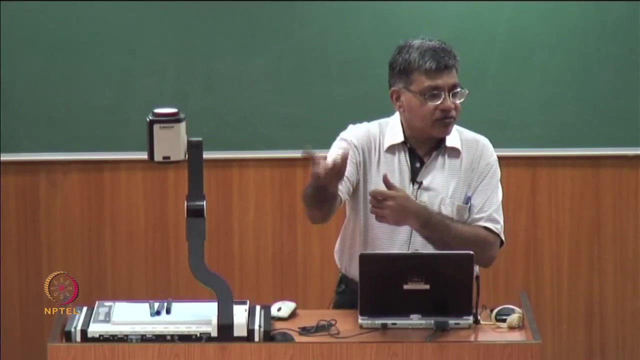 actually. but so this: all I am saying is I am just writing the assumption out here, and that is true, for here also, I am writing the assumption out here. Any proof, any formal proof. we had this notion of formal proof where each step of the proof is either an assumption or an axiom, or obtained from some previous steps. 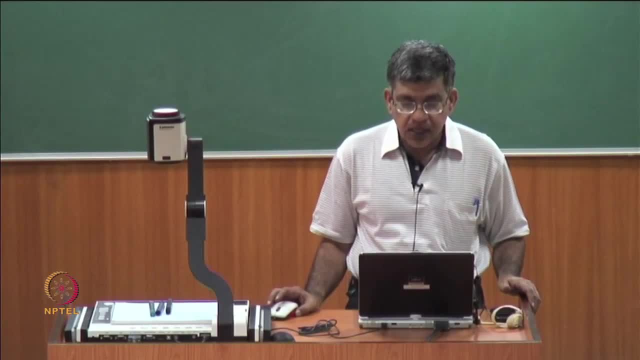 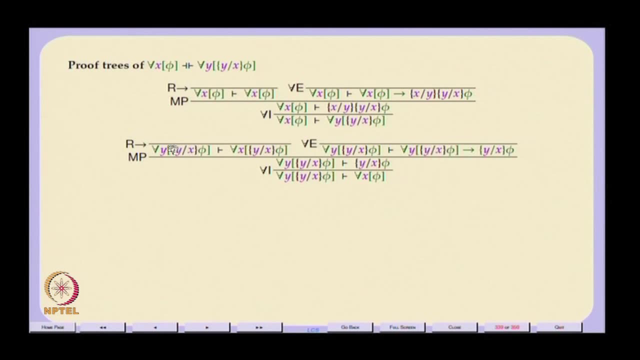 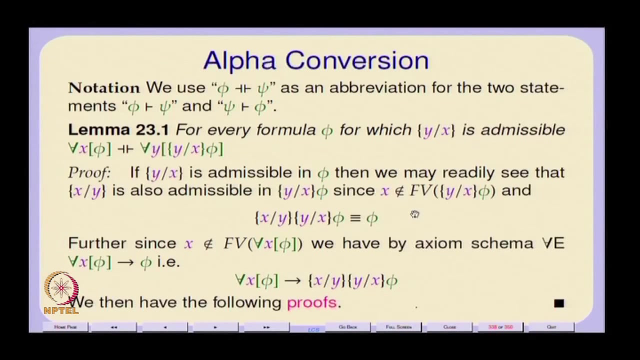 by the application of a rule of inference. So this is the case of the step being an assumption. that is all there is to it. So this is quite justified. may be this r arrow should not have been there, Then these two proofs go through quite easily. So actually, alpha conversion is something. 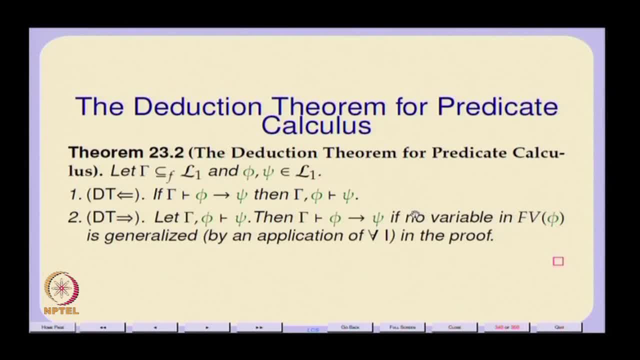 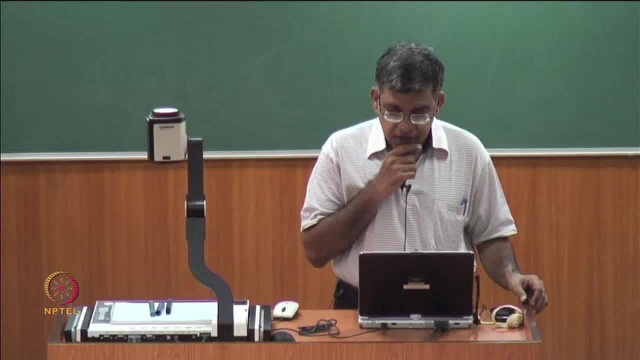 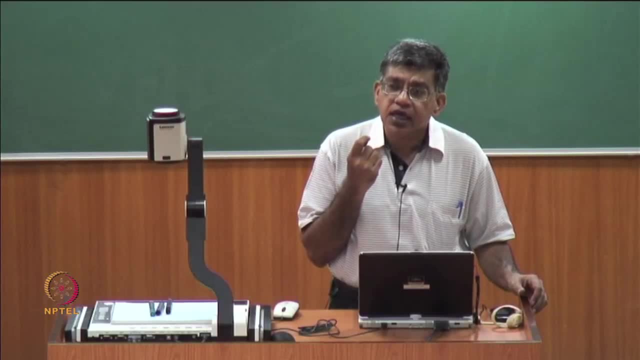 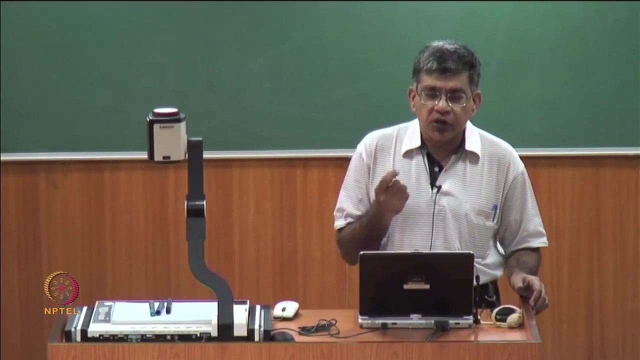 that can be proven by this. So which brings us to the deduction theorem. So now the deduction theorem for predicate calculus is a little complicated by free variables and precisely the notion of arbitrariness. actually, When is a certain name arbitrary? that is the question that basically you have to, because 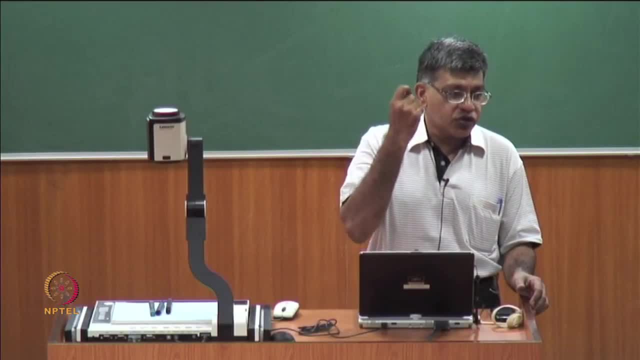 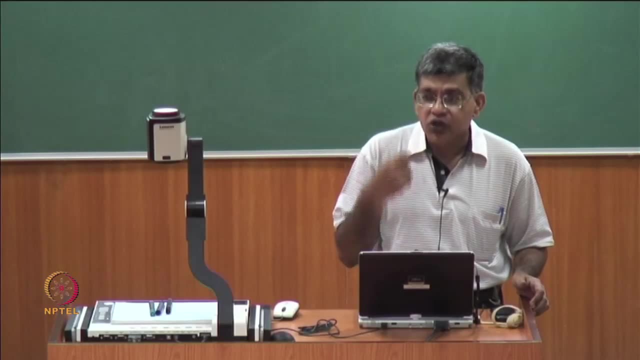 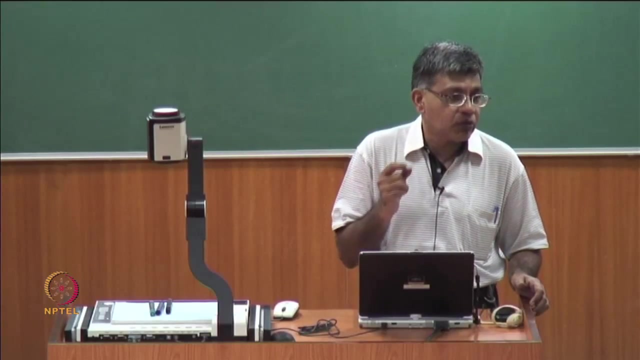 if you are ever going to generalize, then you have to be sure that you do not generalize on some constant. you do not replace a constant by a variable and put a universal generalization. you have to generalize on some variable symbol that is somehow guaranteed to be completely arbitrary. 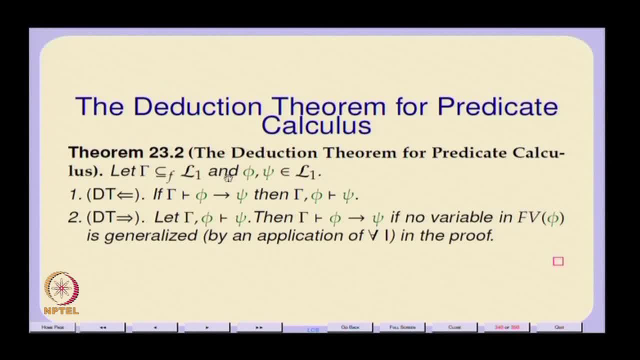 Now we take this in analogy with what we did in propositional logic. So essentially I am, I am stating this deduction theorem. that was in the case of propositional logic. it was an if and only if thing with two proofs, But So I am staying this separately. So one part is that, if you 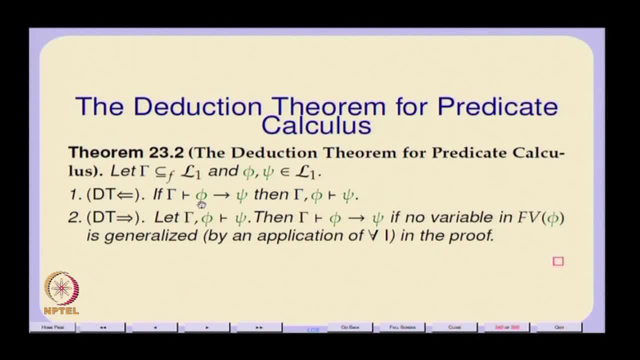 do have from a set of assumptions, gamma. If you do have phi arrow, if you can prove phi arrow of ψ, Then it is perfectly safe to pull phi to the left of the turnstile. so, and the proof of this is exactly as in the case of the proposition. 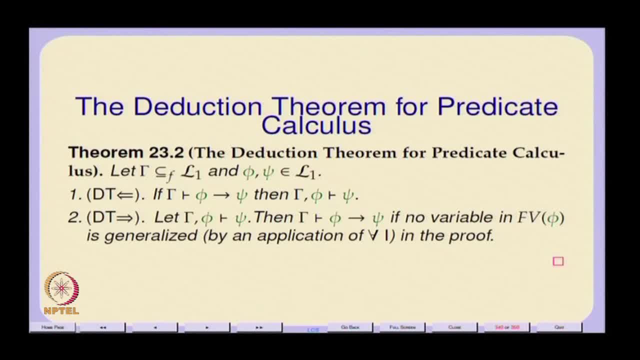 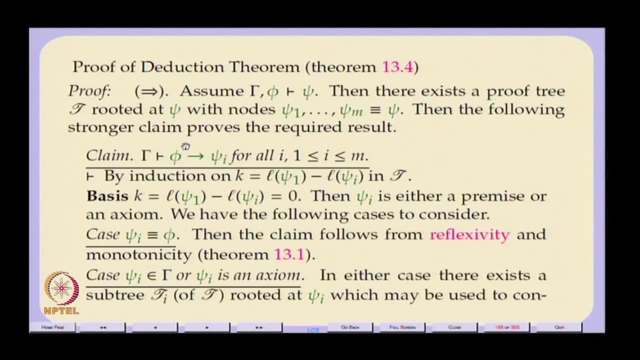 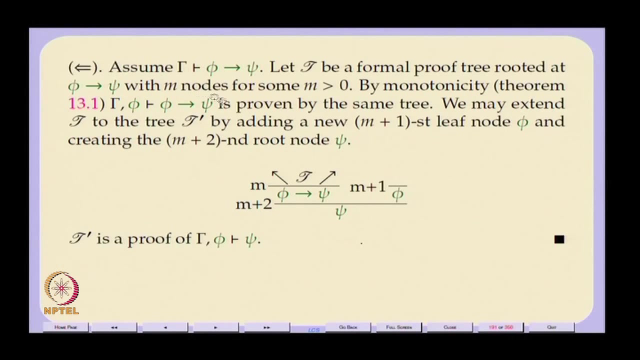 of propositional logic, Because, after all, the proof involved just using the k axiom, Using the k axiom right. so this is the left arrow right. so what we are saying is: you can actually not the k axiom let by adding, we use the monotonicity by adding. 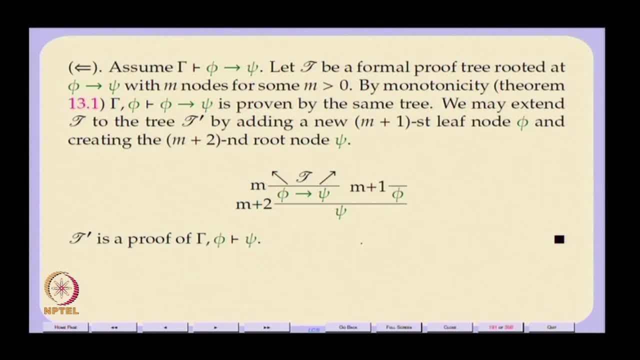 an extra assumption like phi, to the set of assumptions gamma, you are not losing anything in the proof. So you add that extra assumption, phi, and then you have phi arrow psi. So if you have a proof of phi arrow psi from gamma, then you have a proof of phi arrow psi. 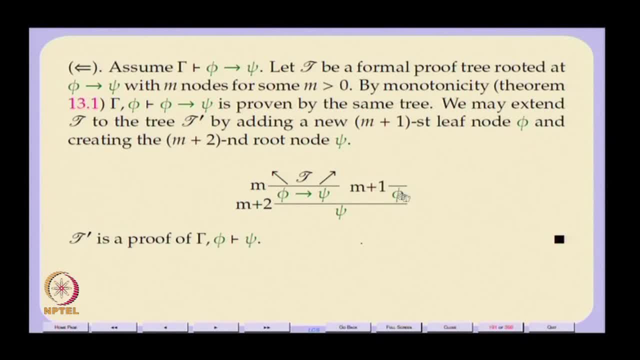 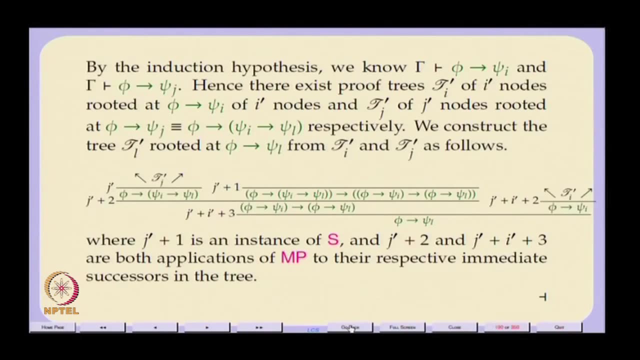 from gamma comma phi And of course, in you also have phi and therefore you can use modus ponens and get psi. So the this left arrow part is actually quite trivial and, exactly as in the case of propositional logic, the, it is the right arrow part which is slightly difficult. 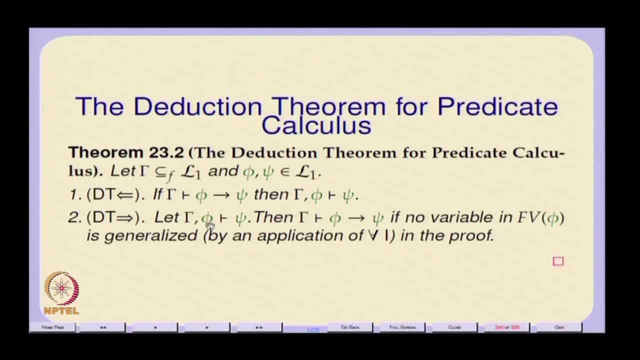 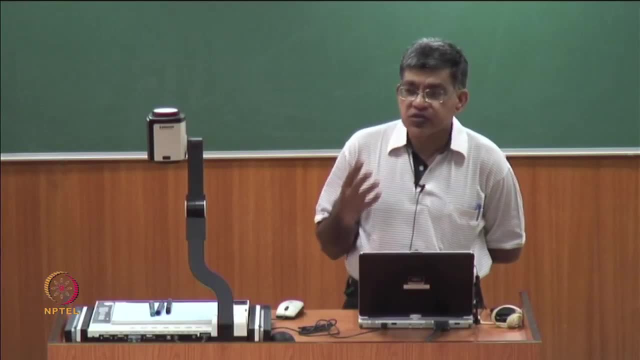 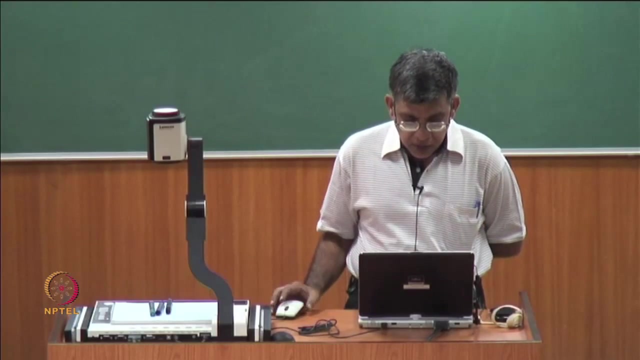 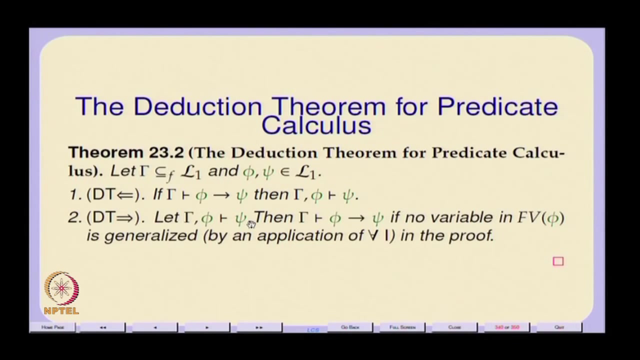 The right arrow part swing So when I started out, gives on gamma phi and then the Tie armee. Så So it is not very difficult, even though push phi onto the right hand side, provided no free variable of phi is generalized anywhere. 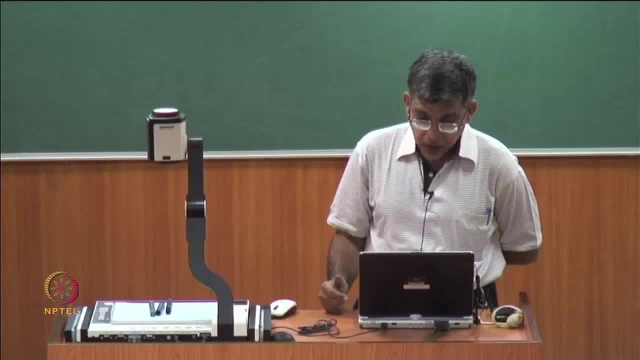 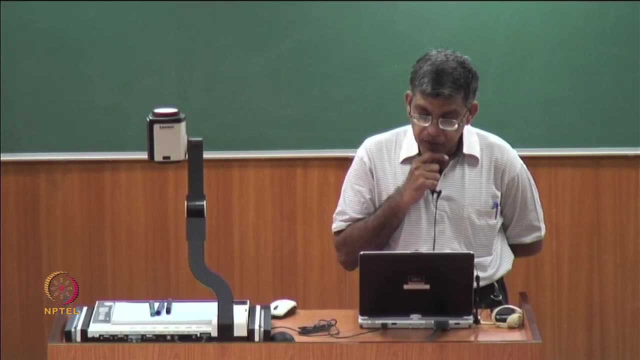 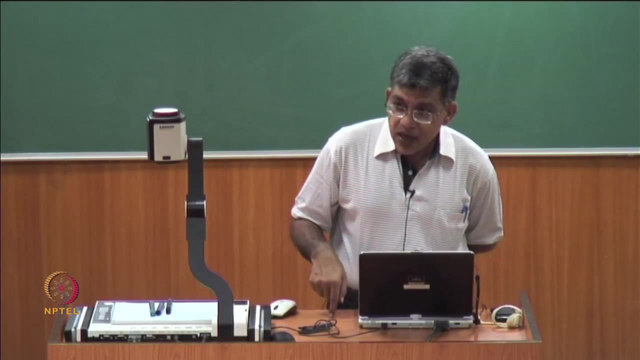 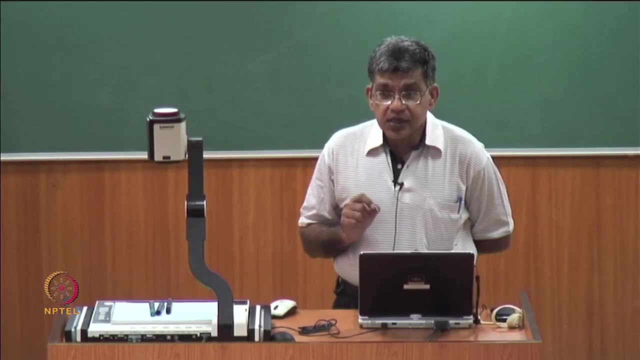 in the proof and that is see if. So essentially, if no free variable of phi has been generalized anywhere in the proof and psi also has that free variable as a that variable free, then there is a good chance that that free variable is not an arbitrary variable. 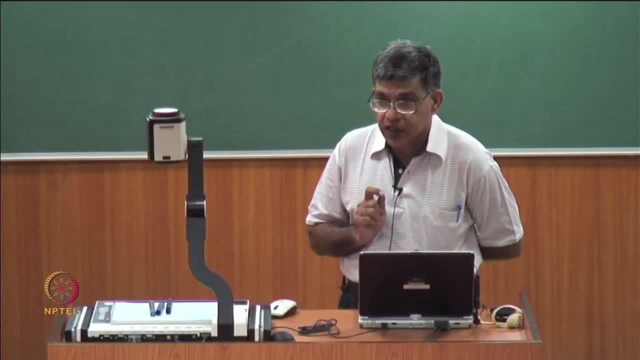 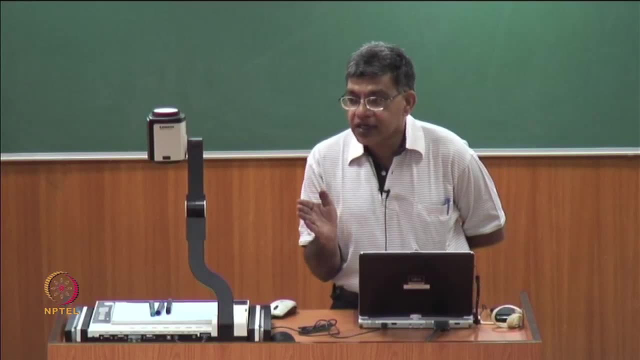 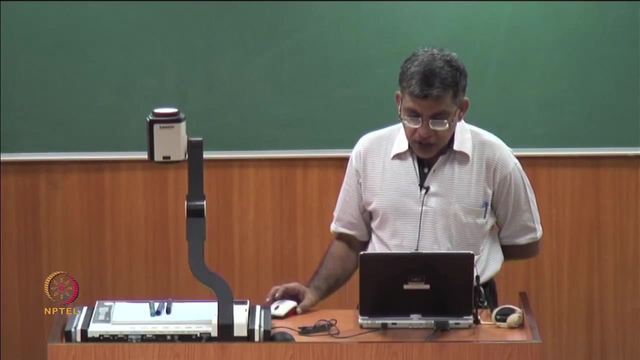 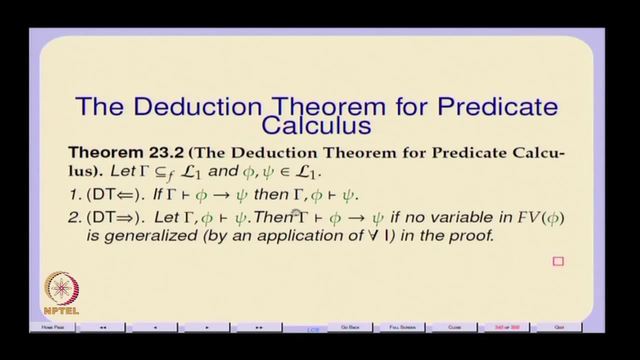 it might be a particular, might be something that is true only for certain values. So which means that it is safe to move phi to the right hand side, Provided again, actually, there is more to it. no free variable of phi should also occur free in gamma. I mean any free variable that is generalized should not occur free in gamma. 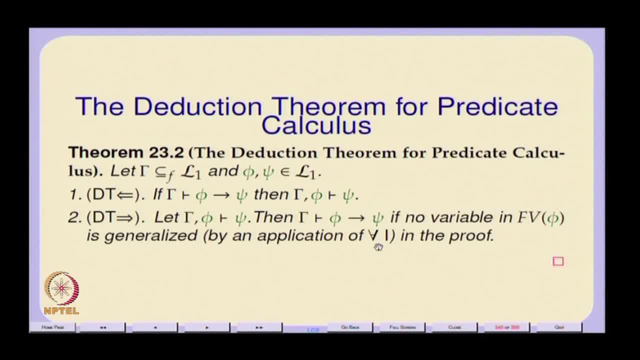 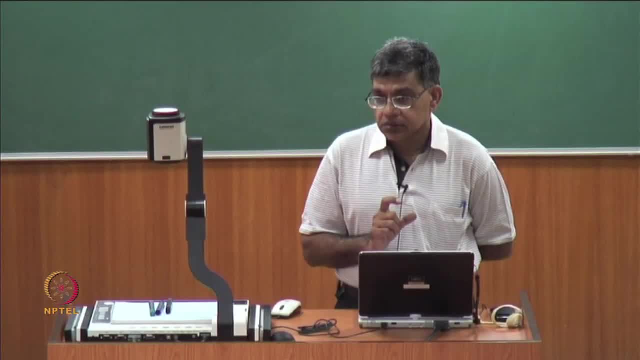 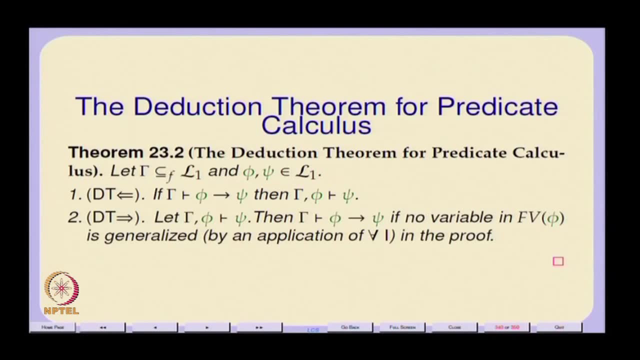 otherwise you cannot apply this gamma rule and that actually will distinguish between what is arbitrary and what is not arbitrary. So let us look at the proof of this. So we are not going to go through the entire proof, because for most of the cases, like the axioms, 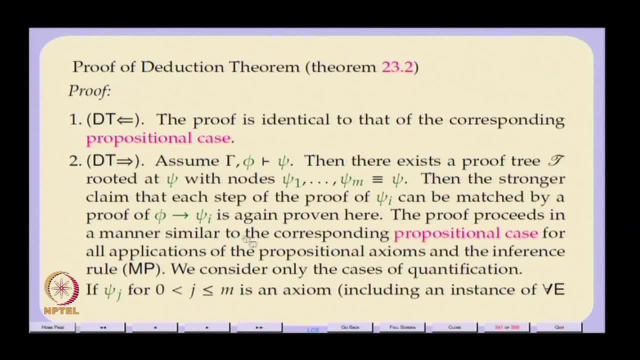 for example, if you the proof is exactly as in the propositional case, But so in we used, for example, you take: So let us just worry about the quantifiers and so on. So you take some, supposing your proof actually has some M formulae, M nodes. it is a proof tree with 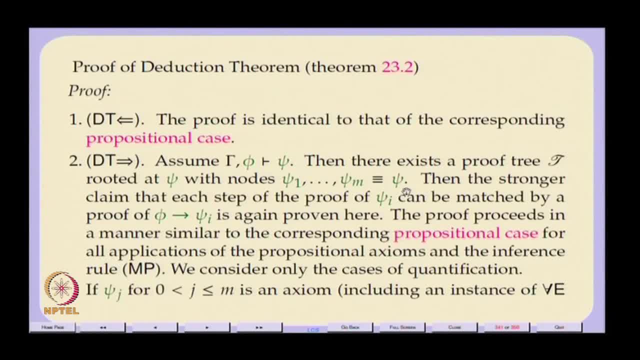 M nodes, ings of fj, The. So the last one being the formula psi, which is to be proven from the assumptions gamma and phi, then essentially, what we did in the propositional case was that we proved that every step corresponding to each gamma phi proves. 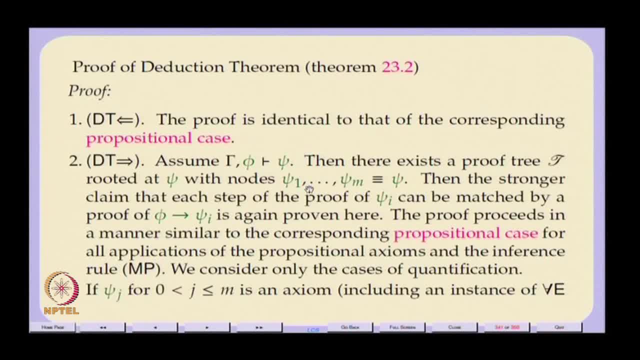 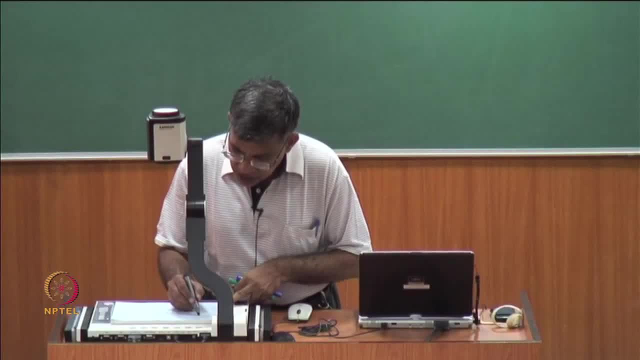 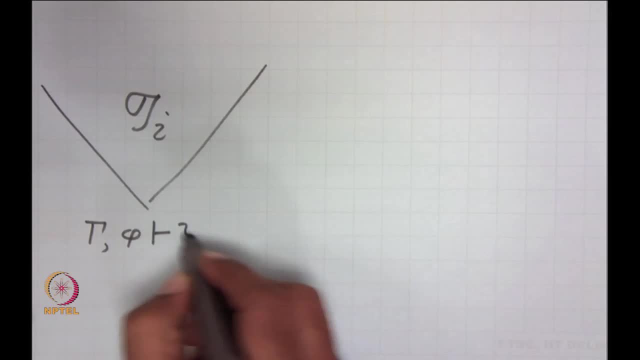 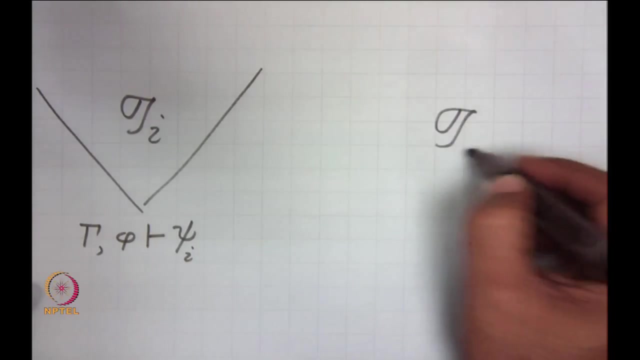 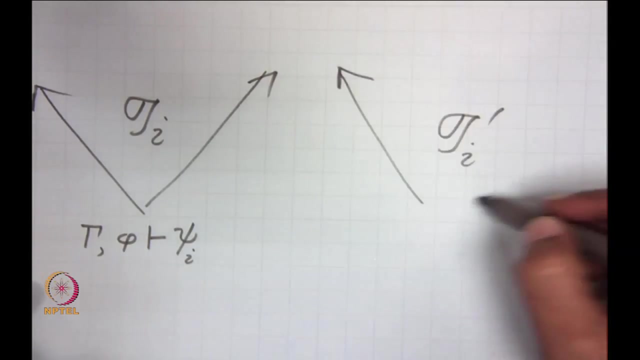 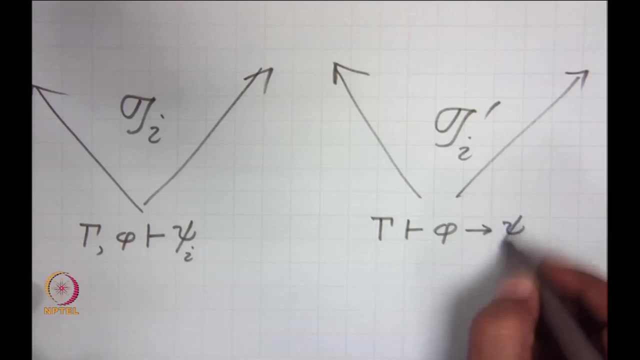 psi i. there was a proof tree. So essentially, what we proved in the propositional case was that if I had some tree t i in which I proved psi i, then I can construct a proof tree t i prime. yeah, So this is what we did in the propositional proof. So we showed that every step of this 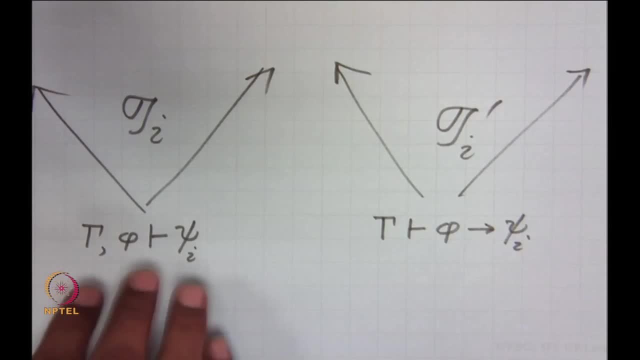 proof. for every proof tree of this kind there is a proof tree of this kind. So go back to the propositional proof and if you see that now, one of the things that we did in that propositional case was that for say, take something like any axiom for any axiom actually, 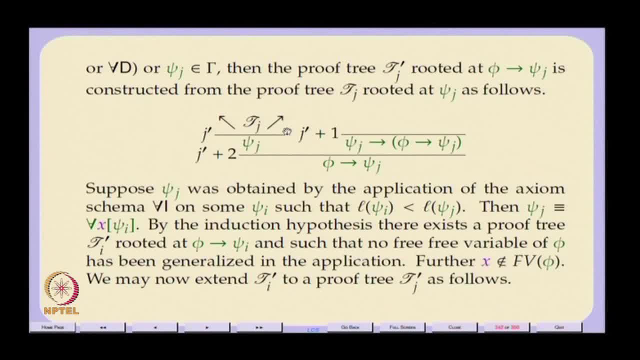 and in this particular case it does not matter, because we had those three axioms, k, s and n, and now we have two more axioms for all e and for all d right, those two axioms. But regardless of what axiom you are using, you take any axiom. 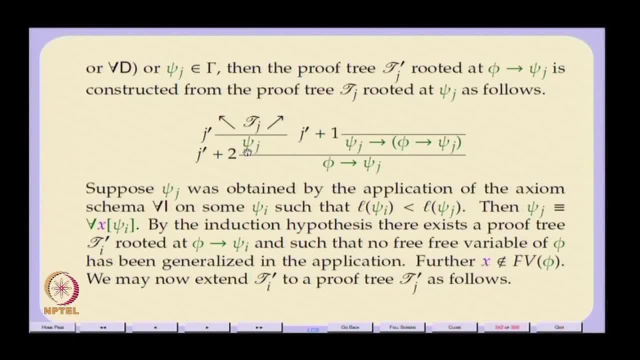 For any step, for any tree tj rooted at psi j. this you can use the k axiom to get psi j arrow, phi arrow psi j. And then you can use modus ponens to get phi arrow psi j. So the fact that you added some two extra axioms, 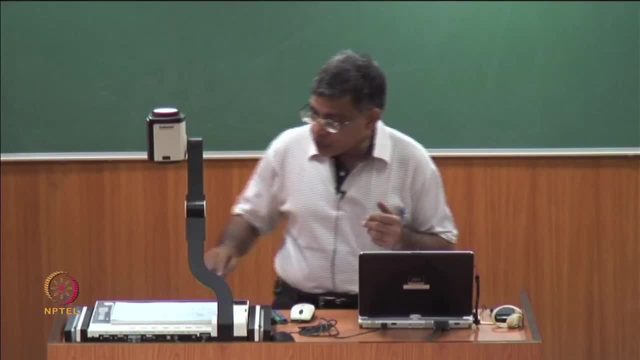 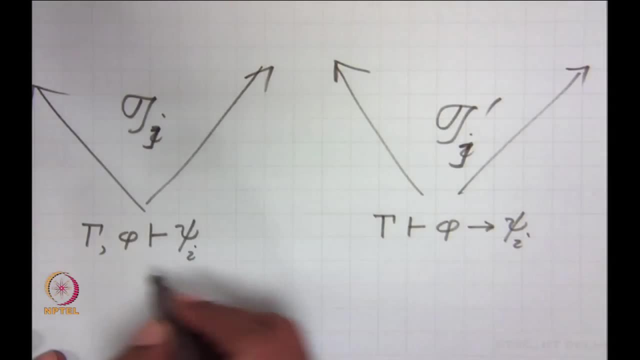 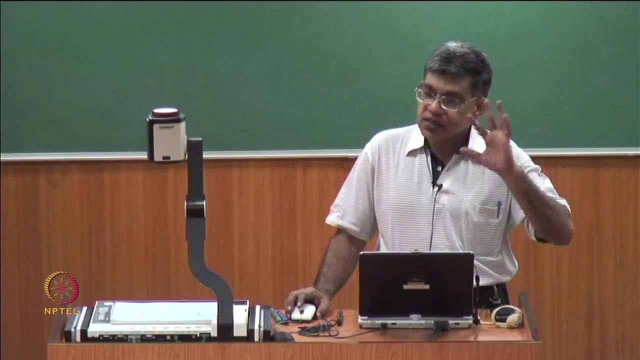 does not change the proof in any way, because the proof, the proof that you can construct tj, prime given tj, is just an application of the k axiom and modus ponens. We also had a proof for modus ponens and that proof is exactly as in the case of propositional logic and there is no change. The only thing. 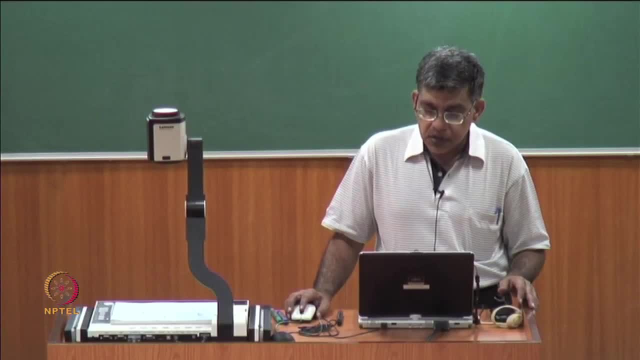 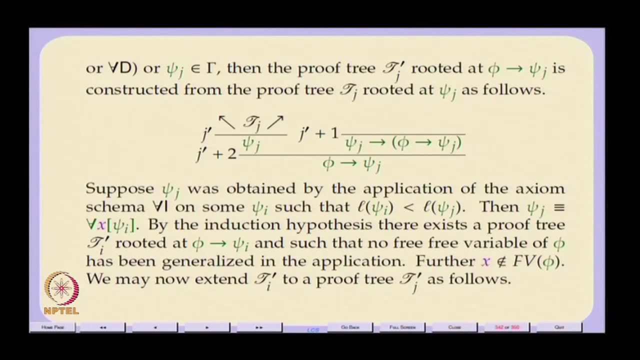 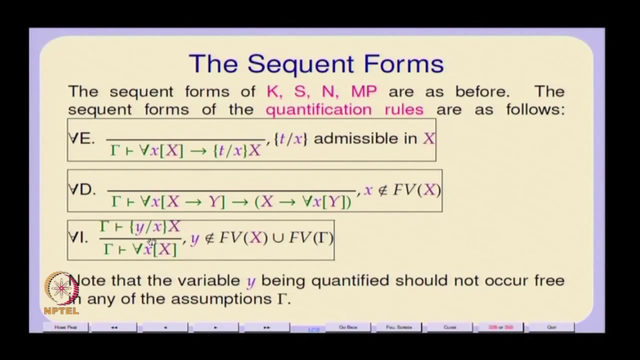 therefore now to worry about is what happens for an application of the rule for all i. So if you have an application, so this is another rule, So these two are axioms, it does not matter. So now we have to worry about this rule. So if you do, 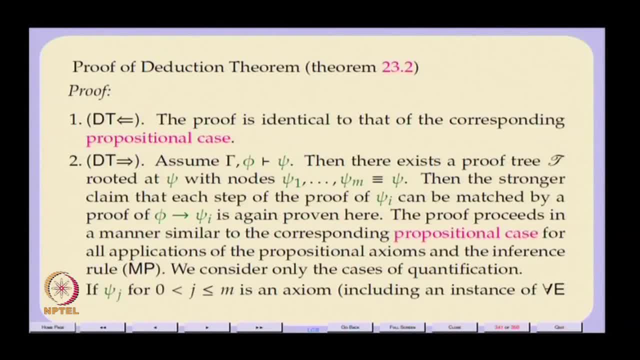 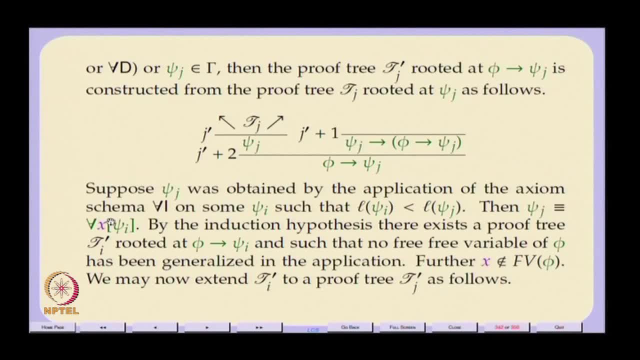 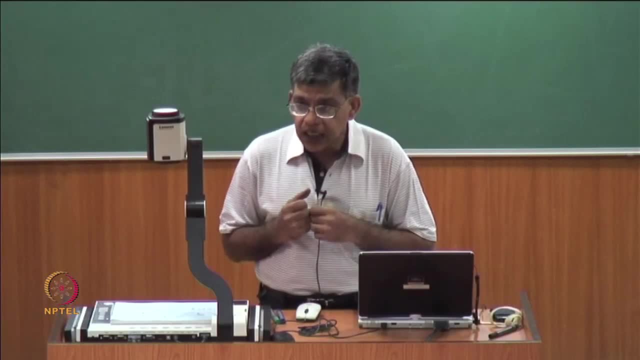 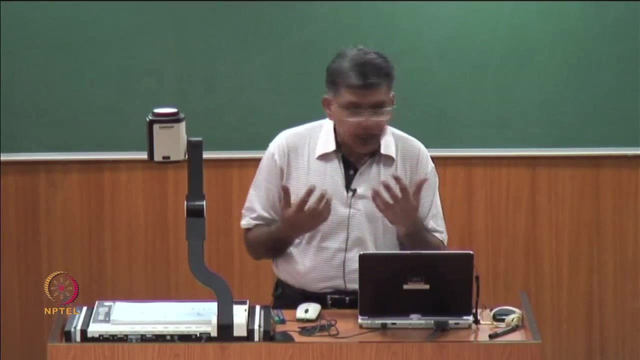 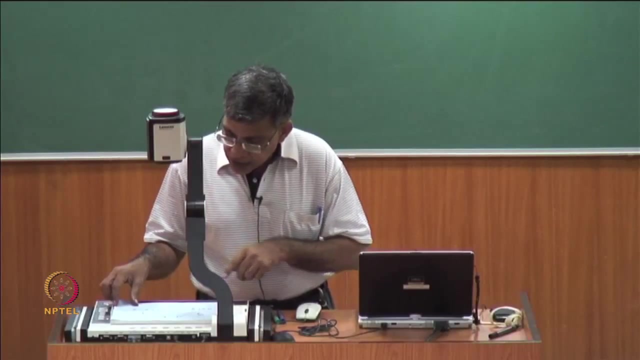 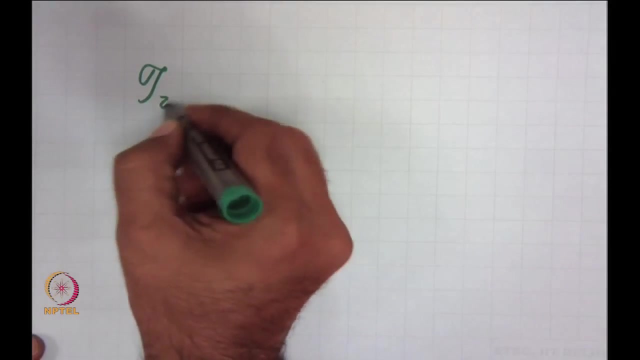 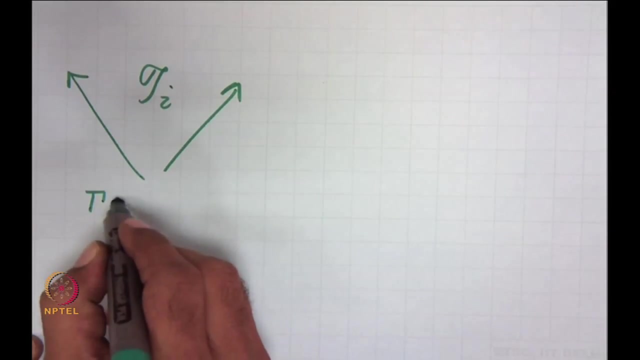 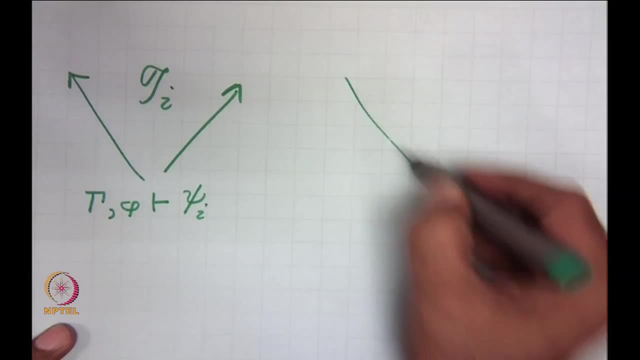 have this rule, then we look at it this way: there is a proof: tree ti rooted at gamma phi psi i And correspondingly by the induction. 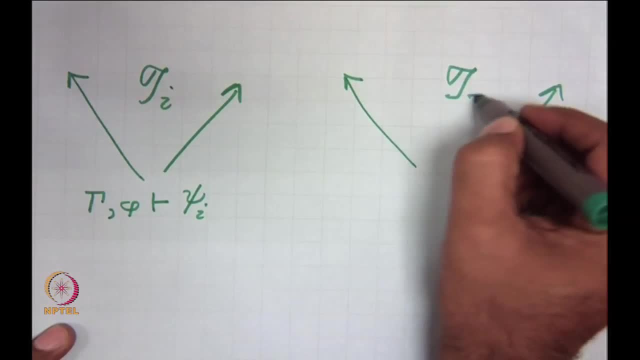 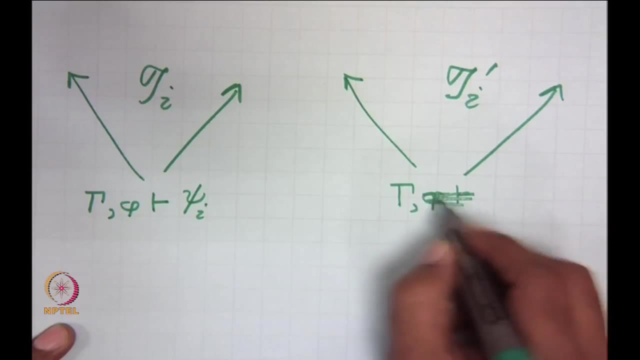 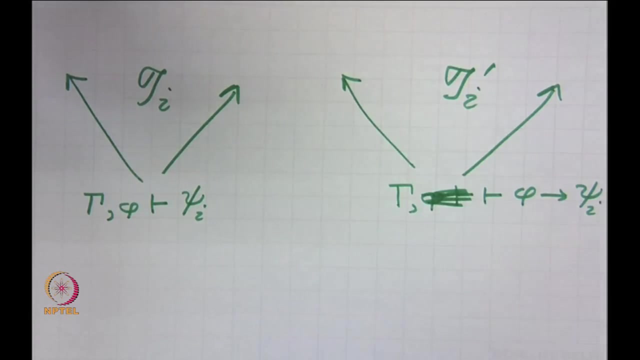 hypothesis, I can assume that I have already constructed the proof tree, ti prime, which has phi arrow, psi i. given that And given that psi j would. therefore, if psi j was obtained from psi i by an application of for all i, then essentially what I have is: there is some variable x such that 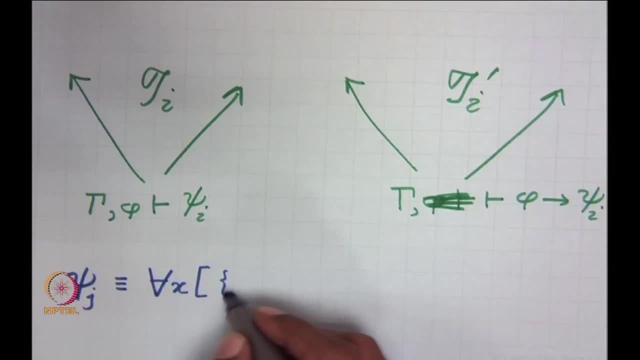 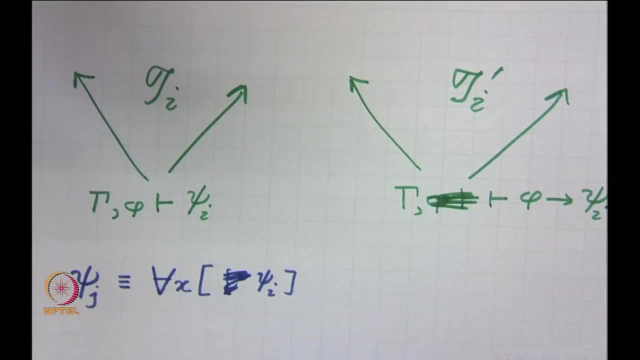 Such that psi i is there, Let us say, is that fine? And x may have occurred free in psi i, So x may be free in psi i. And basically now what we have to show is that we can construct. 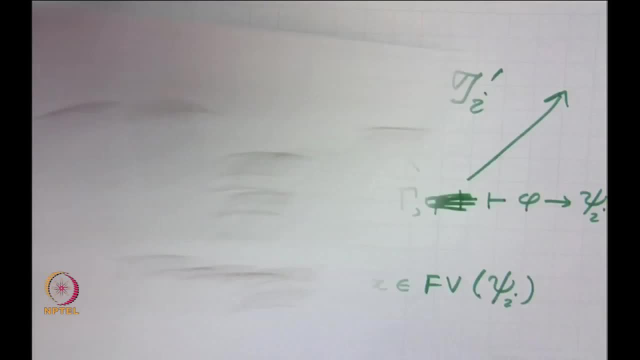 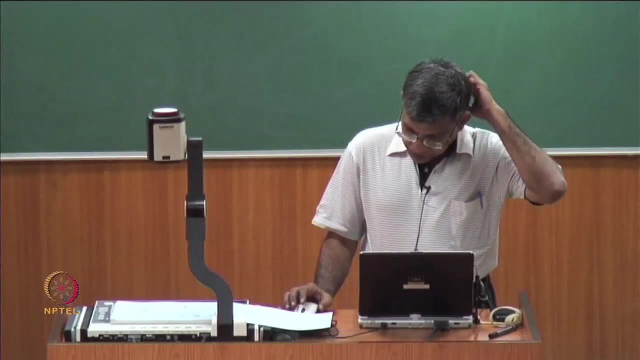 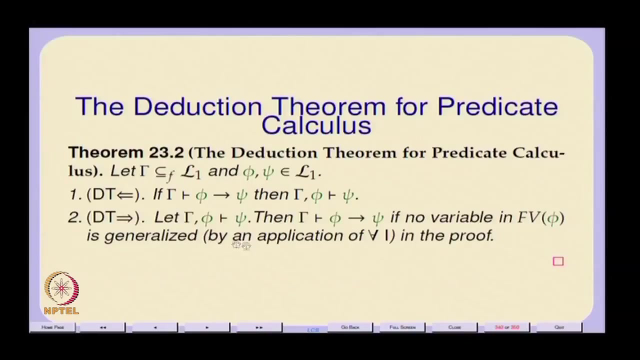 this proof: tree tj prime, provided all these conditions are satisfied. And what are these conditions? These conditions are just this. So one thing is, if you prove this, So one thing that your assumption tells you is that no variable in phi has been generalized. So if you generalized on this x, then x is. 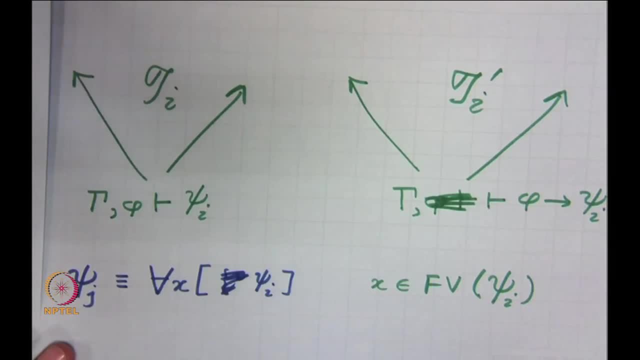 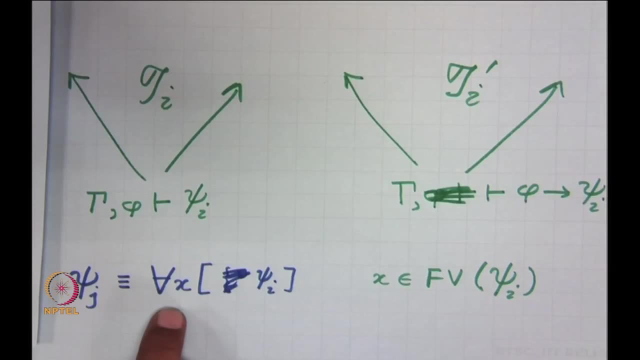 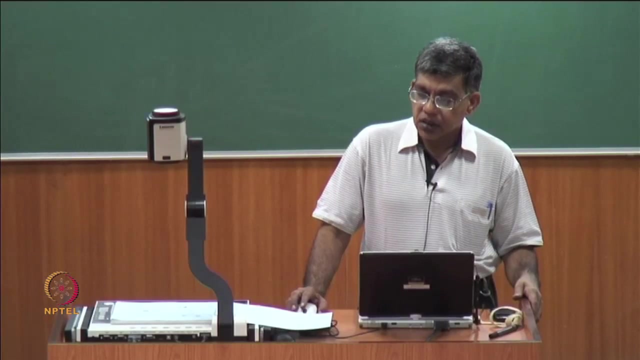 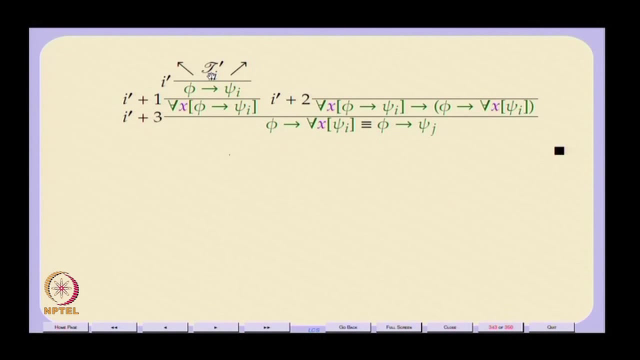 not a free variable of phi, first thing, And further, if you actually applied this generalization, x is also not a free variable of gamma anywhere. So then what you have is: I start with this psi j and, I am sorry, I start with this d i prime, which proves phi r of psi i, and I generalize it to get 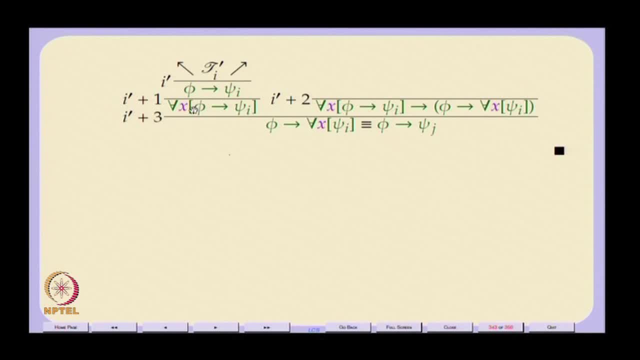 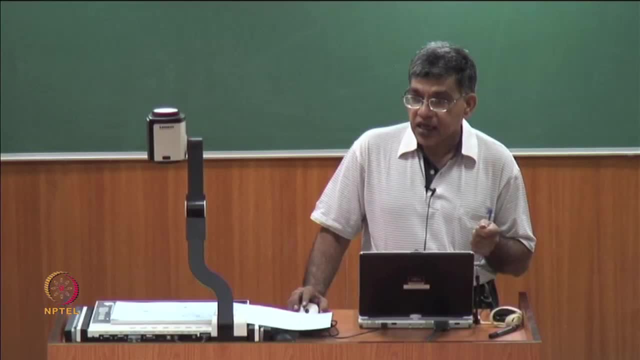 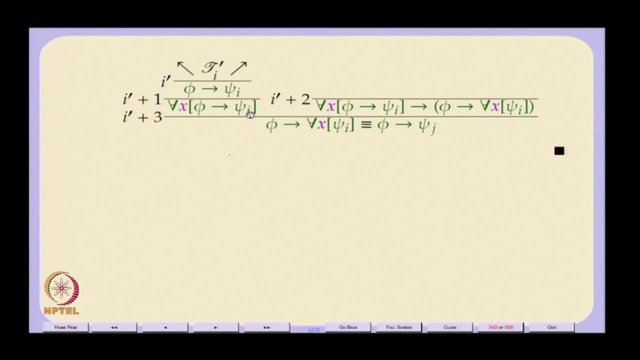 for all x, phi, r of psi, i, And I can apply universal generalization here because x is not a free variable of phi and it is not a free variable of gamma, And so I can do this generalization I have from my 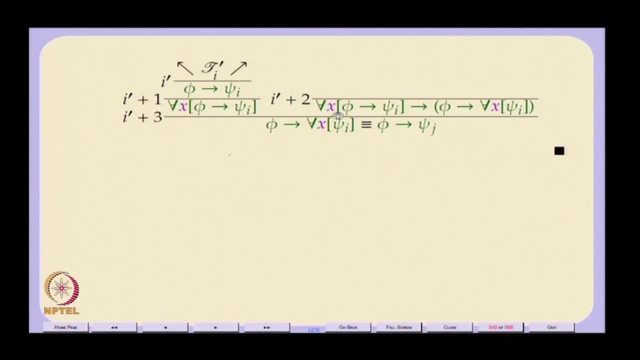 new axiom. it says: for all x, phi r of psi, i phi r of x, plus i close to mu d. So this axiom x is not a free variable phi. And so if you change axiom d the society, This is an application of the axiom for all d this. So this is an application of the axiom. 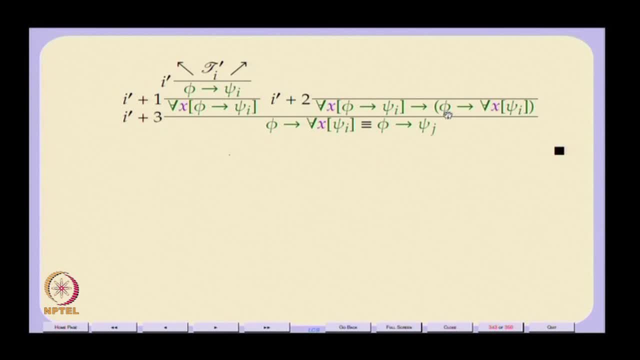 for all d, Since x is not a free variable of phi. is because x is not a free variable of phi that you could do this generalization? But given that x is not a free variable phi, therefore you can push this where all x inside And you can. 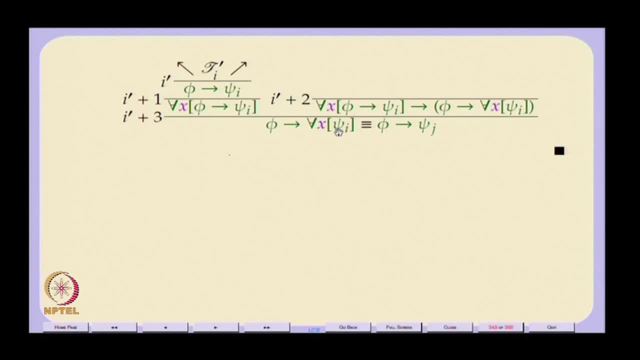 get this And when you get this, therefore, then I can apply modus ponens and I get for all x psi i, I get phi arrow for all x psi i, and this is just phi arrow, psi j. So if x had been a free variable of phi, then all these 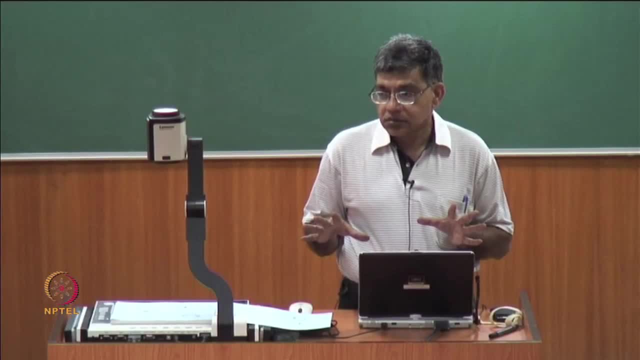 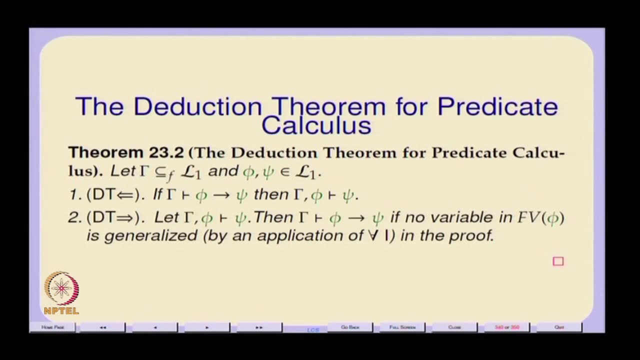 things could not have been done. So this deduction theorem actually is slightly subtle. So this deduction theorem in this fashion, So to actually be able to apply this deduction theorem most of the time you would not be looking at it in all its subtleties, I mean. 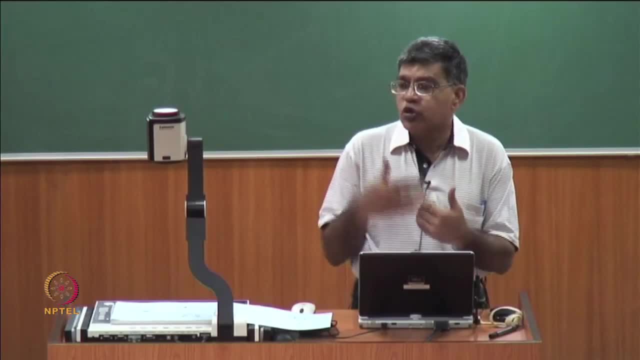 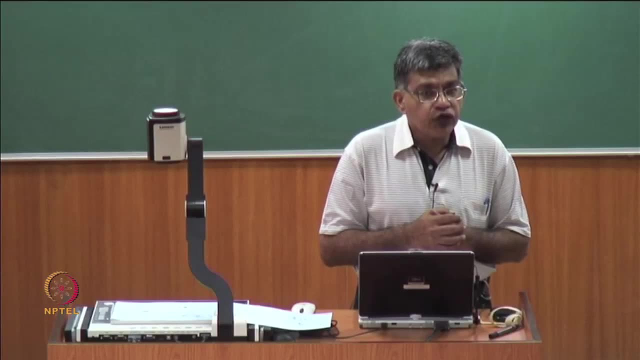 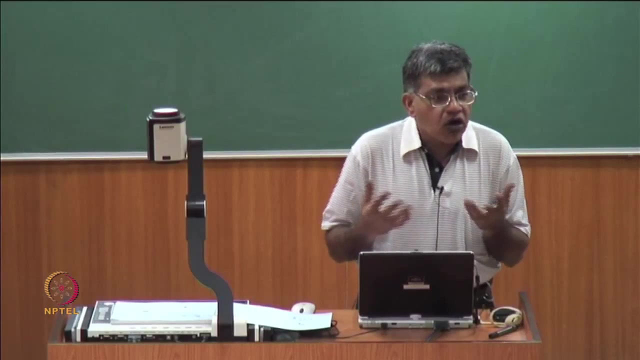 there is one thing is clear: the deduction theorem holds for propositions. So one thing is clear: that if you are you take any general theory, all your set or all your formulae are likely to be closed formulae because you are trying to prove general. 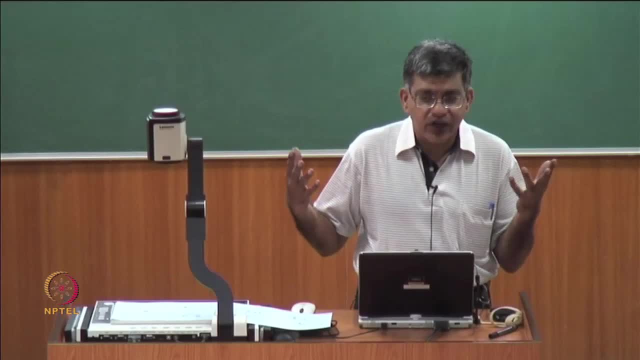 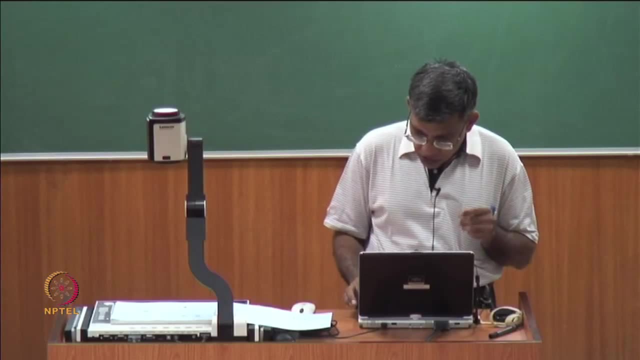 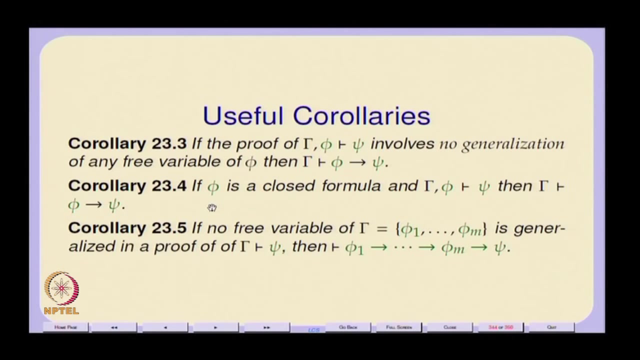 theorems. When you prove general theorems there are no free variables, So the deduction theorem in it is propositional form, there becomes directly available. So actually so the corollary of this is a following: if phi is a closed formula and 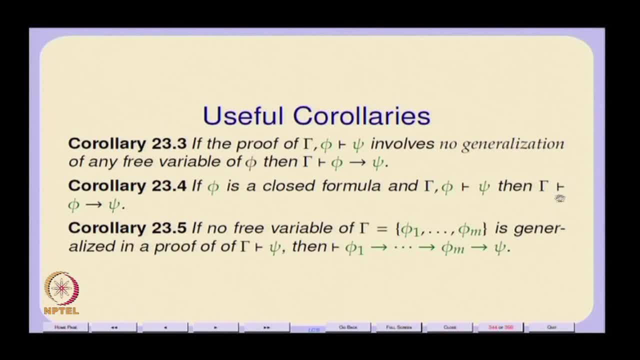 from gamma phi. you can prove that psi, So you can satisfy it. that is how you get a free psi. then you can assume that you can prove from gamma phi r of psi. So even if psi is not a closed formula, it does not matter. But most importantly, if you are proving very 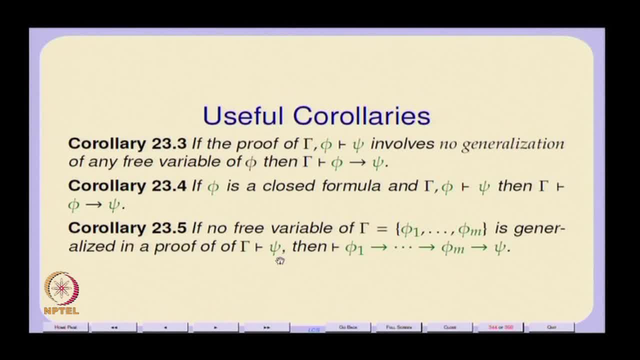 general theorems. if all the formulae that you are taking as assumptions are closed formulae, like the group theoretic axioms, and you are trying to prove general properties of groups, If all of them are closed formulae, then their deduction theorem is any way applicable without any problem. It is only when your 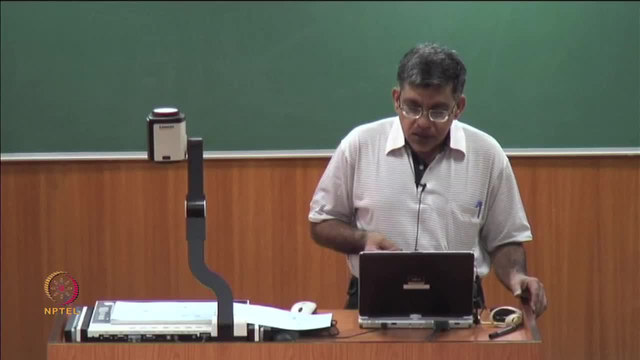 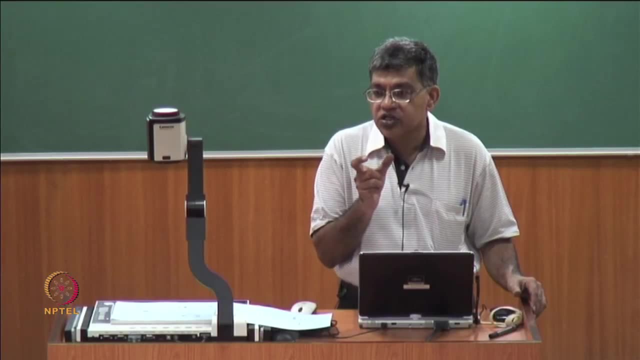 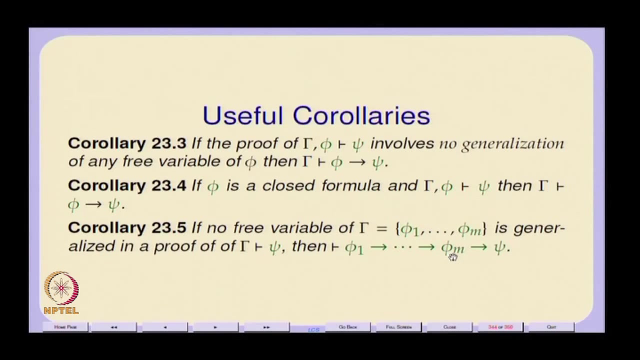 formulae actually use some free variables that you have to be careful about whether you are following the conditions of the deduction theorem before you use it. So, essentially, in order to prove if phi 1 to phi m are all closed formulae. 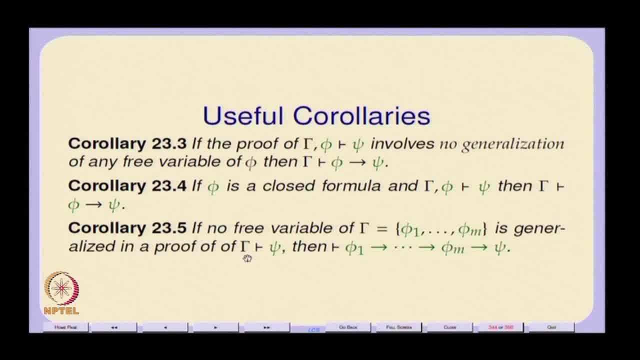 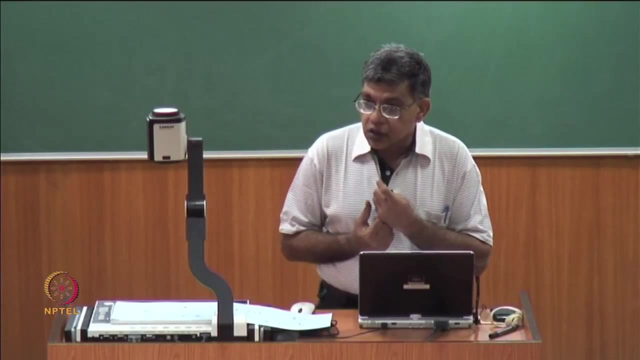 So I can either decide to prove this or I can decide to prove, take all of them as assumptions and prove psi from these assumptions, and both of them are equivalent. So the other thing is supposing your proof actually is a proof of some very specific object which 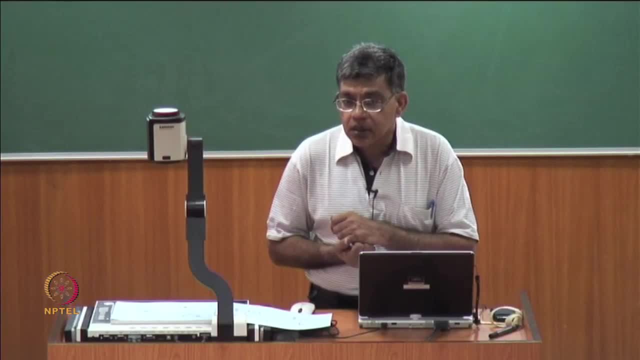 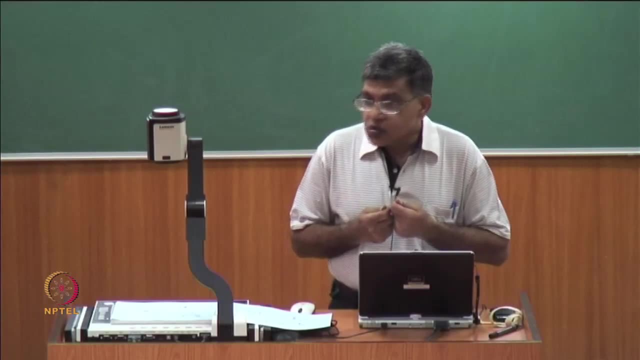 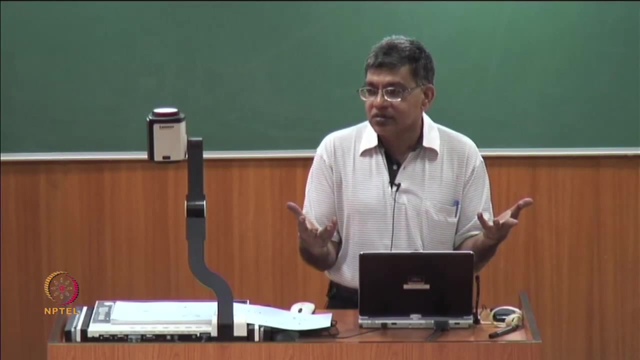 has been, which is called x. let us say, And your proof is all about that, then any way you would not generalize on it. So you take any proof which does not have any involve any generalization. There again the deduction theorem is applicable. So that is the 1st corollary. 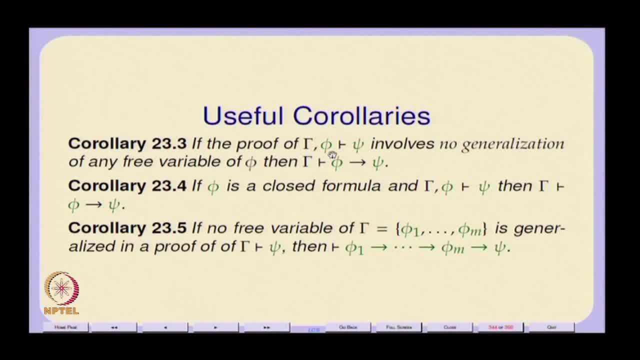 So if the proof of psi from gamma comma phi involves no generalization, any free variable, then from gamma you can claim that phi arrow psi is true. So if phi is a closed formula, then you can claim that from gamma and phi if you prove. 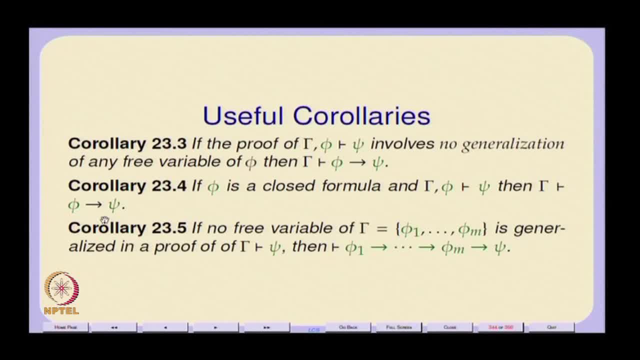 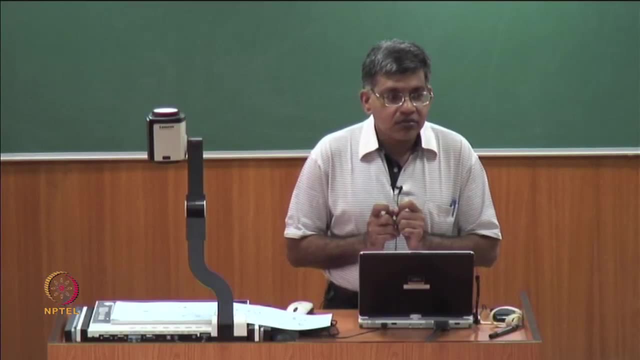 psi, you can prove that gamma proves phi. i root psi, And if there are no free variables anyway, then you can apply the deduction theorem. The only case where you have to worry about whether the deduction theorem is at all applicable is a case when a generalization has taken place in the proof. 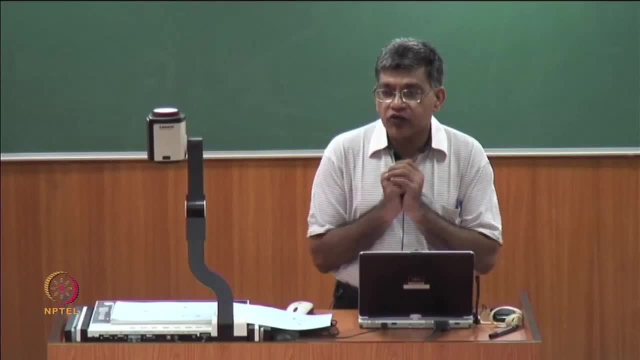 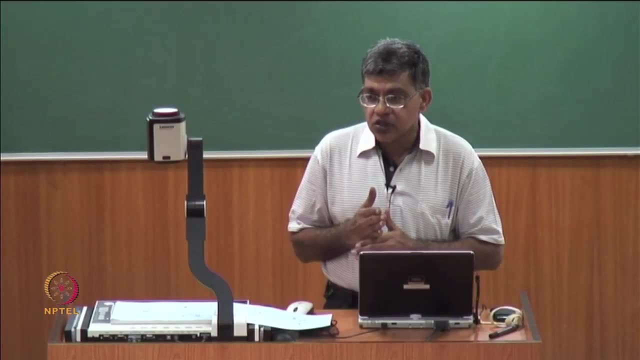 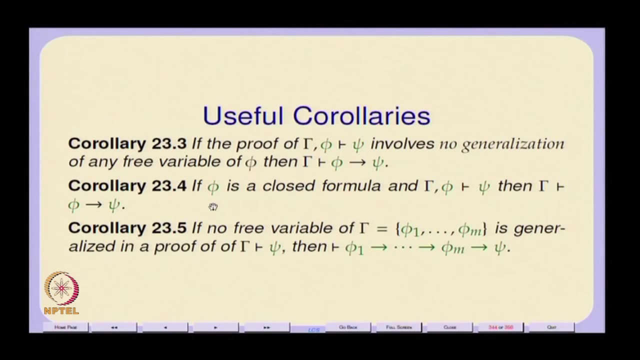 So it requires going through the proof tree to find out whether there is any occurrence of universal generalization. And if you are doing an occurrence of universal generalization you have to check basically whether the free variables in this assumption phi, have been generalized or not. 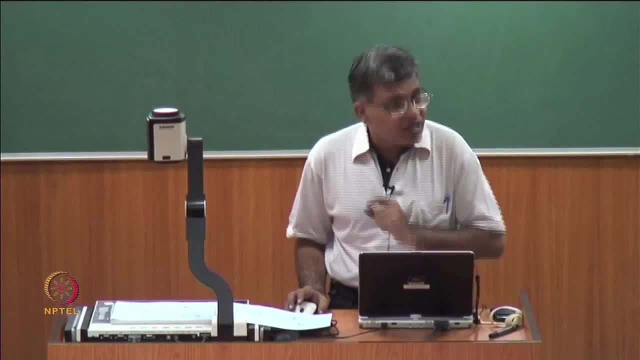 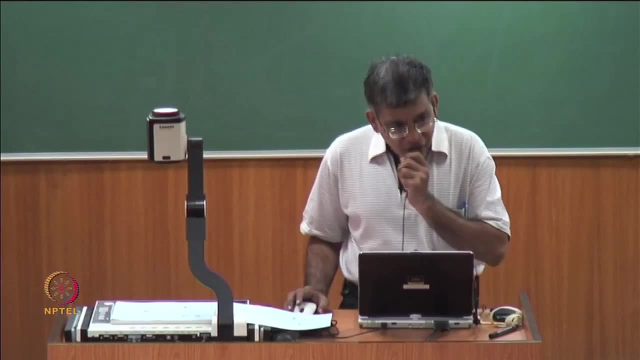 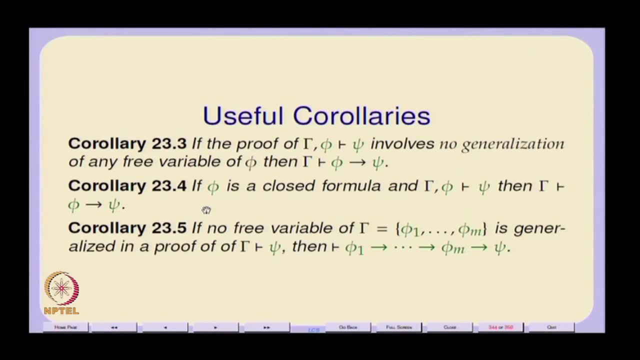 If none of the free variables in phi has been generalized, then again you are safe. You can just apply the deduction theorem If a free variable of phi has been generalized or you are using some. if a free variable of phi has been generalized, then you cannot push it. 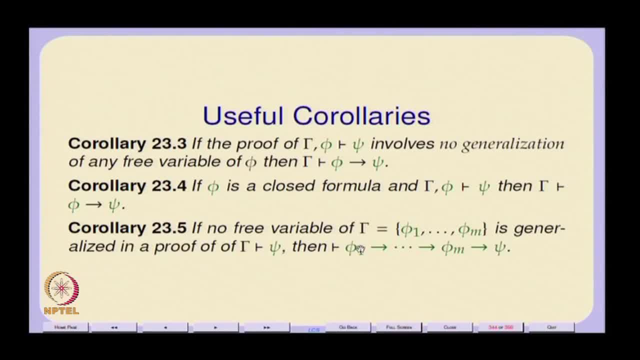 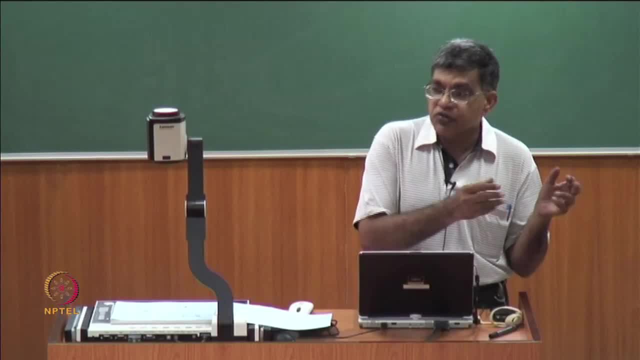 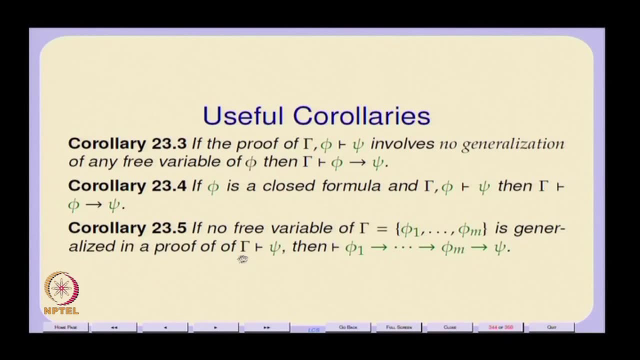 But remember that normally what you want to do is you want to factor out everything which appears on the left side of arrows as an assumption, So which means you are looking at all free variables of phi 1 to phi m. In order to have these two equivalent, it requires that any proof which involves proving 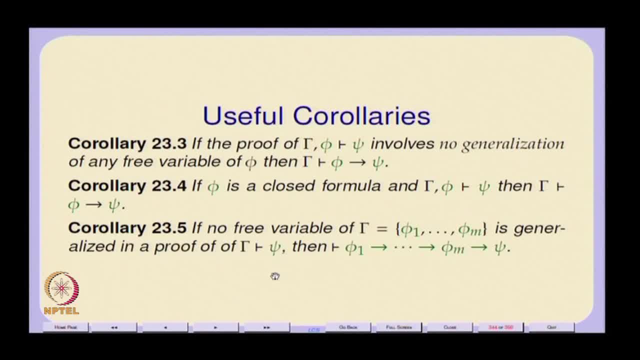 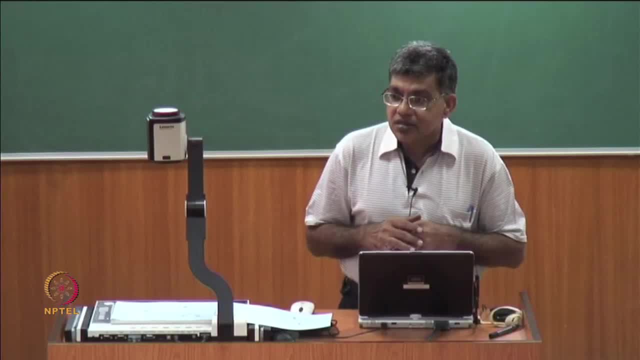 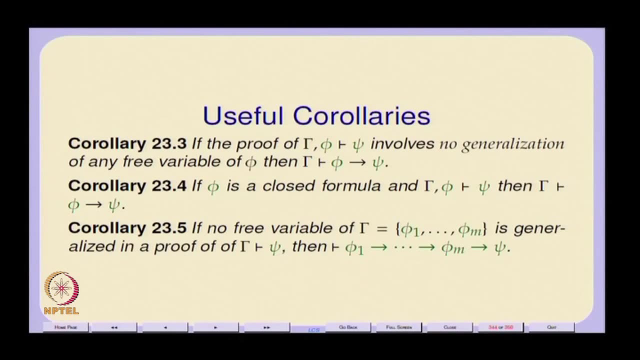 psi from gamma does not generalize any of the free variables in phi 1 to phi m. But if it generalizes something else may be, generalizes a free variable in psi which is not present in phi 1 to phi m, then you are still safe. 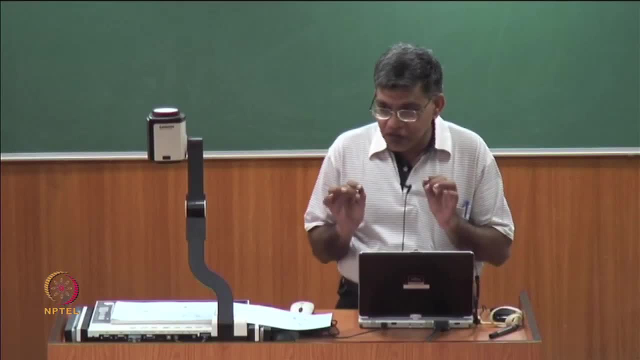 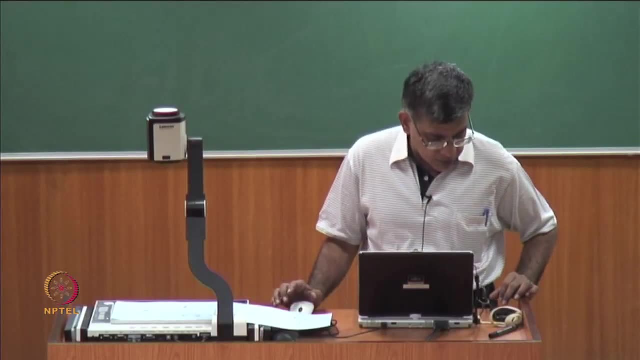 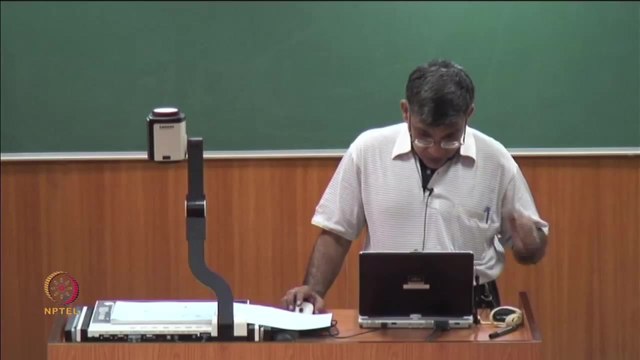 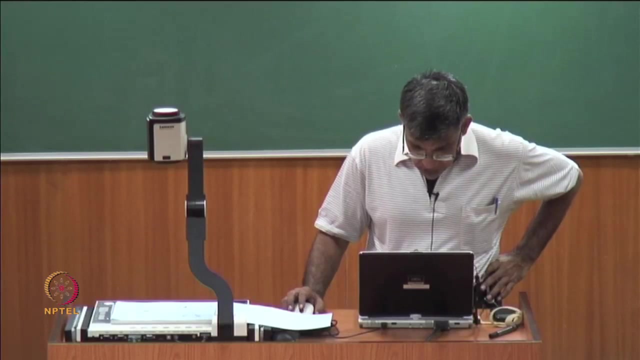 There are various conditions. It becomes very subtle at this point. So under what conditions can you actually check whether the deduction theorem is applicable Now? actually it is. the question is whether I should go into soundness now or postpone that. 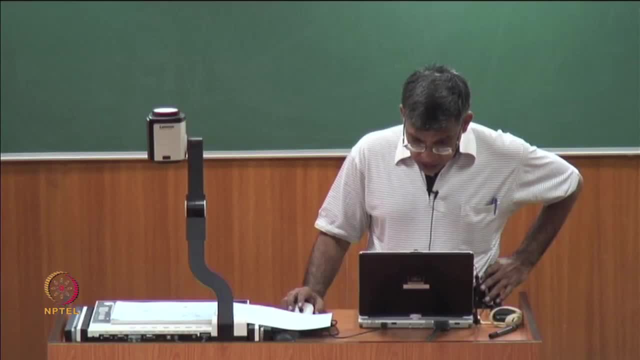 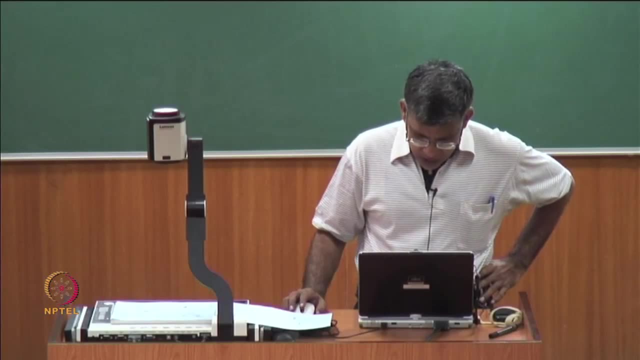 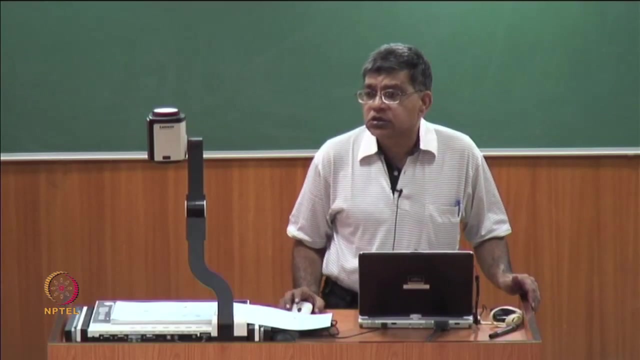 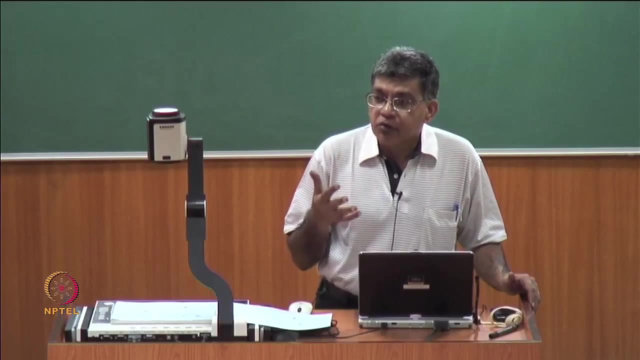 Cn't, Because I am going to do it as before. So another. then there is, of course, is question of existential quantification also. So which? but then let us just do the soundness. So, first proposition, you are. I have not actually spoken about existential quantifier, but the. 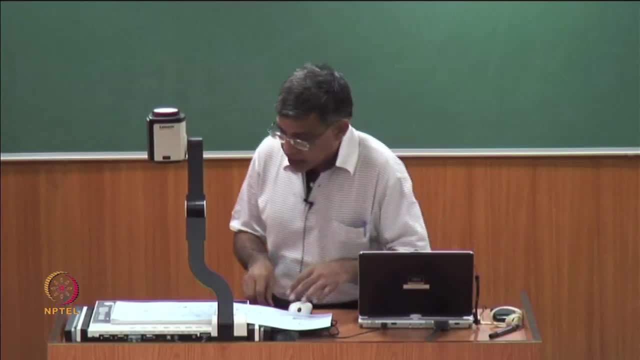 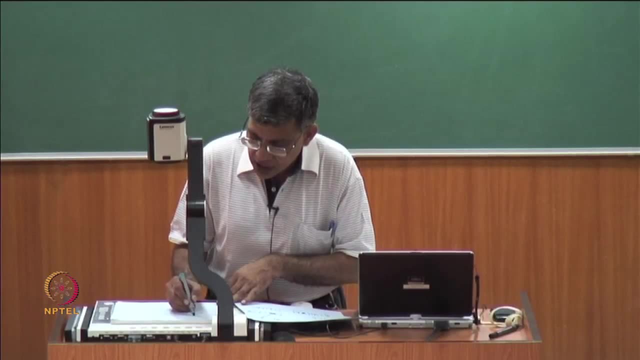 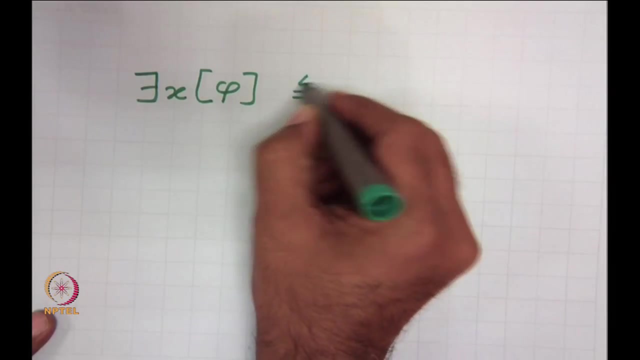 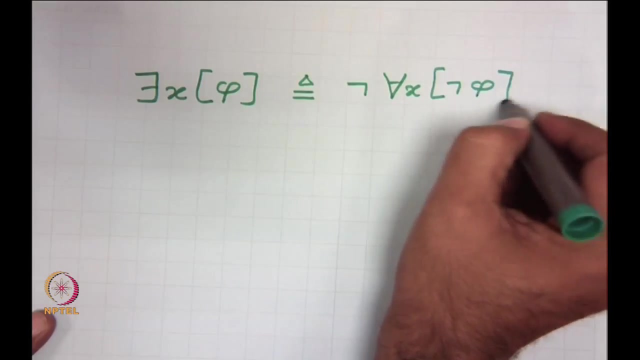 point is that you are existential. quantifier is going to be defined by De Morgan rule. You are essentially in a Hilbert style proof system. you are essentially stating that this formula is going to be defined as not of for all, x, not phi. So you 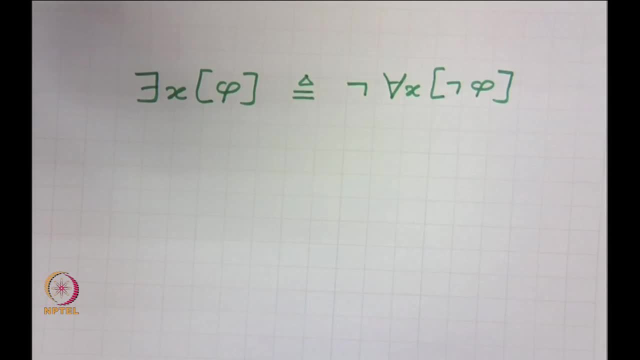 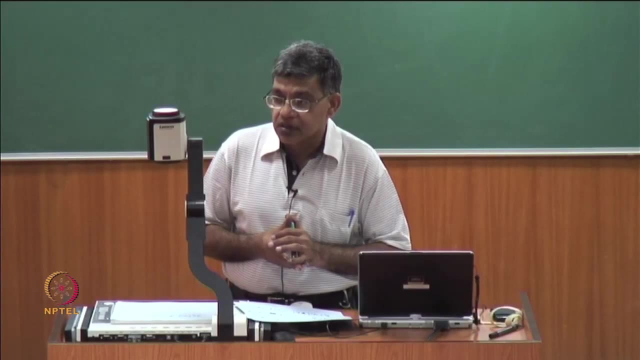 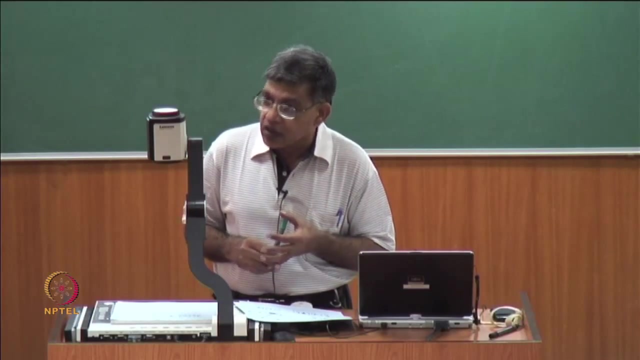 are going to use this definition. So the notion of arbitrary and particular then take a certain meaning here, usually with the existential quantifiers, And we have to be able to justify some of the proof methods that we use for existential quantifiers from the Hilbert style system itself. But that is it is a little complicated So I will postpone. 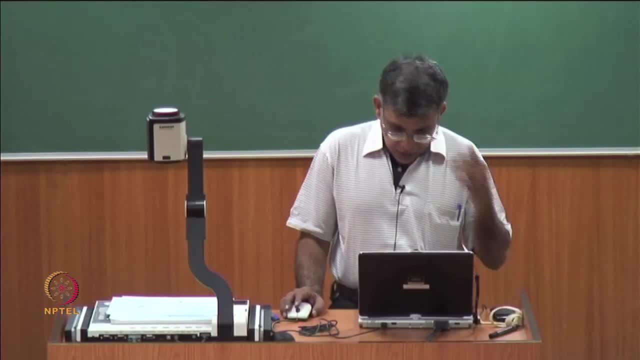 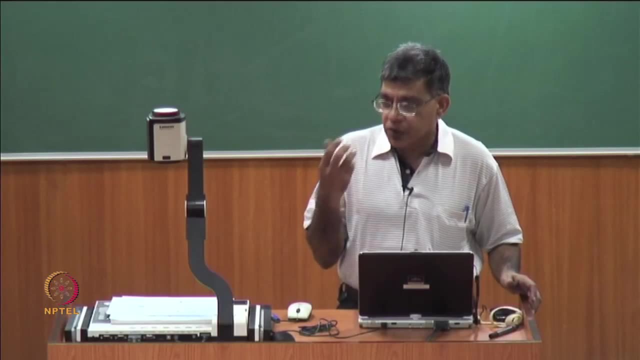 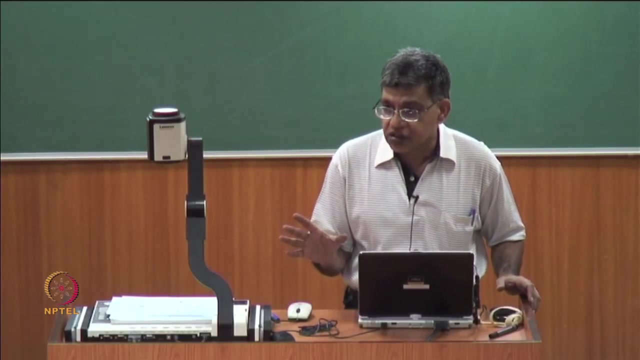 that. in the mean time, let us just look at this soundness. firstly, of course, that you take any well formed formula which is an instance of a propositional tautology. No valuation can change it, no model can change, it is always going to be true. So tautologousness. 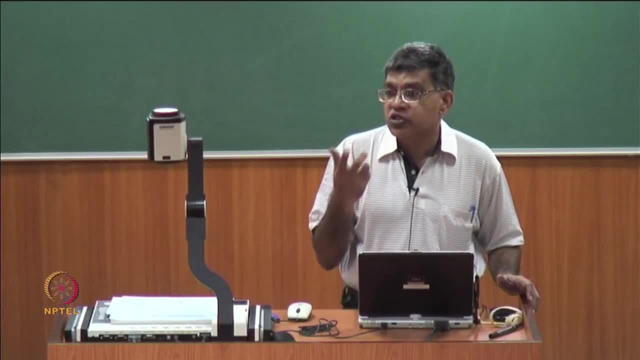 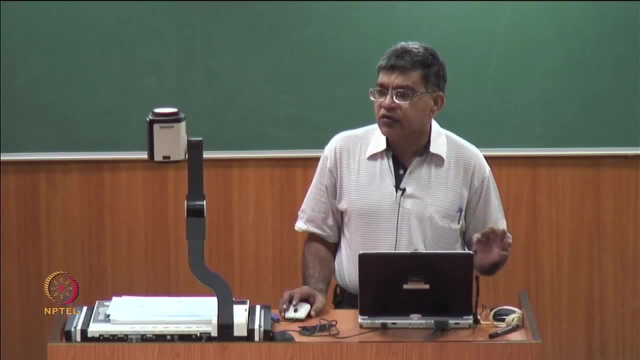 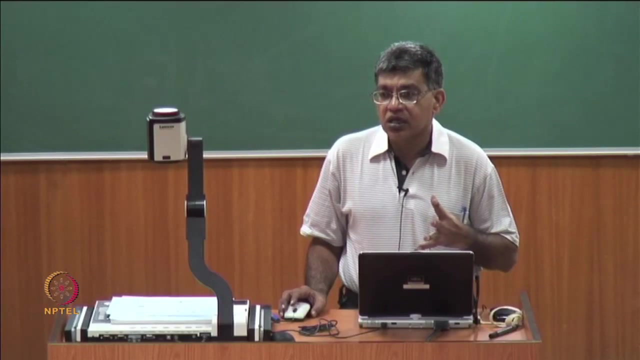 is preserved by the propositional tautologous forms, So you can essentially take so this proposition. I am not even going to prove essentially what we are saying is. So that is equivalent to saying that you take any predicate formula which can be derived by just using k, s, n and. 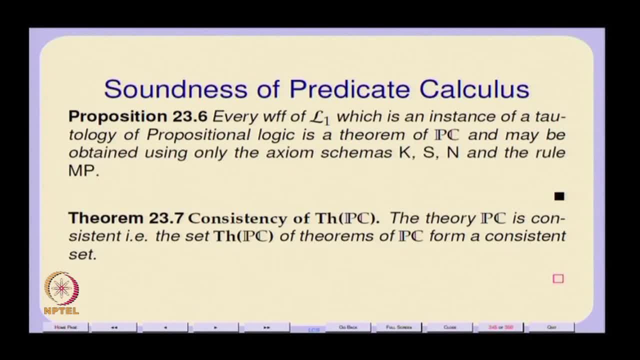 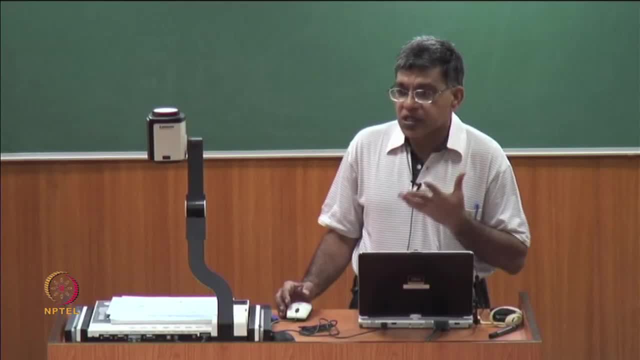 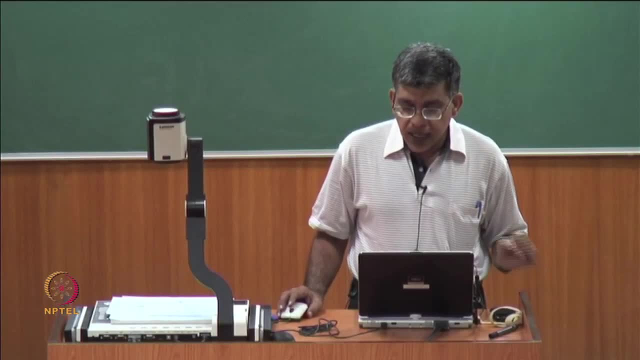 m p. So it is always going to be valid. So all propositional tautologous forms with corresponding propositions, replaced by predicates, do not change their truth value ever and their validity can be proven. So in that sense k, s, n and m p are sound rules for predicate logic. 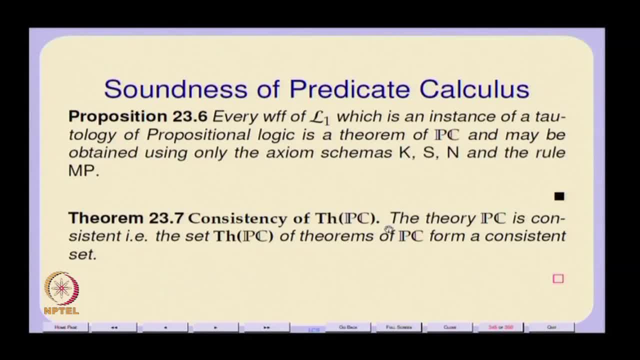 So the other interesting thing is that you take- so I am going to use t h of n, tautological So k s n is thehorse which is used in a heard sounding logic and you need to keep. 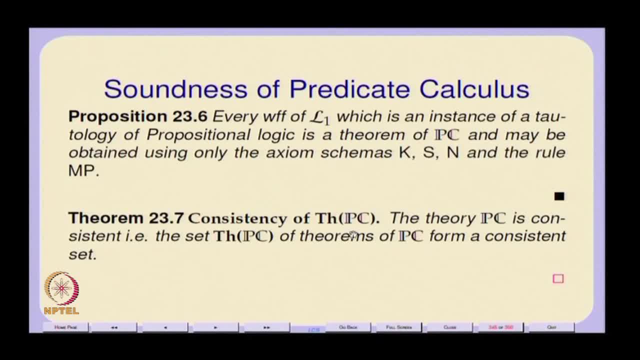 show us that the rules of logic are there. Yes, the other interesting thing is that you take, so I am going to use t, h of n, So I am looking at predicate calculus itself as a theory. you know, with these axioms, k, s, 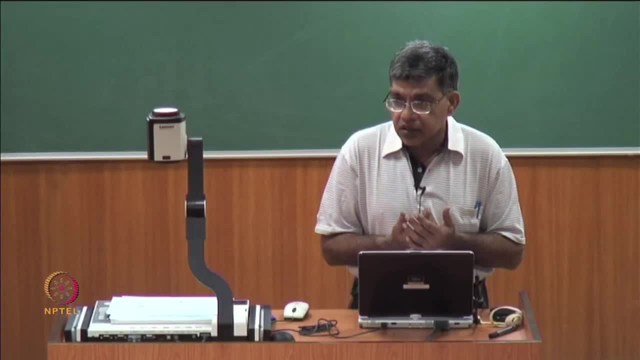 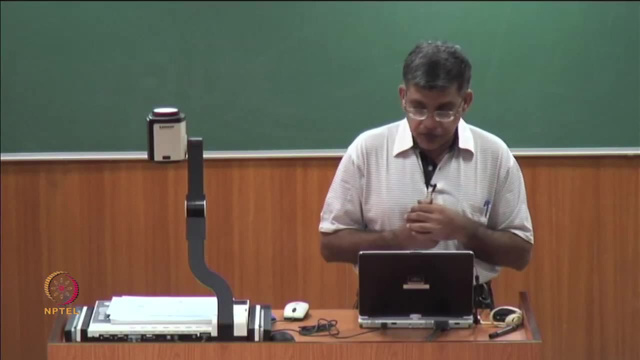 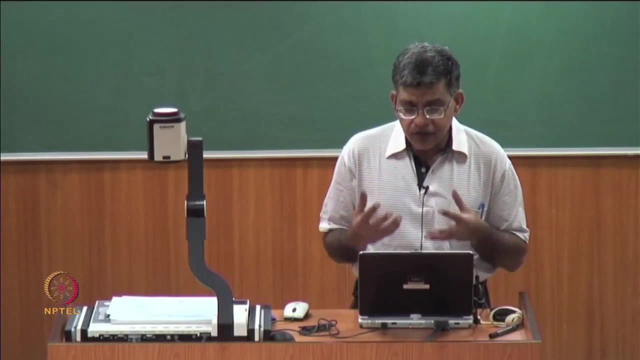 n, m, p, for all i, for all e, for all d, And the t h of P, c stands for all the theorems of this theory. So a formal theory. so take the set of all theorems of this theory. So whatever is, 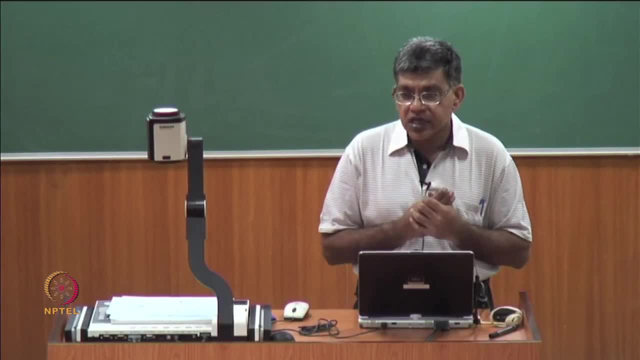 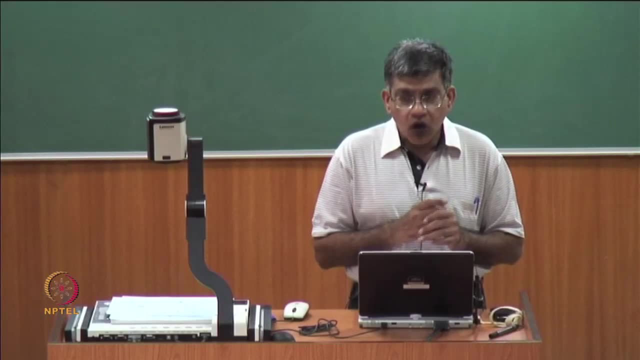 provable by the Hilbert in predicate calculus, by the Hilbert style proof system. So this theory, first of all, is consistent. that means all the theorems that you prove are have truth, values, They have models and valuations, have interpretations in which they can be. 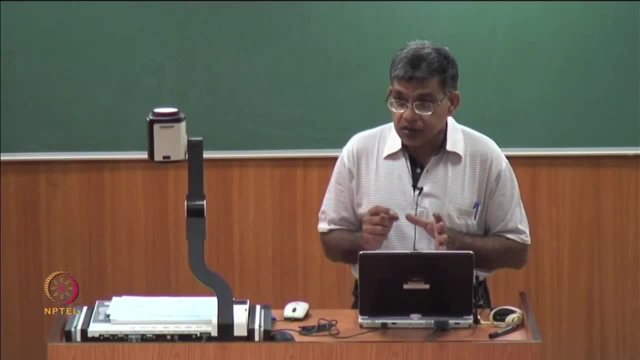 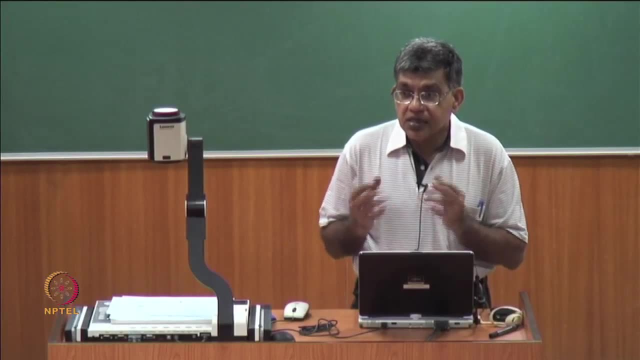 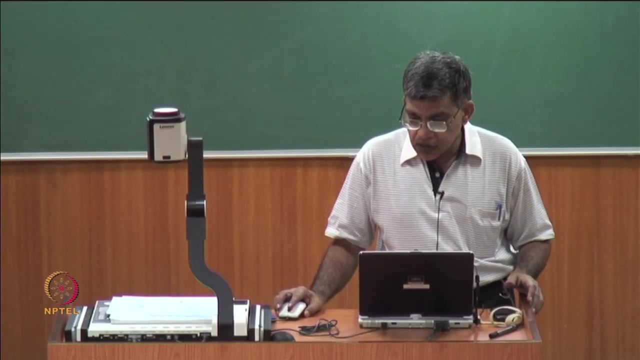 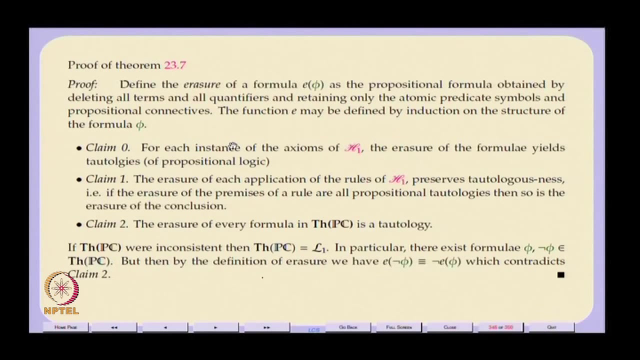 made true. It is important because the consistency of the set of formulae is required to show that your proof system itself is sound. So this, the consistency of this is just depends upon this claims. So I take any of the theorems, any of the formulae in the theory of predicate calculus. 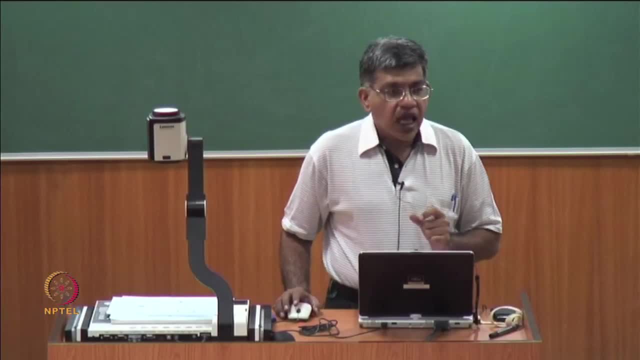 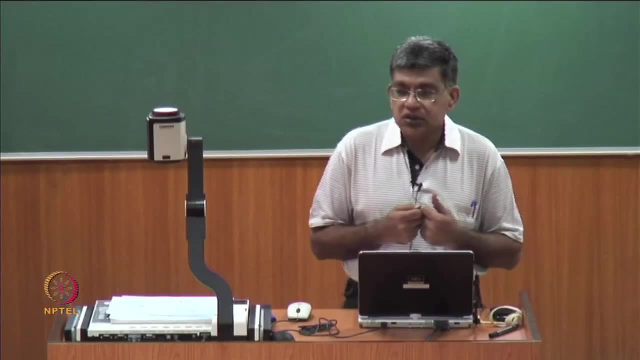 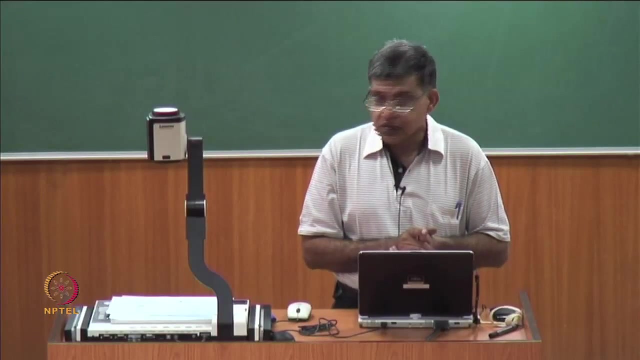 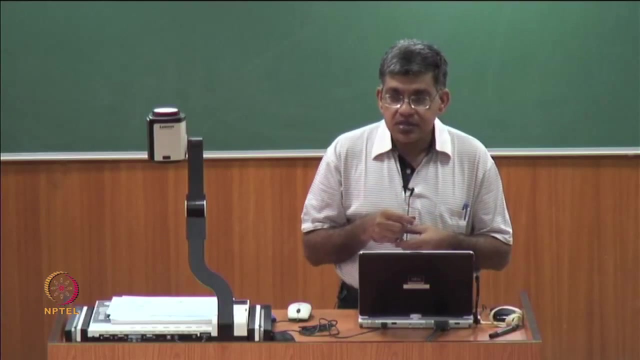 calculus, some formula phi, and I define what is known as its erasure. The erasure of a formula is just that I remove everything that is violet in color from it. I remove all the terms, I retain only the atomic predicate symbols and I remove all the quantifiers. 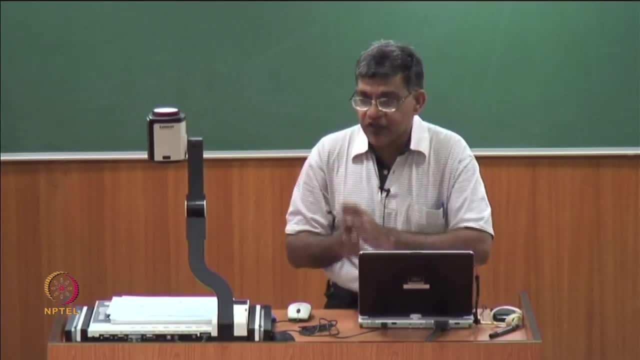 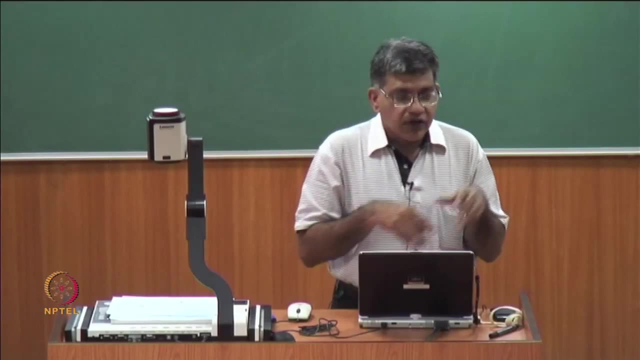 If I remove all the quantifiers, I have also removed all the variables. if I have removed all the terms, I have removed all the variables, So the quantifiers are anyway of no use. I have removed all the quantifiers. When I remove all the terms and all the quantifiers, what am I left with? I am left with something. 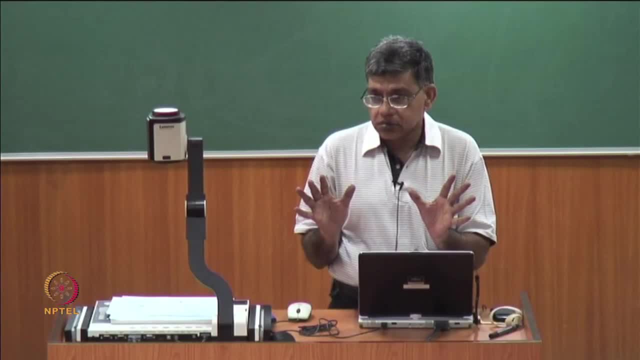 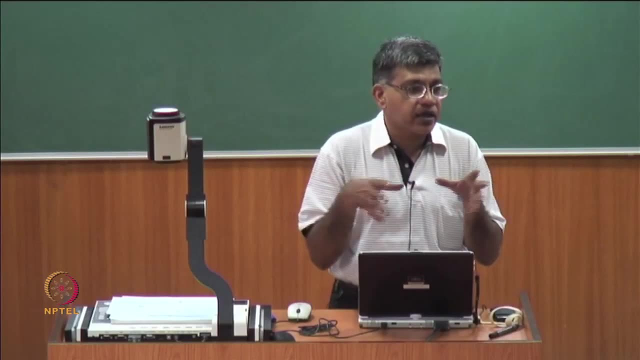 that looks purely propositional. It just looks like a proposition with propositional atoms and propositional connectives like not and arrow and so on and so forth. that is all. So it looks like a propositional atom, It looks like a purely propositional formula. 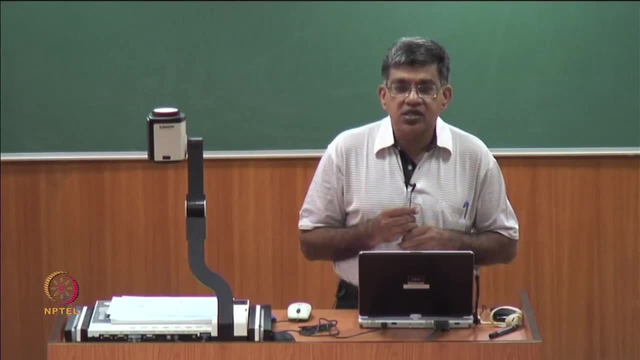 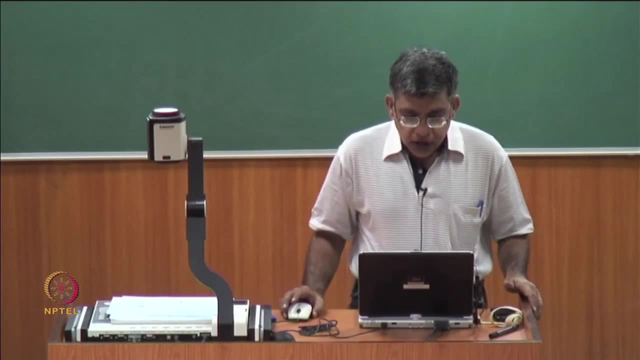 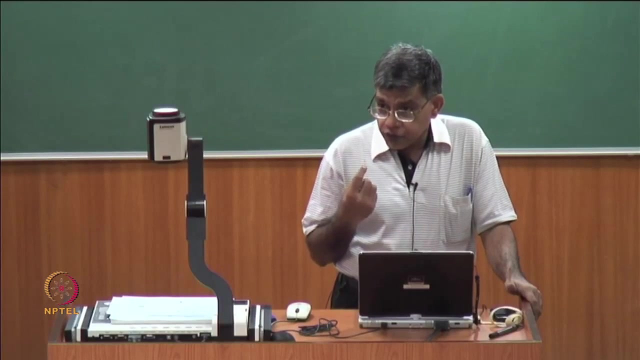 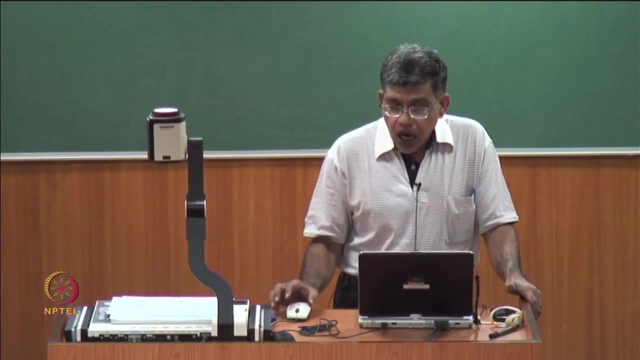 So the erasure of a formula E phi is just a purely propositional form with propositional connectives, no quantifiers, no terms, nothing. Now you take any of the theorems of first order logic. So you take anything that is provable in the Hilbert style system: H 1.. 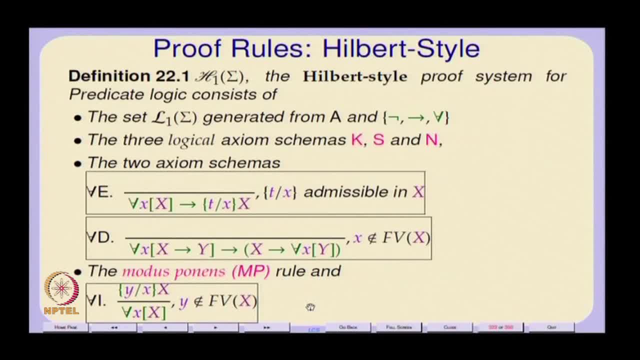 The erasure and take the erasure of any of the formulae that you get as theorems. The erasure is always a tautological form for all the axioms. So for k, s and N is easy to show that there there are tautological forms. 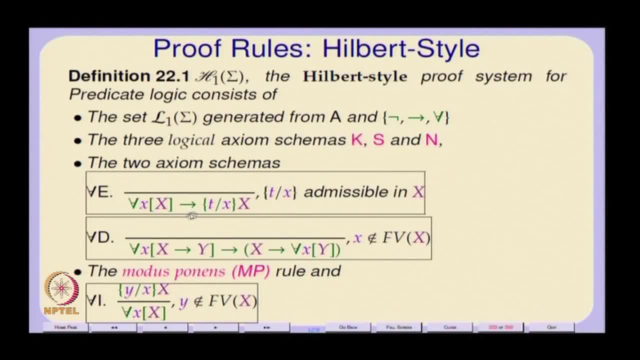 The only thing, therefore, it is show for these two, But for these, you can see, I mean if I erase, if x is a purely propositional atom, and I am going to erase this for all x, and I am going to erase all this t for x. 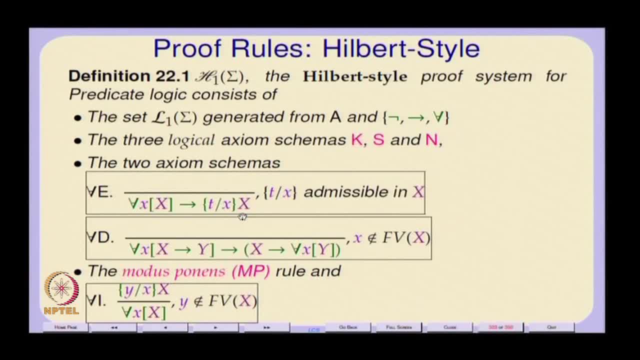 I am erasing all the terms there, all the violet terms there. So then, what am I left with? I am just left with x arrow, x, which is a total logus form. Similarly, in the case of Feroldi, when I do the erasure, 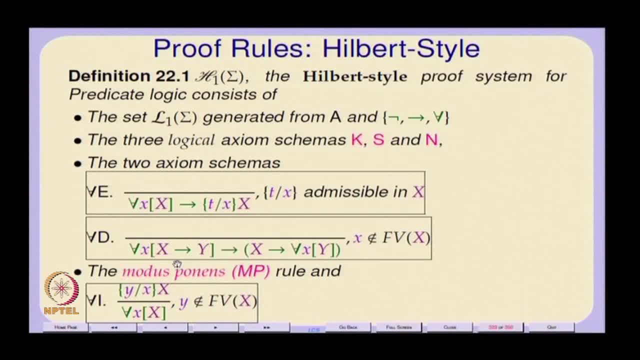 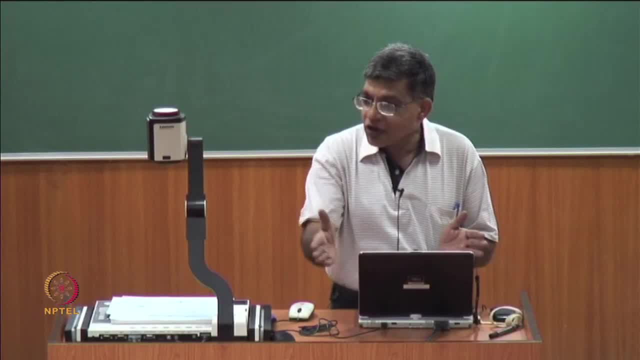 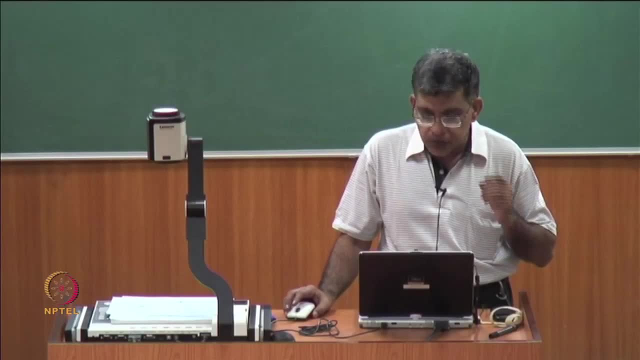 I am just left with x arrow, y arrow, x arrow y, which is also a total logus form. So the erasure ensures that you will have only total logus forms, And in fact so the modus ponens rule of course preserves total logus form. So that is not the problem. the problem is: 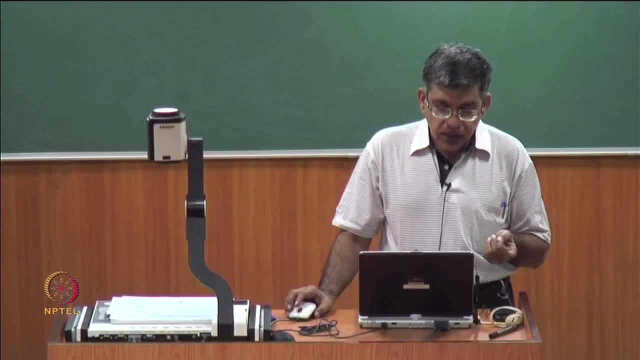 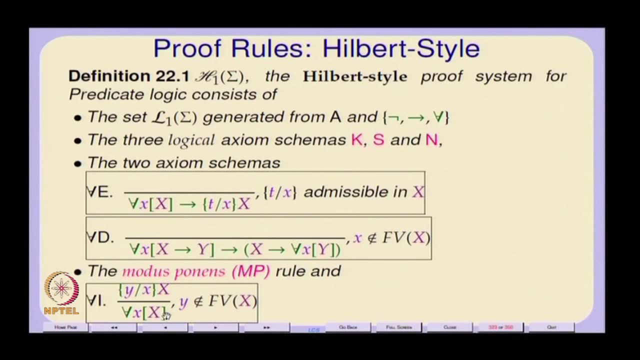 with universal generalization. Here again, when I do the erasure, what do I get from x? I get x, which preserves tautologies. If x is a tautology, then x would also be a tautology, So all. so the erasure is such that all the axioms 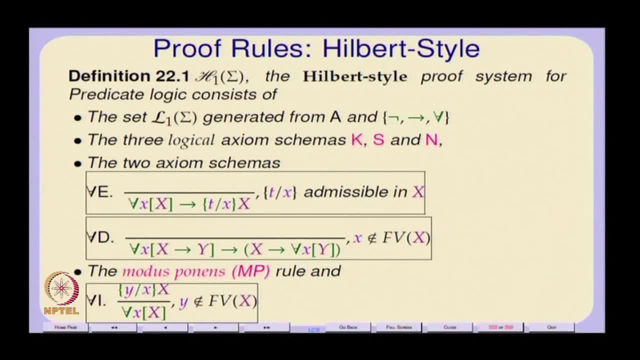 and inference rules Of H 1 of the system H 1, the axioms only create total logus forms. the rules of inference preserve total logus forms, So if they had a hypothesis which are total logus, then the rules would ensure that the conclusions are also total logus. The erasure is of the conclusion. 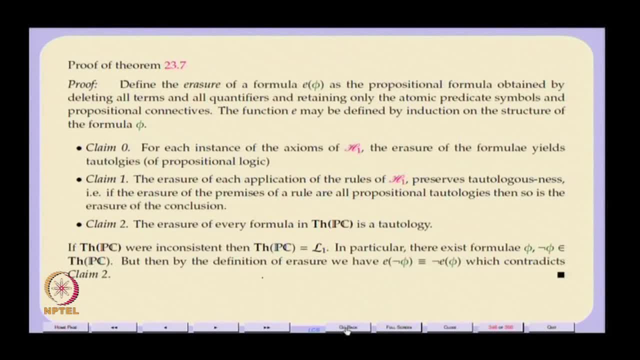 is also total logus. So claim 0 essentially says that the erasure of all the axioms gives you total logus forms. Claim 1says that the erasure in every rule preserves total logus forms. So if the hypothesis was a total logus form, then the conclusion was also total logus. 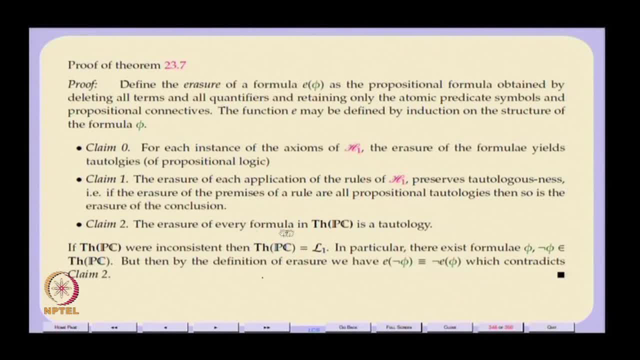 form. And then claim 2 say the erasure of every formula in PC is a total logus, because every proof just preserves total logus forms. So now so the? so you take the erasure of the theorems of PC, you will get only tautologies. 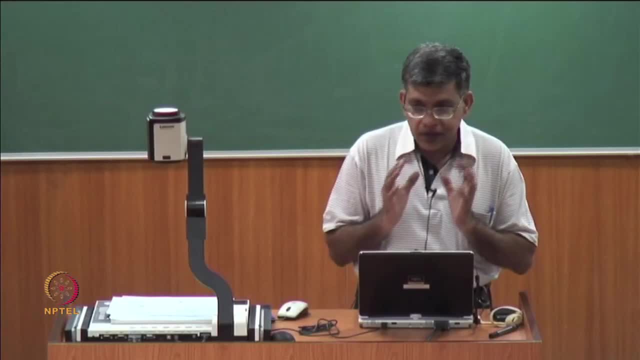 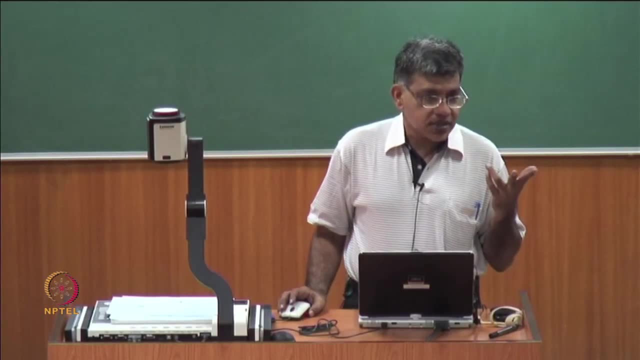 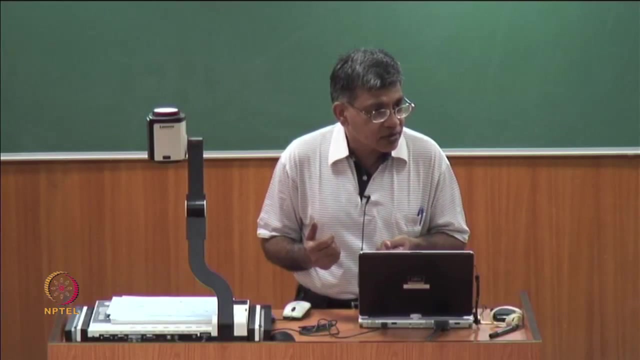 So all the sentences in theory of PC you apply, erasure on all of them. you will get only tautologies. Now we know that that has to be consistent, but now, but that does not mean that theory of PC itself will be consistent, right. 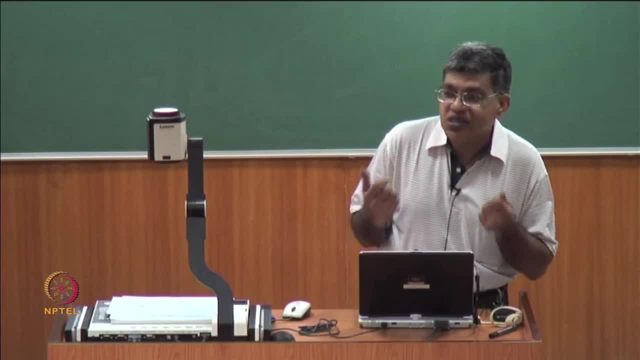 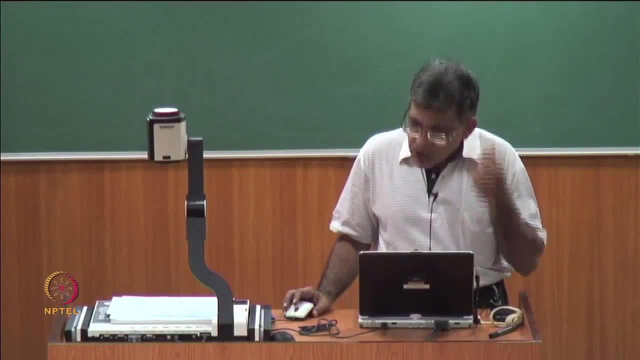 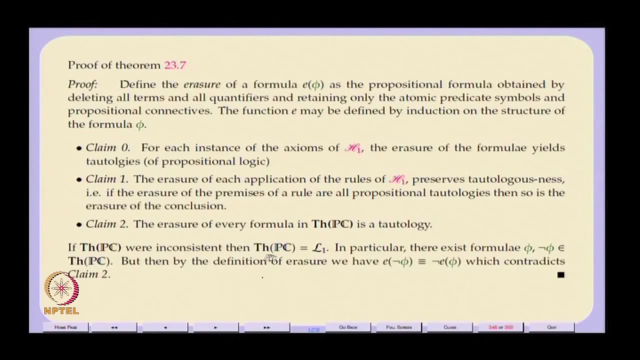 It is only the erasure, since it produces only tautologous forms, it will be consistent. So now we argue by contradiction. suppose theory of PC contains, supposing it were inconsistent, then firstly, the theory of PC would be the whole language, L 1.. 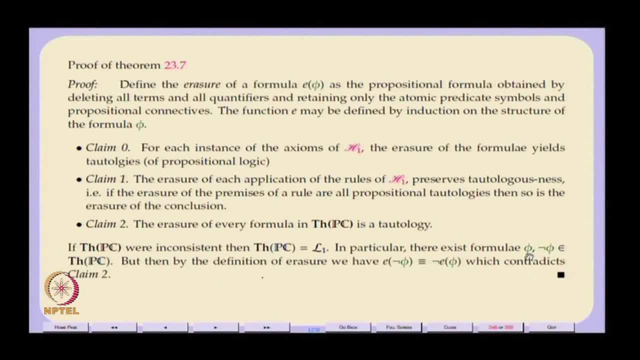 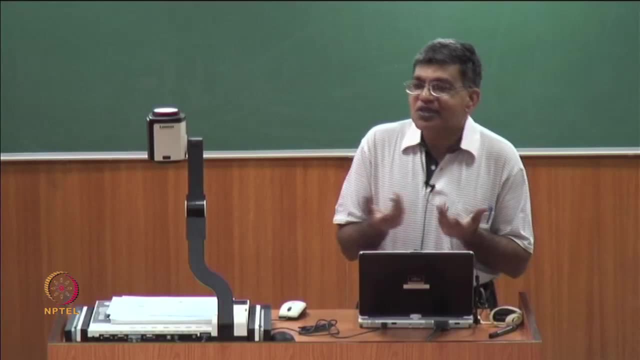 And in particular, there will exist two formulas, Phi and naught, phi belonging to the theory of PC. But if phi and naught phi both belong to the theory of PC, then the erasure should be both the tautologies, but naught does not get erased.